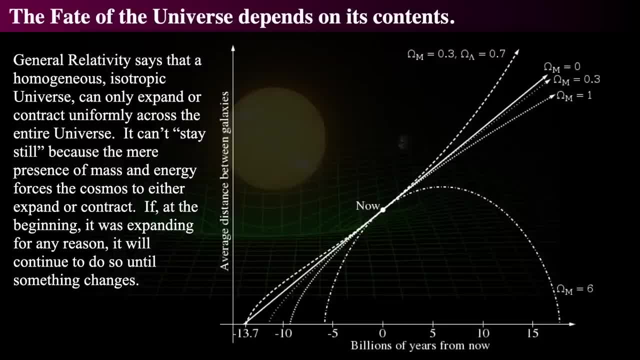 be homogeneous and isotropic, and it will if it's. if it is homogeneous and isotropic, there's only two possibilities. Actually, there's a third: It can expand or contract uniformly across the entire universe, And that's the nature of the assumption underneath the Friedman-Robertson-Walker. 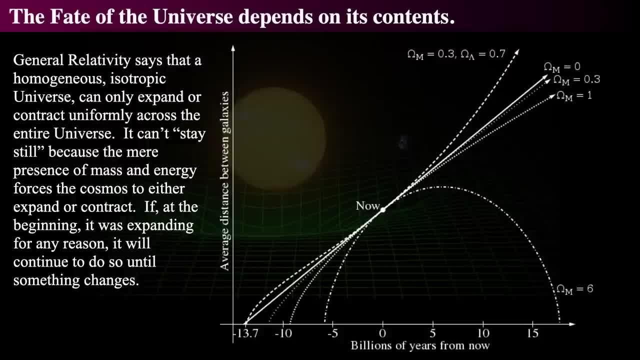 metric which posits an isotropic, homogenous universe on the largest size scales. Now, of course, we don't know how the universe will expand. We don't know how the universe will expand. Of course, the flow of the expansion is halted because inside of, like the Earth. 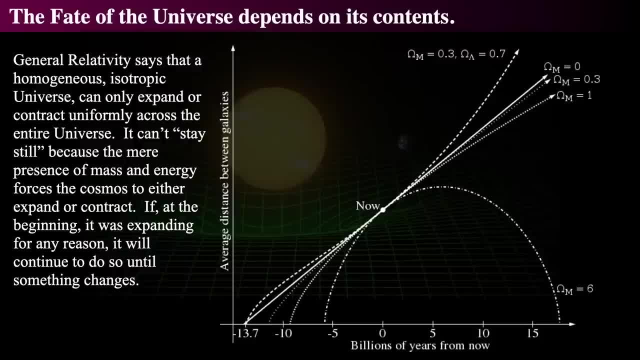 because the Earth is gravitationally bound, so it also is the Milky Way, so is the local group, so is the local supercluster. But when you get size scales much larger than the Hanayakia supercluster, then you are experiencing the expansion of the cosmos, And that's uniform. 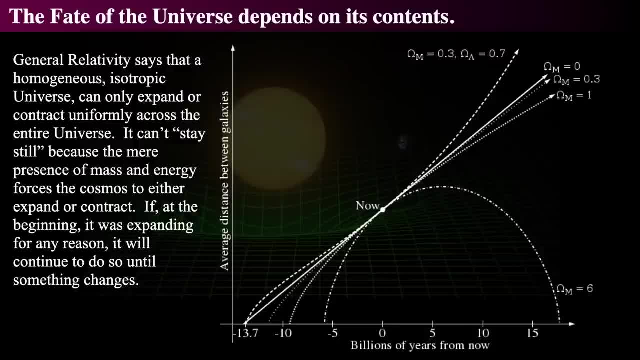 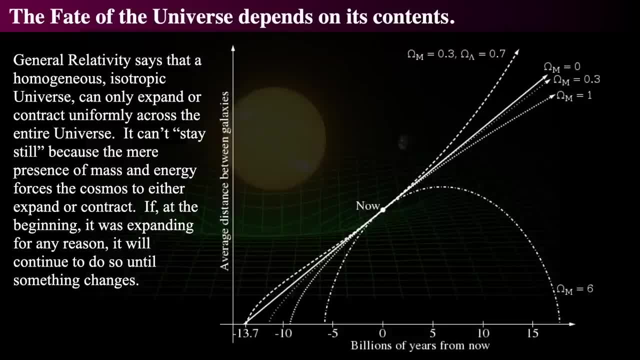 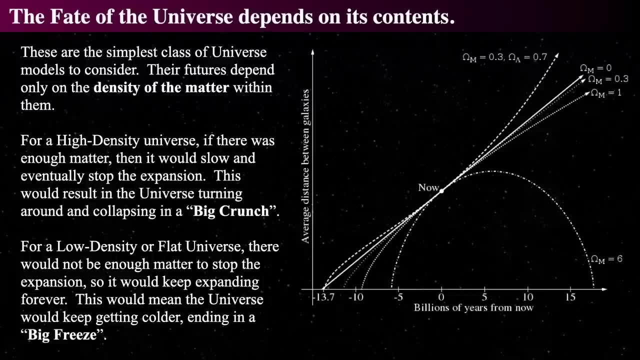 It's still forever, but that's an unstable situation. So if there was a tiny, tiny, tiny change, then the stand still would either expand or contract. So the contents of the universe dictate what's going to happen And of the simplest possible models of the 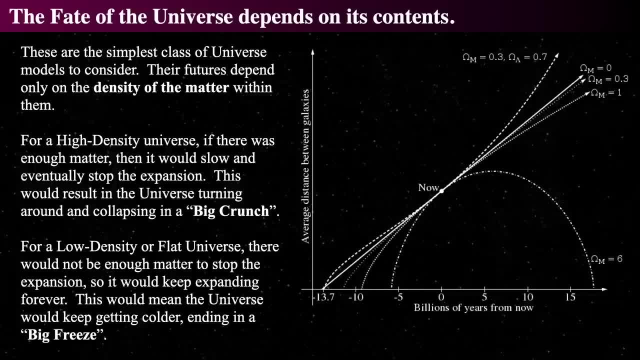 universe in which I grew up with and dealt with when I was in college and grad school was that the universe was only considered to have matter in it. matter and light: Those are the only things that people thought they were And, in fact, people understood that. 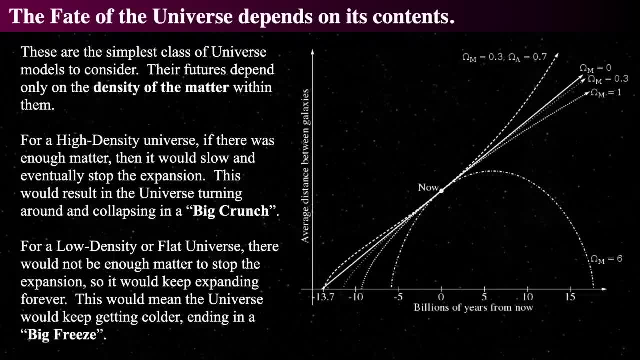 the energy density due to light and radiation, or, more specifically, ultra-relativistic things like neutrinos and so forth, contributed not as much energy density to the cosmos as regular matter and cold dark matter. So if cold dark matter and normal matter were the only, 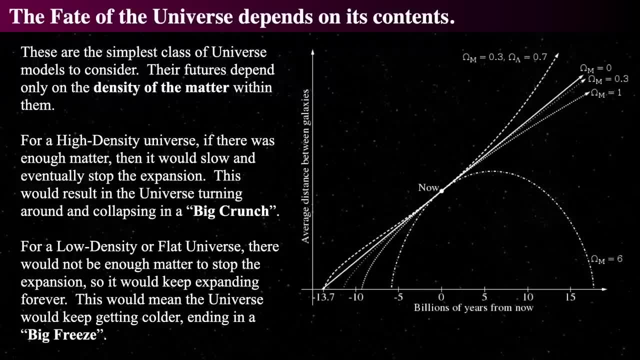 thing. then the destiny of the universe would depend 100% on the density of the matter. And for a high-density universe, for a very, very high-density universe, greater than the critical density, then it would collapse back down eventually to a big crunch, meaning the expansion would 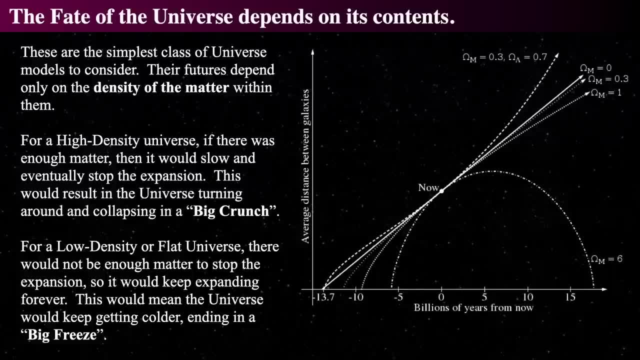 slow down and then reverse. if the density of the universe were greater than the critical density and it were completely made of normal or dark matter, If it were lower density than critical or flat, then the universe and composed only of dark matter and normal matter. then 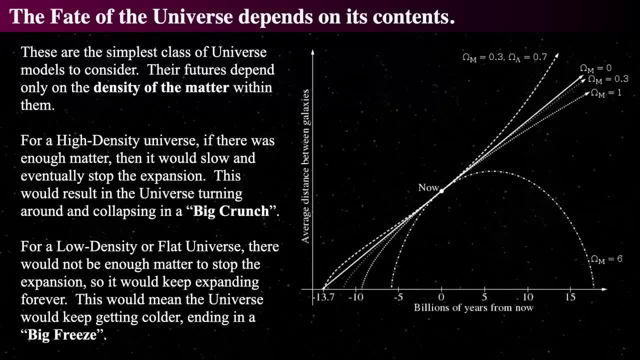 the universe would eventually get larger and larger and larger and expand and expand and expand and in fact expand forever, And its rate of expansion would gently increase. but it would certainly expand forever And that's called an open universe And that would mean a big freeze. 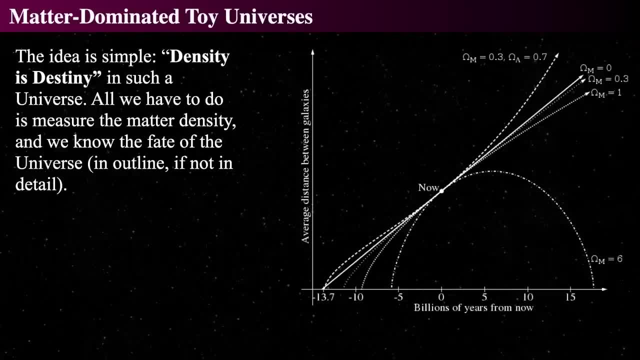 So pretty much the idea was when I was in grad school in the 90s was the idea was people were trying to measure the matter density of the universe and therefore how fast the universe was decelerating, And that was the. The big idea is that the matter was what was in the universe, So the density is the. 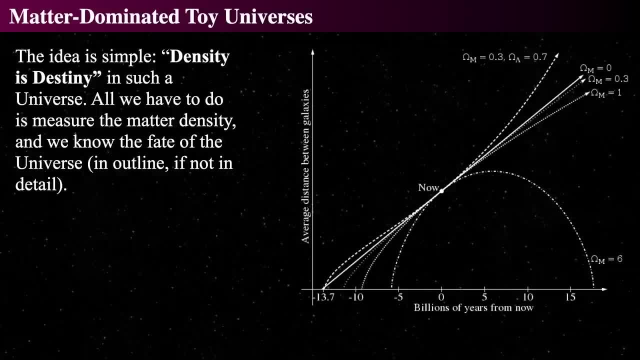 destiny. So people wanted to know how long in the future it was before a big crunch, or how long it was in the future before a big freeze. That was the ultimate concept of the 1990s And that was one of the reasons why the Hubble Space Telescope was launched and determined. 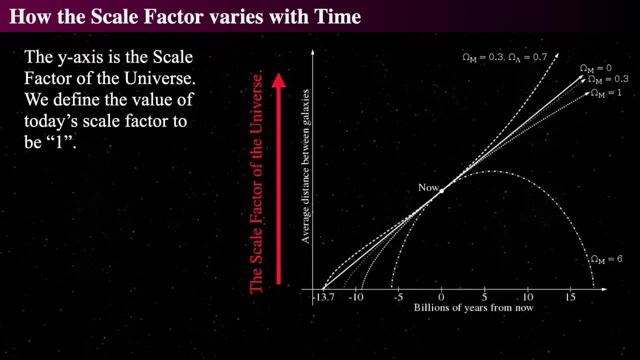 the. This is what we're going to talk about today. So this particular graph shows the scale factor. Now, remember, the scale factor shows the rate of. It shows the expansion of the universe now as opposed to then, or later compared to now. 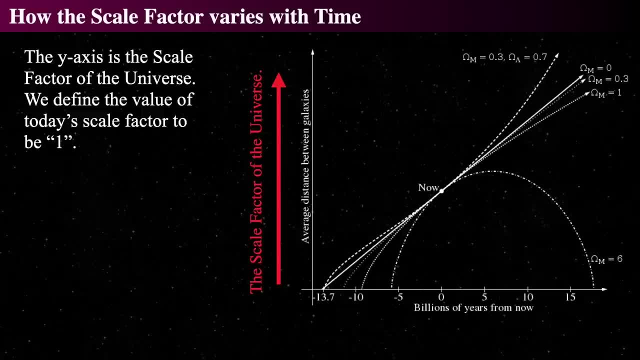 And so the y-axis on this graph could be the scale factor, meaning how much bigger tomorrow it will, How many times bigger it'll be tomorrow than it is today, And that's what we define to be the scale factor Today. at now, we define the scale factor to be one. Remember the scale. 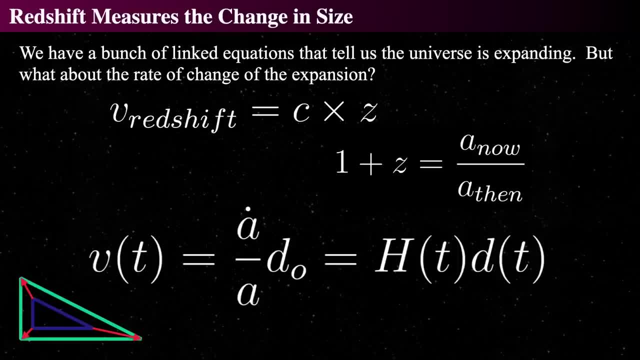 factor, though, was defined by the Redshift. So the redshift itself, remember it went. Hubble went back and looked at the expansion of the universe and discovered it, and discovered that every galaxy had a redshift. So this V of redshift, meaning the speed of the redshift or the recession velocity, that 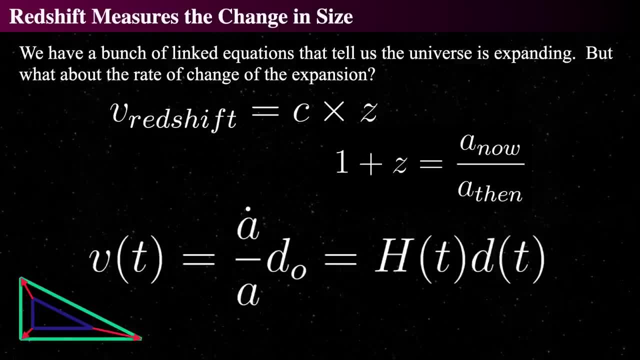 is the V in redshift is equal to the speed of light times. the redshift value that was measured, Remember the redshift value here is defined to be the ratio of the scale factors of now and ago, So that high redshift means smaller scale. 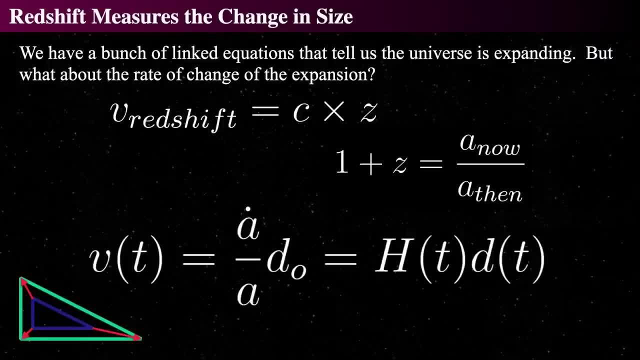 So the speed of the redshift, The scale factor, remember redshift- is directly related to the change in wavelength compared to the original wavelength. That's the definition of redshift. We also then related the redshift to then the scale factor. 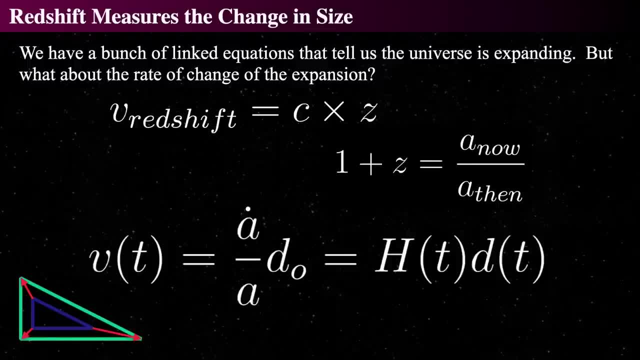 So if we look, we find that, importantly, the expansion velocity then is related to what we call the Hubble cut, the Hubble parameter, which is h of h as a function of time, and d the distance between two objects as a function of time. 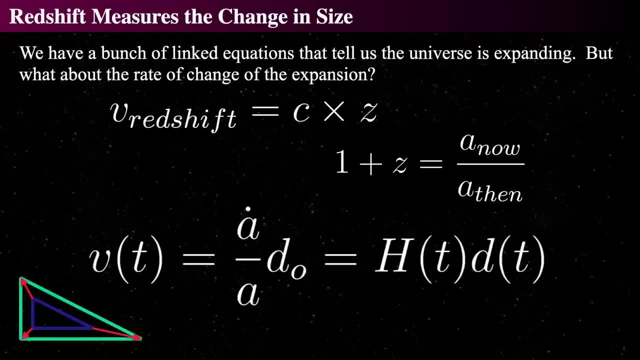 So the velocity, the recession velocity, as a function of time- that's what that parenthesis t means- is equal to the time derivative of a meaning, a dot. And a dot simply says: how does the scale factor vary as a function of time, as the universe? 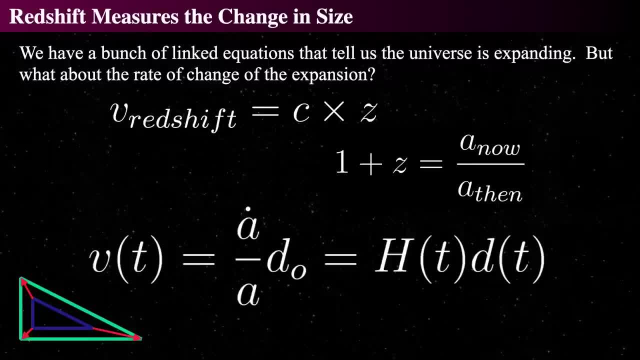 ages, Or how? How was? What was the scale factors? How has it changed with time compared to today? So that's what the a dot over a means. How has the scale factor changed with time compared to the scale factor? How does the scale factor change with time compared to today? 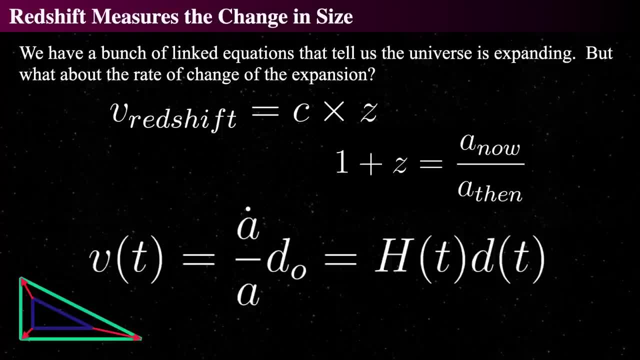 So that's what the a dot over a means, The scale factor itself. So, whatever the scale factor is at a given time, how did it, how is it currently changing with respect to that moment? And that gives you the Hubble parameter as a function of time, of distance today to 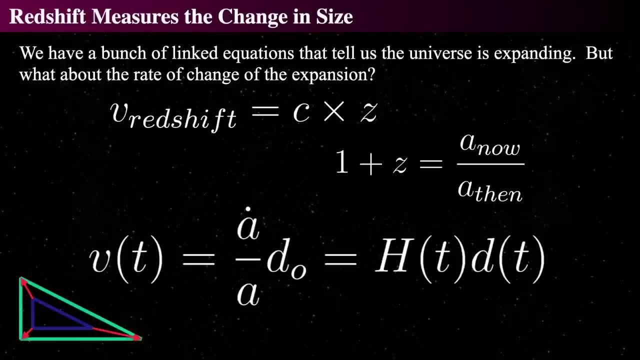 a given object. Alright, So we can then say a very interesting thing: We really don't know a priori how the universe scale factor changes with time. We really don't know that. So the scale factor itself is kind of unknown. so we don't know it. 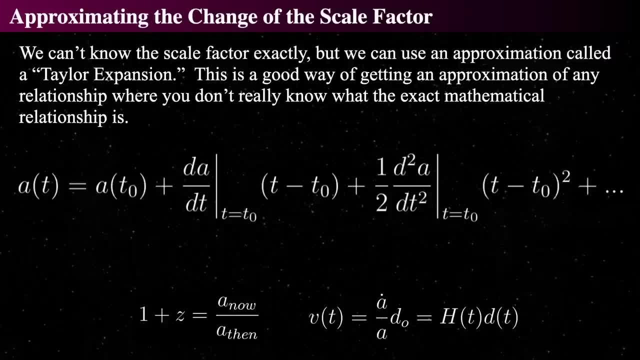 since we don't know it. we can use a mathematical trick, And this mathematical trick is called a Taylor expansion, And this is commonly used all throughout mathematical physics- where what you do is you say: I have no idea how this particular thing is a function of time, or 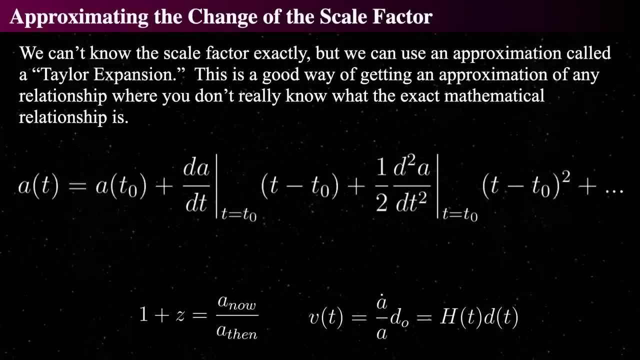 distance or space or what have you. You just have no idea. But what I can do is I can say: well, I know it doesn't vary wildly, I know it doesn't vary crazy time. So what I can do is I can take first and second derivatives of that function with respect to time. 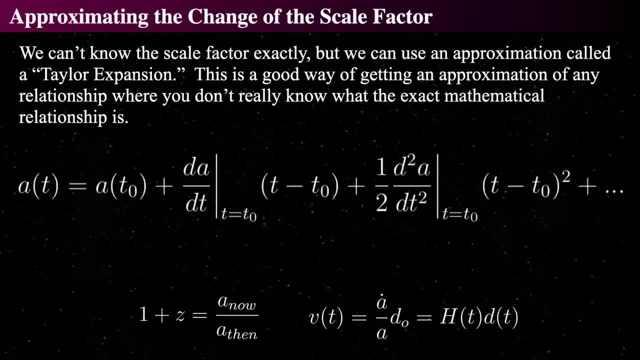 multiply it by the time it has changed by and we can see: okay, take the scale. So we take the scale. factor a is a function of time and say: well, what is it today? a is a function of t naught. 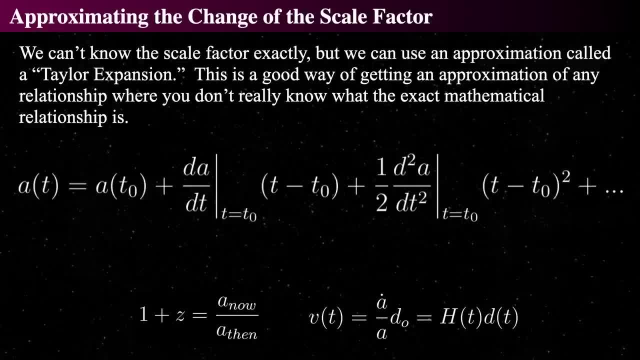 and t sub zero is the time today, So we can say it's equal to that. Fine, So how has it changed? been changing as a function of time? now, How is it changing now? And then multiply it by the time it has changed by the time it has changed. So what I can do is I can 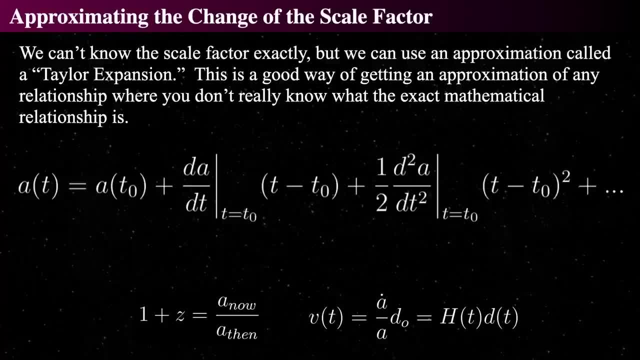 multiply that by the difference in time you're trying to measure, meaning t minus t naught meaning ago compared to today. Then you add on to that the second derivative with respect to time, and that's usually called an acceleration times, the difference in time squared And this sum: 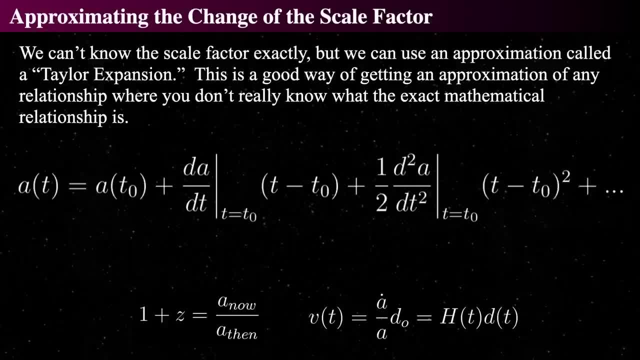 goes on forever. It's an infinite sum and it's called a Taylor expansion. I invite you to look it up if you want. However, what we can do is we can say: this is just a way of saying we have no idea how a as a function of time actually works, So we're going to do a mathematical approximation. 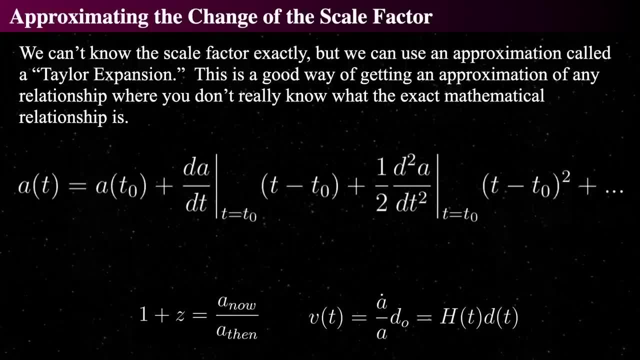 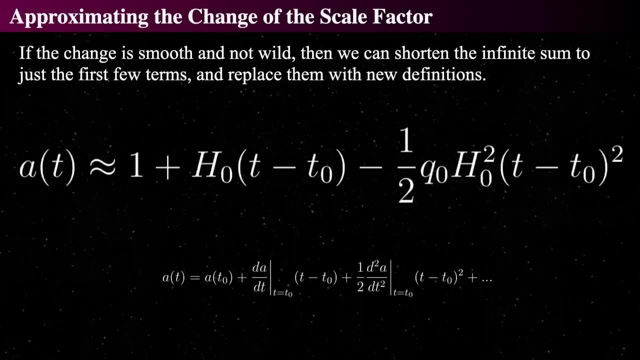 of it, assuming that it doesn't vary very crazily, and that's called a Taylor expansion. It still is a function of redshift and time and so forth. but right now we say it has a function of time, but we really don't know what. it is All right, so then we assume it is smooth, It's. 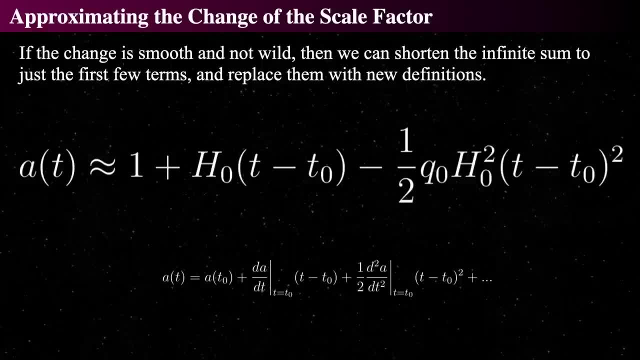 not wild, and so we can shorten the infinite sum to just the first few terms, because if it's not wild, then those little terms are going to vary. very, very short, very small, because a very tiny difference in time, say the t minus t naught, will become really small as time. 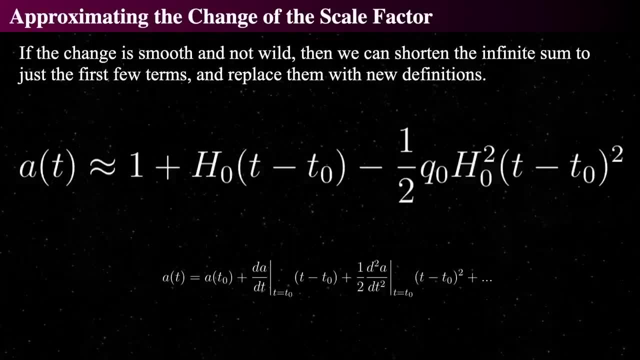 goes on And the higher derivatives, meaning the change of scale factor with respect to the change of the scale factor. with respect to the change of the scale factor with respect to time- you mean like a to the, so how it changes, multiply with respect to time. 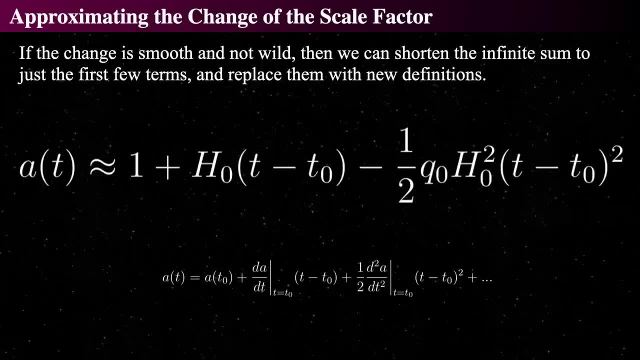 those things are very small changes so we don't really notice them. So there's not a really big acceleration, there's not a really big change in acceleration, there's not a really big change in the change in acceleration. So basically it's moving really smoothly. So if we do that, then 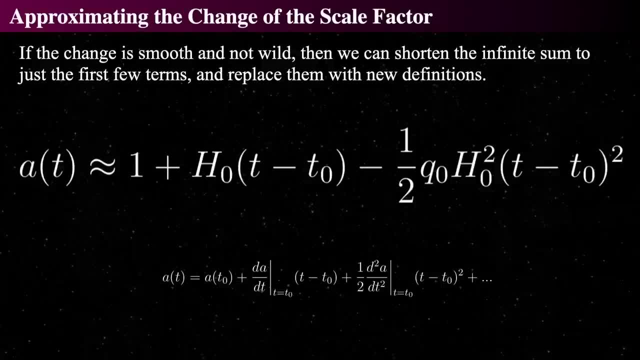 we can approximate that infinite sum with this very simple little equation, and that's what the twiddles is is the a is approximately equal to. That's why we make the bendy line equals. The bendy line equals says that we're making it approximately equal to, And we're also doing 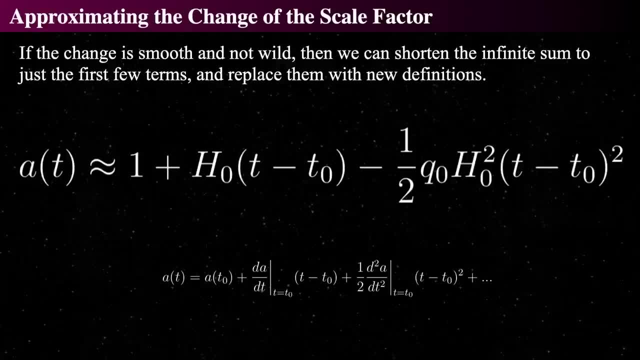 we're saying that the scale factor of today equals one. So that's okay. We've known that, we've done that all the time. So if we have the scale factor today, the scale factor of any time is approximately to one, plus the Hubble constant which we measure today times the time compared to today's time. 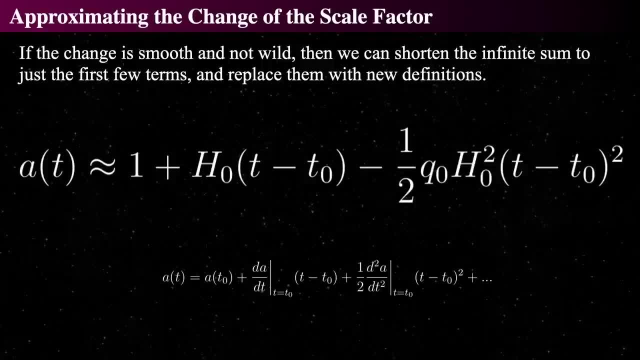 minus a half times this new thing, q naught times the Hubble parameter squared, times the time squared. So we kind of keep that Hubble thing squared. So we have this one thing there, but we have this one thing there. but then the Hubble the q naught is a new thing. And notice we changed the. 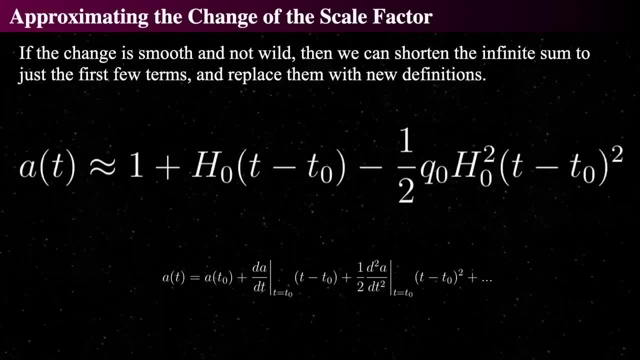 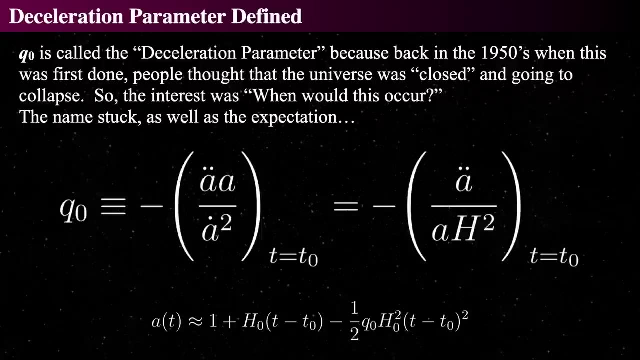 plus to a minus. but all right, that's fine. So we can make a new definition, And this is an approximation, and we define a bunch of things based upon that. So what's this? q naught. q naught is called the deceleration parameter And it came back. it was it was. it arose because back in the 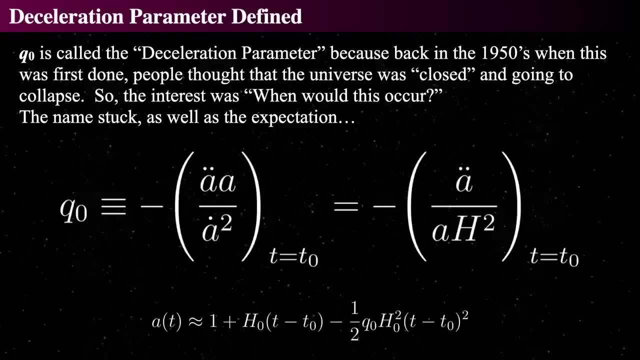 1950s, people knew that the hub, that the Hubble constant, wasn't necessarily the same as the Hubble constant. Or they said: well, perhaps it isn't constant, Perhaps the scale factor and the rate of change of the cosmos expansion has changed with time. So what they did is they said: fine. 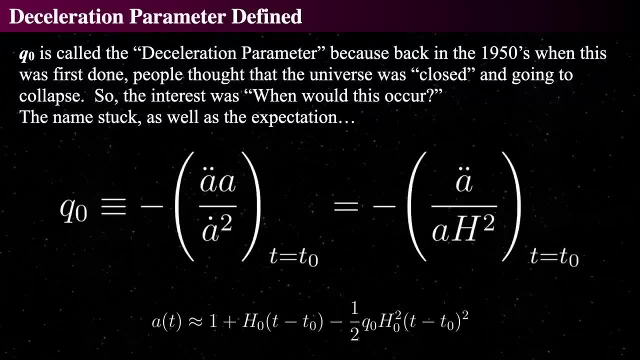 let's do a Taylor expansion, And somebody. somebody figured: well, the universe should be slowing down because it's got a bunch of matter in it. So this was back in the 1950s And people said so, if the universe is going to be slowing down, we want to see how fast it's decelerating. So q naught was? 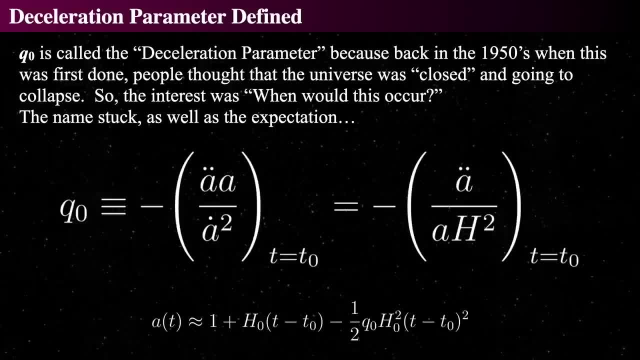 called back in the 1950s the deceleration parameter And people thought the universe back then was closed, that it was going to collapse back in on itself. It was more philosophical than anything else And also because they didn't understand the. 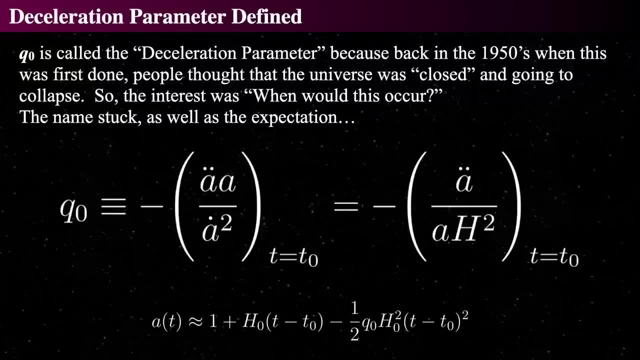 size scale of the cosmos at the time. But it made seemed to make sense at the time. So they defined it to be the deceleration parameter. So they wanted to know when the big crunch would have been, when the deceleration would turn around and how long the universe would live. So q sub naught. 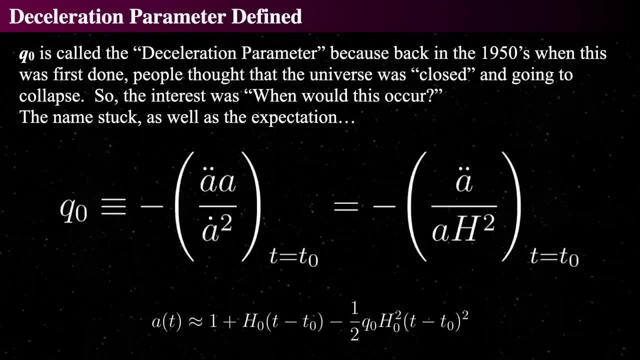 is defined to be- and that's what the three bar is Mean- is defined to be the negative of the second derivative of the scale factor. That's what the a double dot means times the scale factor divided by the first derivative. with respect to time of the scale. 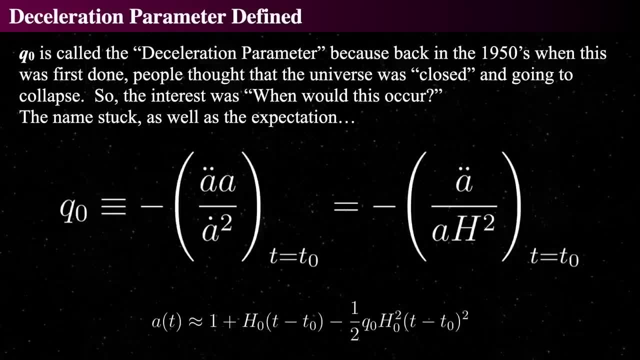 factor squared, And that's kind of a weird way of talking about it. It's a very strange definition, but it allows us to then say: ah, look at, that actually ends up being the acceleration of the scale. factor is a unitless number, So it's not actually a distance, It is a factor that you 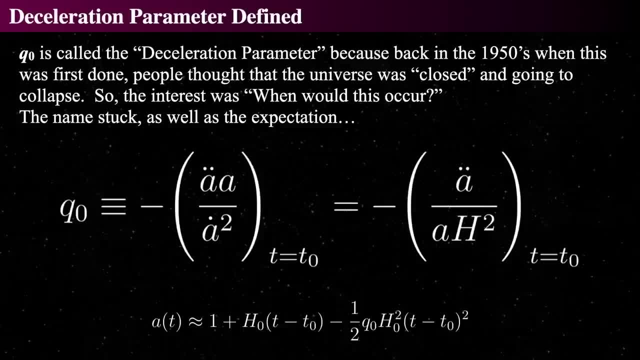 multiply a distance by in order to see how big it is tomorrow as opposed to today. So the scale factor then has a double dot over an a, over the a, and that means it's a second, it's an acceleration, It's a change of time. and the per second per second, per year, per year, what have you compared? 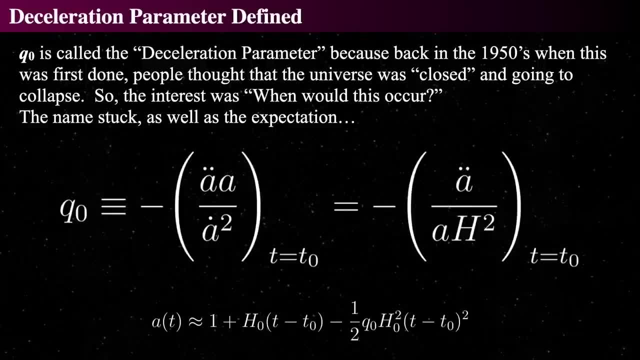 to the scale factor And that's divided by the Hubble parameter, And that's how it's all been defined, And so that's been inserted. that q naught goes back into that equation And this is the definition of the deceleration. 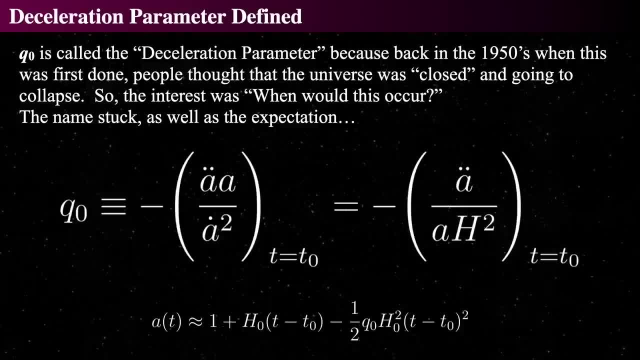 Parameter and it measures how quickly or how slowly the universe is changing its Hubble parameter. Remember, the Hubble parameter said that Edwin Hubble said it is going at 70 kilometer, roughly 70 kilometers per second, per mega parsec, And that's a linear relationship. That's what he. 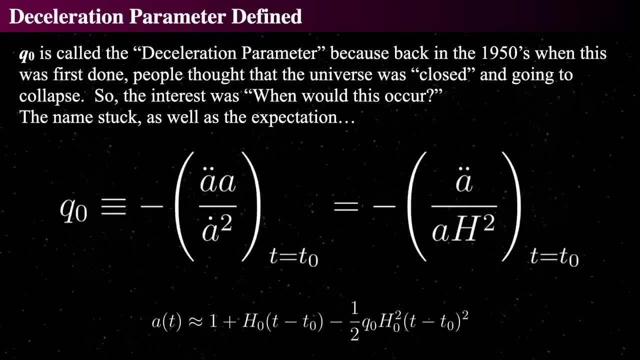 found. But back in 1950s, when people really had no idea, they said: fine, the universe is expanding, There's a scale factor. If that's the scale factor, then maybe there's a change in the scale factor. 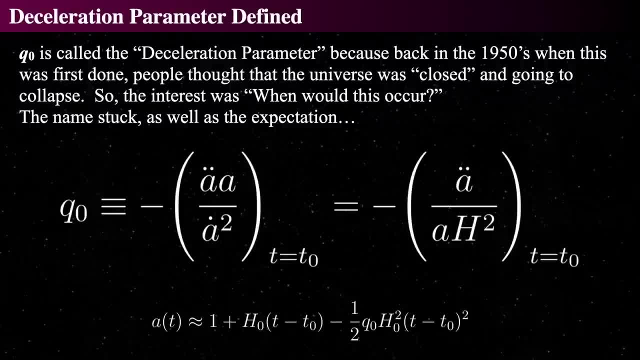 So let's create the deceleration parameter because it's got to be slowing down, because matter pulls on matter, So it's expanding, It's probably slowing down. So let's define it this way, And so they did. Now the deceleration parameter can then be plugged back into another very important 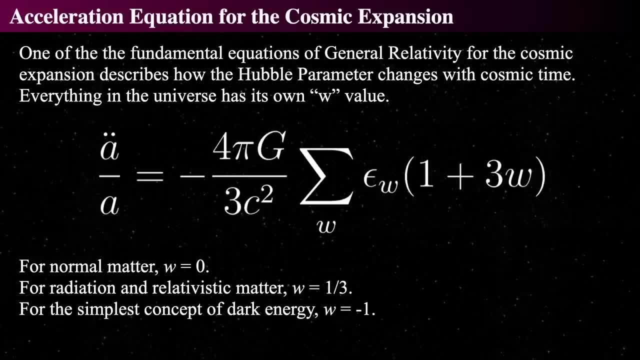 equation from general relativity, And that is the one of the other fundamental equations that arises from general relativity and cosmology, and the simple, the simple concept of an isotropic, homogeneous, expanding universe is that the acceleration parameter double, a double dot, compared to the, to the scale factor, The, so the left-hand side acceleration. 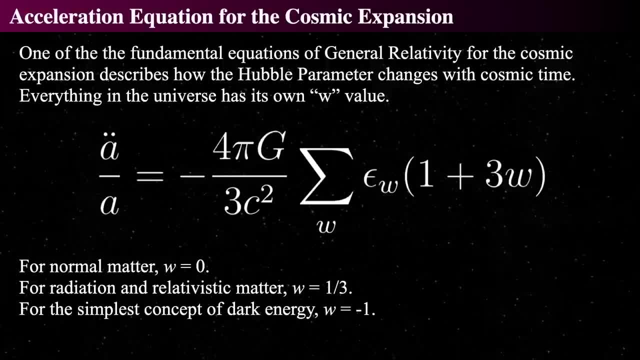 equation is equal to some crazy bunch of numbers: four pi times the gravitational constant divided by three times the speed of light squared. And that big sigma, that big letter E, which is a Greek sigma, means the sum of and the little w means a bunch of things like w, some of all w. 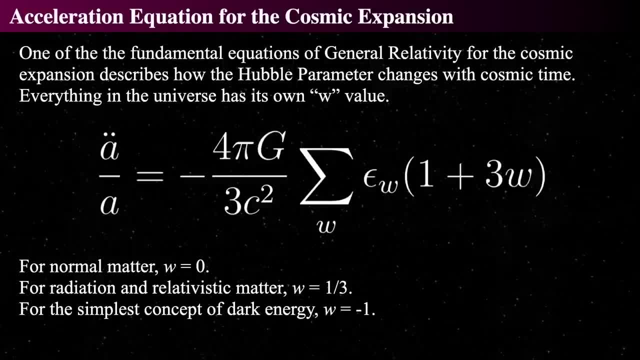 where the sum is the things to the right and e is the energy density of one parameter of w. so maybe energy transfer this or energy density of that, and then times one plus three w. so every energy density does something different to the acceleration parameter. now for normal matter. 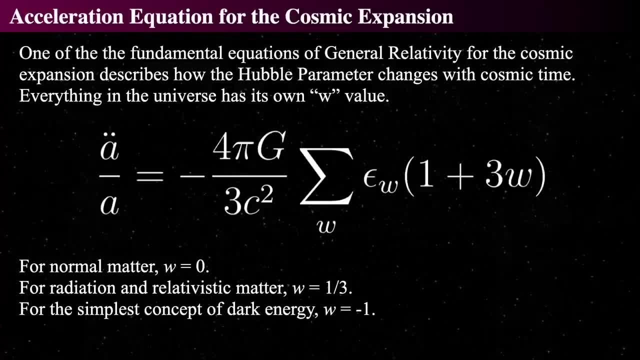 like. like atoms and molecules and even dark matter, the w is zero because it doesn't do, and it it doesn't doesn't do anything different to the acceleration. either it's there or it's not. it pulls by gravity. it does nothing any different, so it just behaves like normal energy density. that 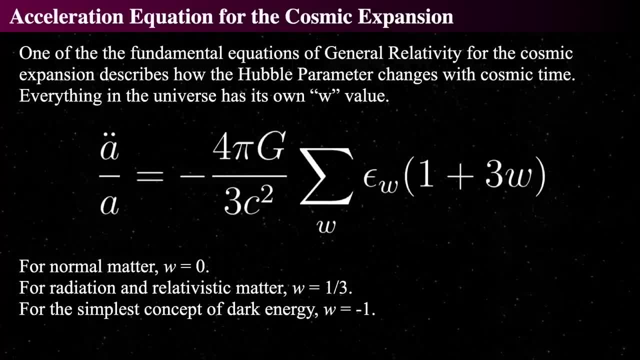 we perceive. for radiation like light or neutrinos, w is equal to one third. so that changes the little thing to the to the right. so that becomes two e w right. so you get this one third, and it's what? two times e w. so whatever the energy density, 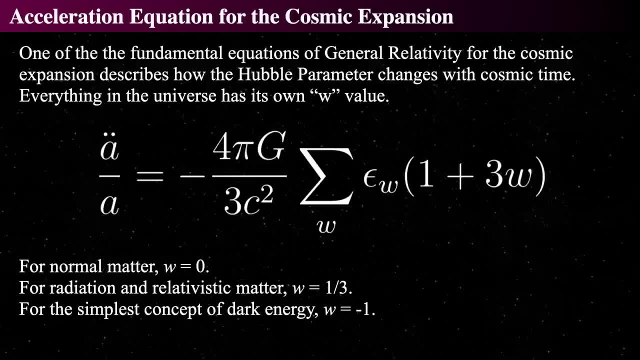 e sub w is for for radiation, whatever that is, that's what it is. it's twice that, that's so. it contributes twice as much to the acceleration as normal matter. and then if we say some concept like dark energy or more specifically what einstein called a, 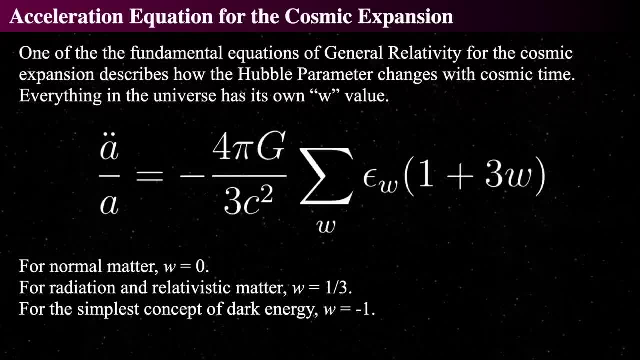 cosmological constant. we would plug in: w is minus one, so then that becomes a. if w is minus one, then that thing on the right becomes negative, two, and then the acceleration. if you look closely it becomes positive, and that becomes the instead of a deceleration. this whole thing's been 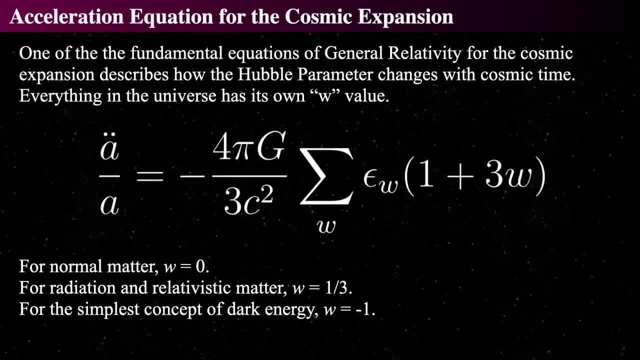 defined in terms of a negative acceleration. a negative acceleration is a deceleration. everything is a deceleration. so matter provides deceleration because on the right hand side it stays negative. radiation, like light, provides a deceleration because everything on the right stays negative. 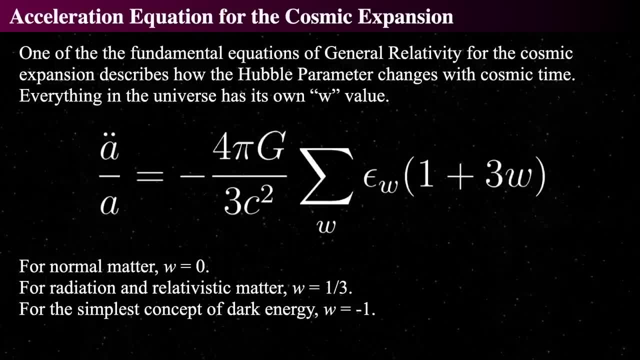 however, for dark energy, if you plug in a minus one into w and you see just the components who make it negative. so we're going to add together normal matter and radiation and dark energy or anything else. we don't even care, we just have to know what its w is. maybe there's some crazy sort of thing. 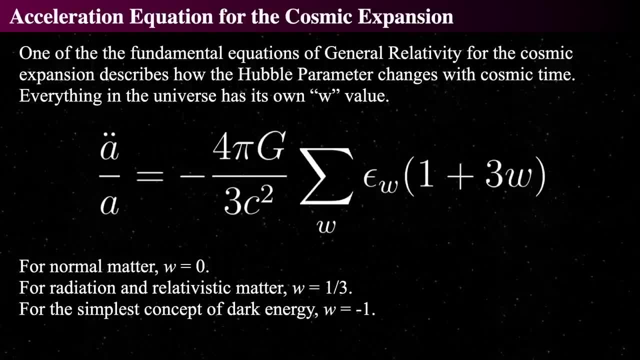 where the w is equal to like four or minus a minus one-third, or maybe it's equal to like, uh, one half or something. maybe there's a different w so you have to say, oh they, energy density of the stuff, that is, w equals one half. but so far there's only really three things that we care about: normal matter. 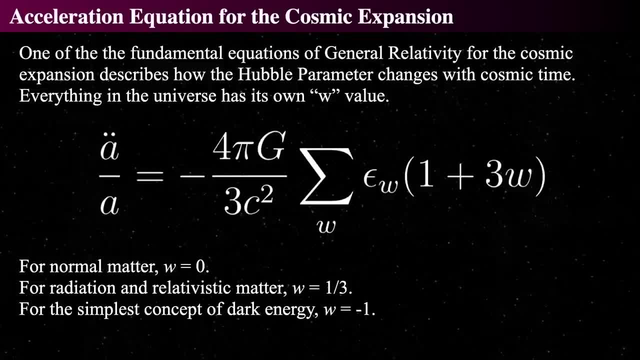 light and maybe dark energy or cosmological constant. so notice that if you plug in minus one for w and consider only that and get rid of the sigma with the w below it, then it becomes positive and it's an acceleration as opposed to deceleration and that kind of helps, because when 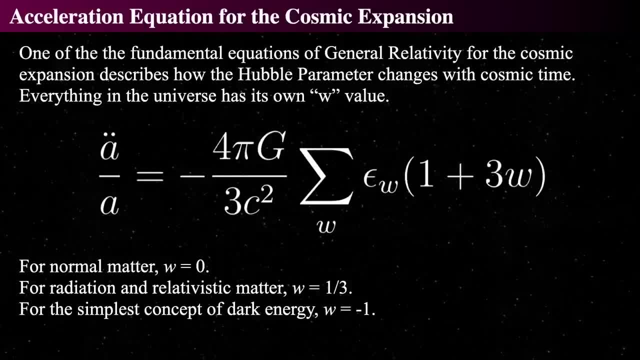 d it? well, because when einstein first created the cosmological constant, remember, he thought it was done to balance against the pull due to matter, because matter would pull as a negative. so he said: let's throw in a cosmological constant and have it be this stuff that pulls, that pushes. 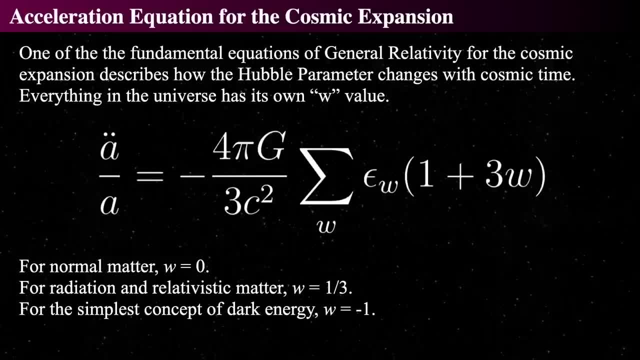 and so he said that would be a negative one. and that's where it comes from. that's why even anybody was even thinking about it. now the acceleration equation can be twisted and turned around, and something can be done slightly differently. we can define it in terms of the deceleration parameter. 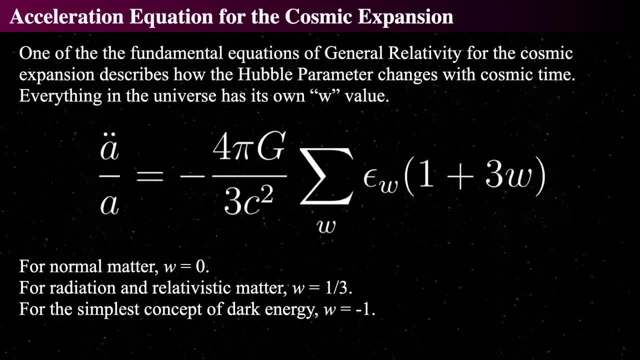 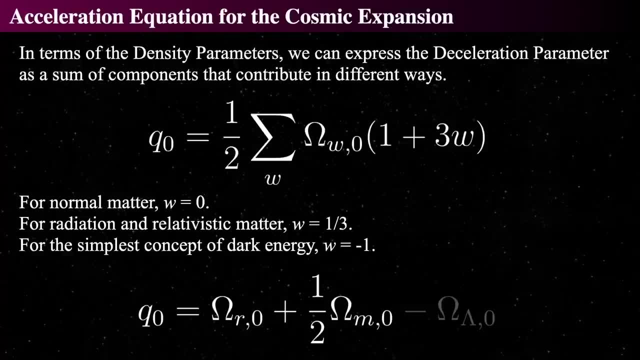 this equation can be defined that way. so let's see how we can do if we do that, if we define that equation in terms that the deceleration protein parameter q naught, and instead of energy density we use the density parameters, those omegas, which means how are they compared to the critical density and we would say the sum of all of the? 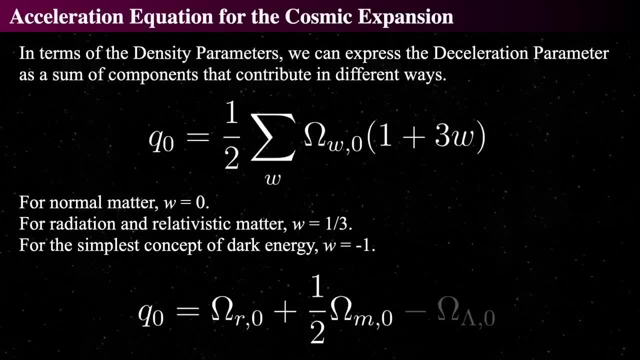 omegas at of different, different components. w's times, whatever that fracting off is to the right. that gives you the deceleration parameter. so let's see what that equation looks like more simplified. the deceleration parameter for normal matter, remember. w zero for radiation it's one-third. 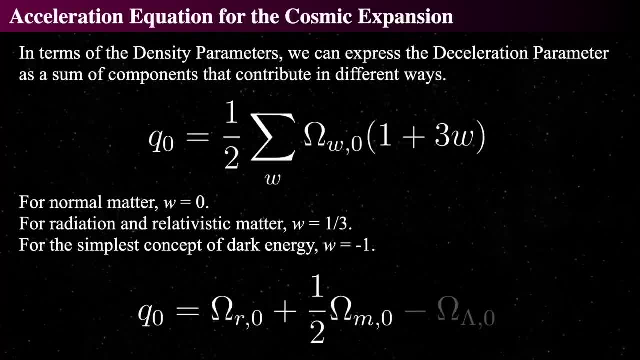 and dark energy or cosmological constant. it's minus one. now, cosmological constant, i graded out because that lambda would be constitute, would make the cosmological constant and that's what einstein did to put in there. and he said, oh, there's no evidence for it. and once he found 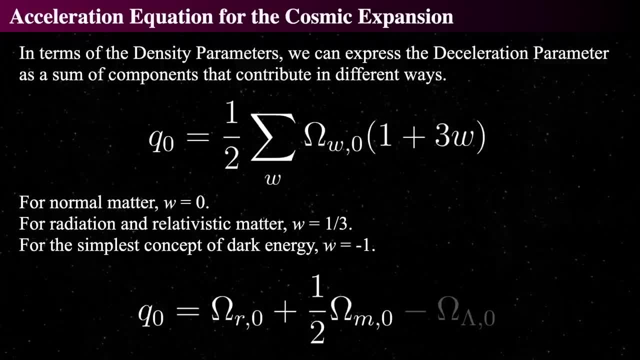 the hubble's expansion later. because einstein thought the universe had to be static, so he plugged that in in order to, to give something to, to keep the universe from collapsing. it's because he figured: oh, the universe is out there, it must be collapsing, so i'm going to push, put this thing in there, to force it apart, and that's. 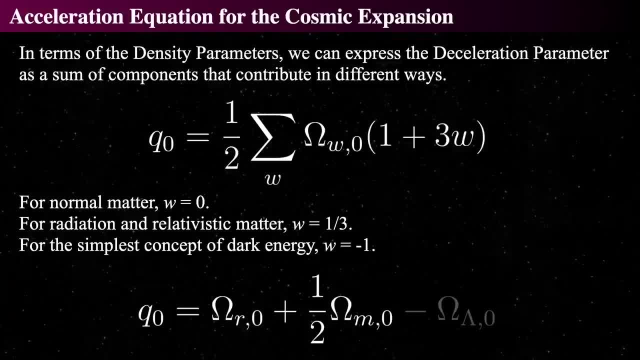 the cosmological constant, which has a w of minus one. so what he did is he tossed that in there, and so, in einstein's tradition, he lit. when he found out about the expansion of the universe, he said, oh, this is terrible, this was the greatest blunder of my career. so he removed, he disavowed the 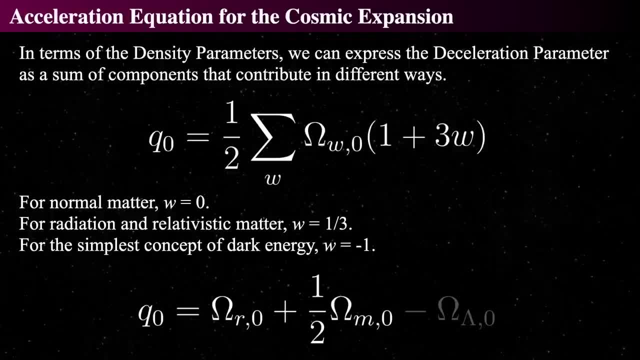 cosmological constant, but wrote about it and talked about it and the mathematics was done. so people kept it around, just as you know, put on the shelf. so but but after einstein people said, well, there's no, they didn't think of that anymore, they didn't think the universe was static anymore, so they didn't see a. 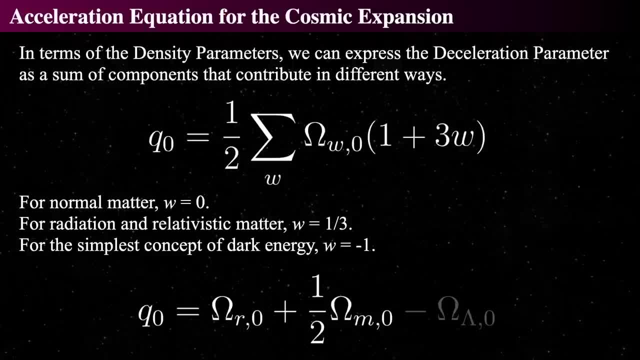 need for it. so they only thought of the first two that are not grayed out. they said: what is r for radiation and what is m for normal matter? so that is the deceleration parameters for both. and so it's like, well, okay, what's the? what's the? 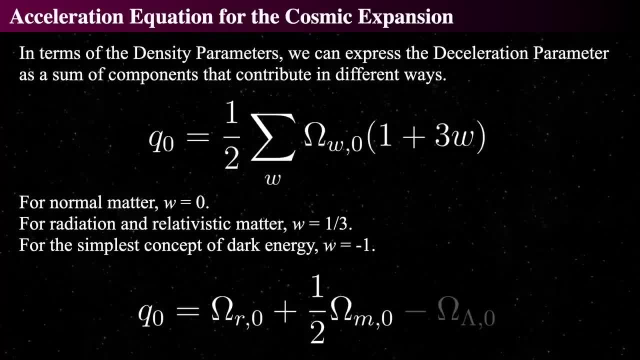 constitutes. how much of the critical density is there? because if the deceleration parameter is positive, then it's decelerating, and if it's negative, then it's accelerating. so that's how we would look at this. so the question is: how much deceleration is there? how much matter is there in? 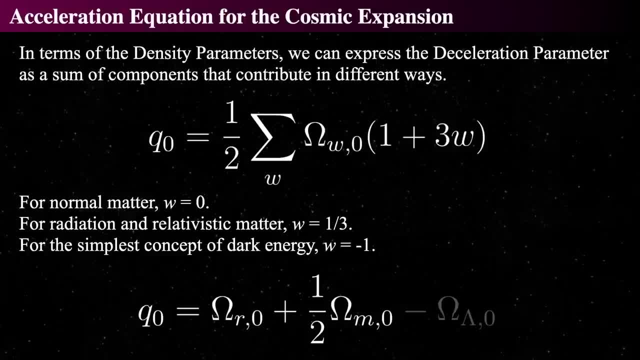 the cosmos? how much energy density is there from the cosmos? because looking just at this equation is for the Bewängen theorem. how can we generator that mess around like that in order to get here the solution? another equation would be that whatever we haven't seen, what the으면서? 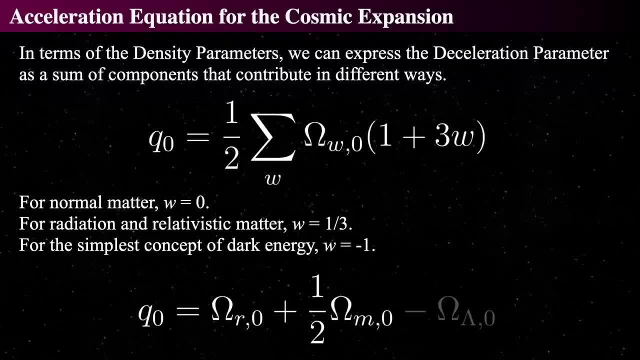 we can convert to energy density is that we can't never be negative of a matter, so you never do energy density, and we can determine that because, again, what energy density left over now? and so here's the solution. okay, so thus we need to go back to our разбikier. 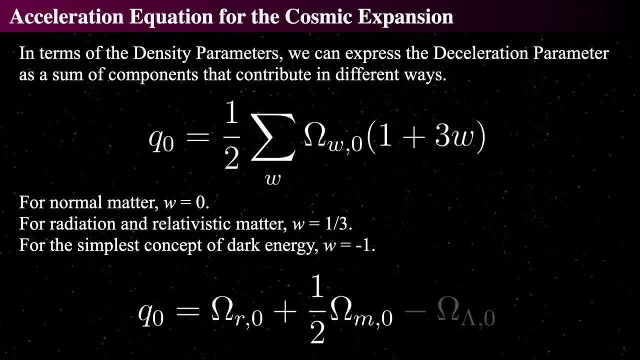 problem. and then we can still think about in terms of lincoln, this condition which we even mentioned before. we can�now describe how much mix in like this we can think about that comes from that. so the energy density and the omega of emas ohm becomes negative of a serom- some other i have in. 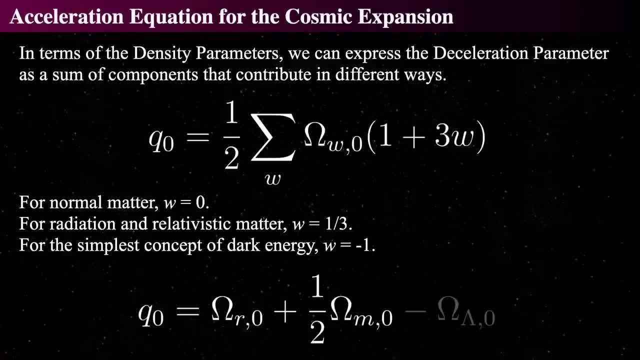 this. i can think of that kind of phenomena, so that's why i grate out the thing that's. it's always easy to literally degrade the term can another and will not destroy matter. but that's also suffering from like brighter energy density. much stuff is in the universe. to determine the deceleration parameter. 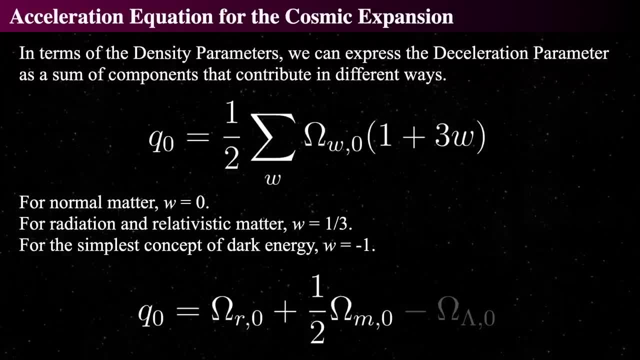 And that was consumed most of cosmological study from the 1950s all the way through the 1990s. It was a 40-year quest to understand both the Hubble constant and the deceleration parameter. I remember that from college. 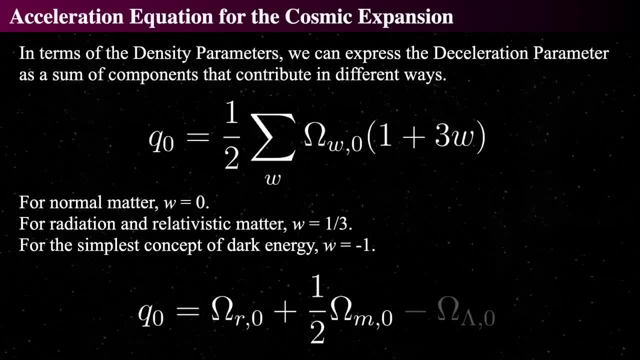 It was like the quest for two numbers: H-naught and Q-naught. What are they? That determines the future of the cosmos. That was a big deal. It still is, but it's not as big a deal today as it used to be. 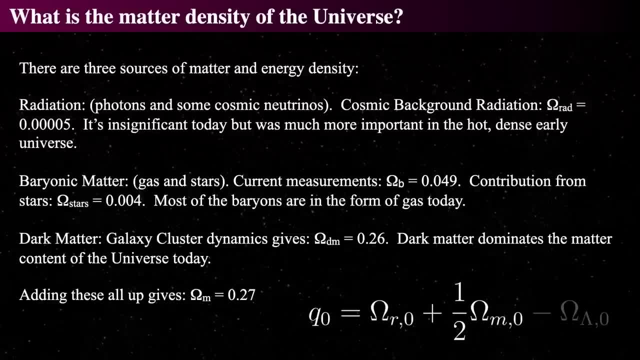 We'll find out shortly why. What are these things? Well, there are three sources of matter and energy density in the cosmos that we know of, that we can easily measure or, for the purposes right now, Radiation, which is photons, and a lot of cosmic neutrinos. 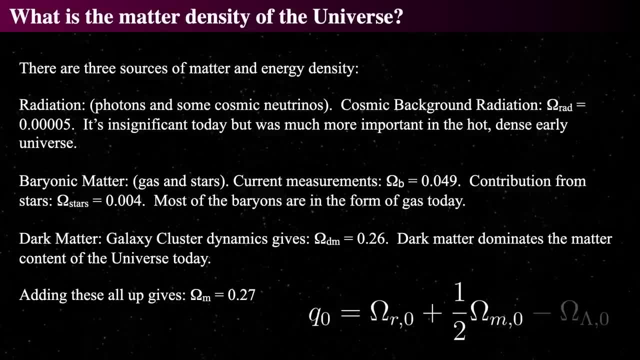 We know neutrinos are out there in scads because of supernovae in the sun and so forth, But all of that, the neutrinos are swamped by the energy density of the cosmic energy density of the cosmic microwave background radiation. But that's an incredibly tiny part of all the energy density because the universe has 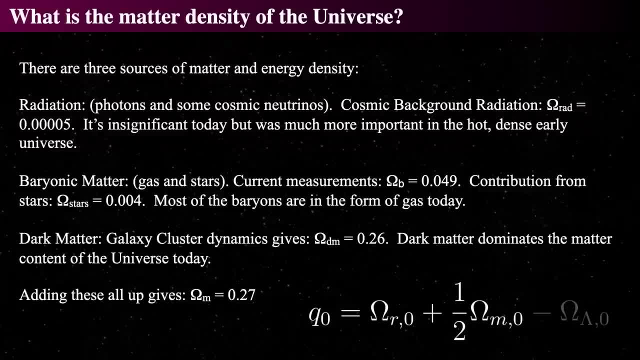 stretched. it has stretched the photons to the point where they're microwave photons. Now, if you went back in time, they'd be the same number of photons, but their lengths would be not as long. their energies would be higher. they would actually be much more. 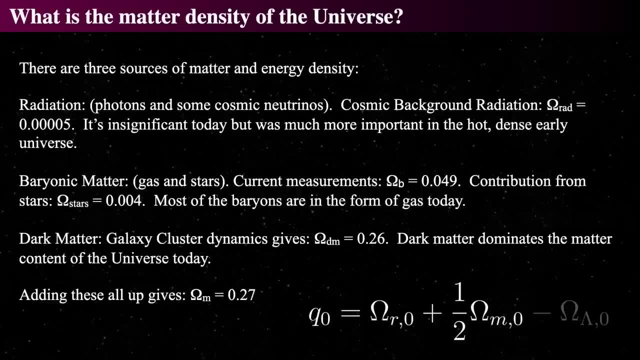 dense, And that's why, when we look at the early cosmos, it's radiation dominated, but the later cosmos becomes matter dominated and otherwise dominated. So the cosmic microwave background and all photons from all stars, actually photons from all stars in the universe that have ever been made, and all neutrinos that ever been made. 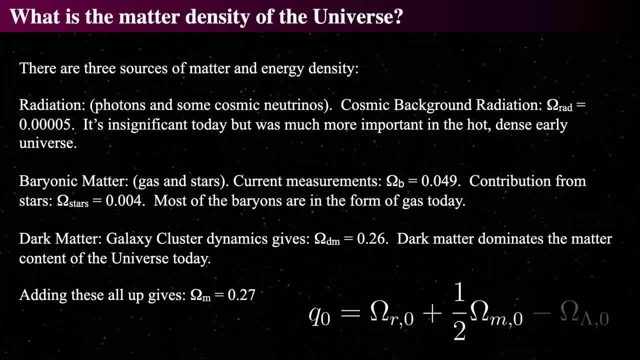 are less energy density than the cosmic microwave background, So light doesn't do too much, So we can basically ignore that part of the thing. So our next step is: what are those? normal matter? and normal matter, it can be called baryonic matter. 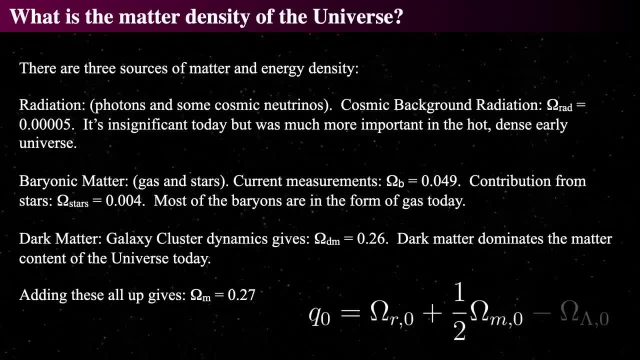 And that's kind of a weird word, but I'm not going to get into why it's called that- But baryonic matter. Baryonic matter is like gas and molecules and stars and planets and people. So that's baryonic matter, normal stuff that you stub your toe on and that you eat for. 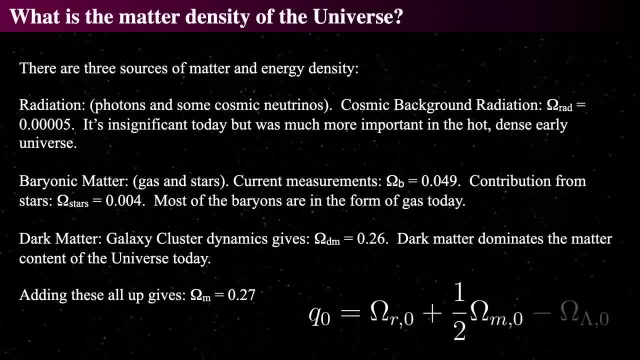 breakfast. That's baryonic matter. So the current measurements of normal baryonic matter across the entire universe are about 5% or 4.9% of the critical density of the universe is in the form of baryonic matter. 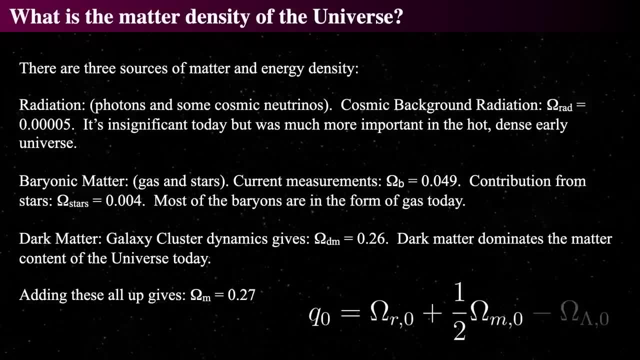 And that is interesting because if we say, then most of the baryonic matter that we would encounter, planets are really small compared to stars. So if we then say what is the contribution of baryonic matter from stars which is like the sun and Sirius and Betelgeuse, that's really tiny. 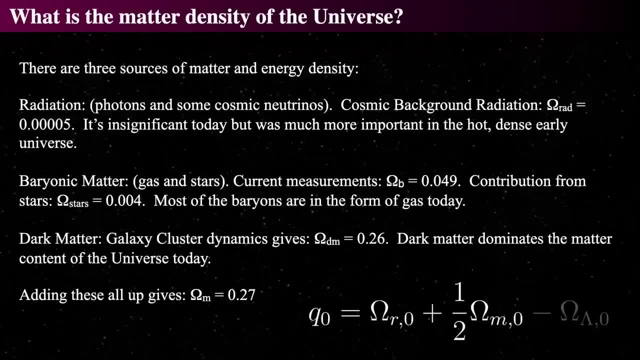 That's four percent, four tenths of one percent. So most of the baryonic matter is in the form of hot interstellar and intergalactic gas. So stars make up almost just like only 10% of the normal stuff. So most of the baryons are in the form of intergalactic hot, hydrogen and iron gas permeating the galaxy. 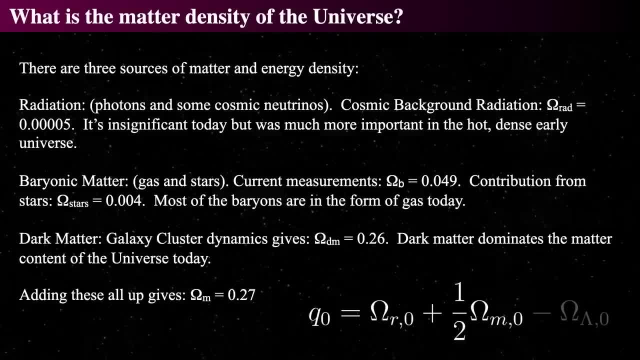 clusters And that's what we saw in cluster physics previously. However, we found that dark matter, because of cluster dynamics and how the Milky Way is rotating and how galaxy clusters fit together, that actually galaxy clusters show that dark matter constitutes about 20 times the amount of baryonic matter in the universe. 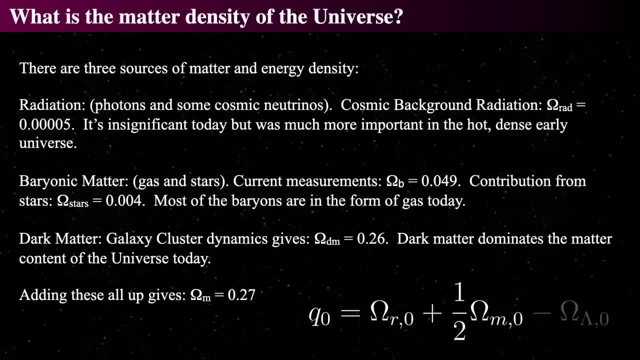 Wow, That's 26%, or is 26% of the critical density? So, essentially, adding everything up there, So dark matter dominates the total matter content of the universe today. So, of all matter, if you add it all up, it gives you only 27% of the critical density. 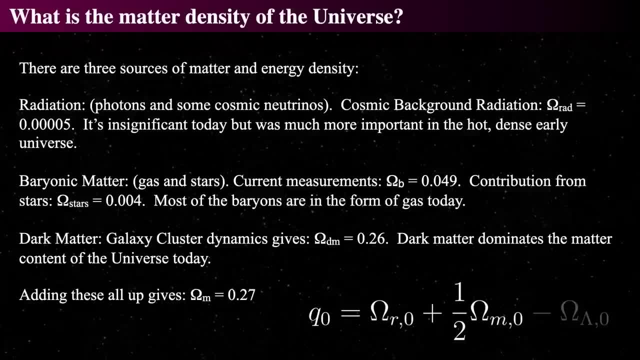 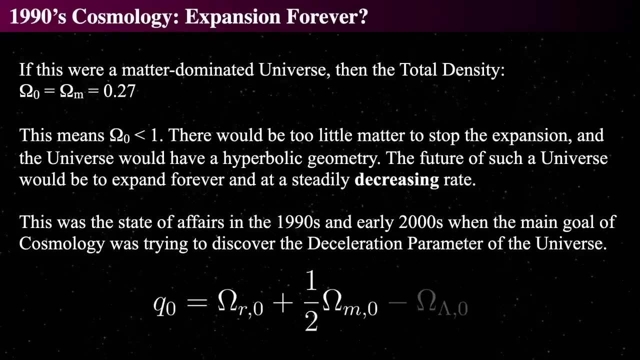 So it's not enough to make the universe flat. It's less than flat. So therefore it is under the. it's an under critical density universe. So what does that mean? So the universe would be matter dominated. If the universe were matter dominated, then the total density of the universe right now, 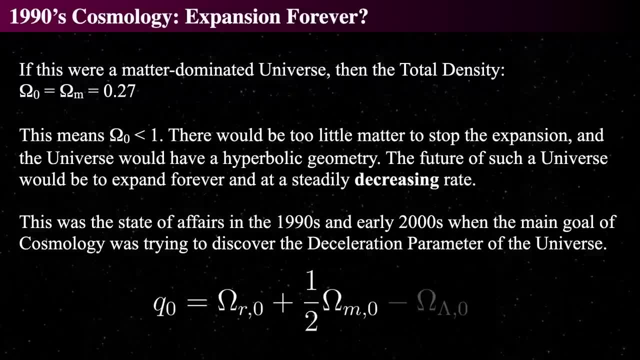 that's what omega sub naught means- is basically equal to the matter density, which is 27% of the critical density. That means it's less than one and it's too little to stop the expansion. That means the universe would have an open hyperbolic geometry. 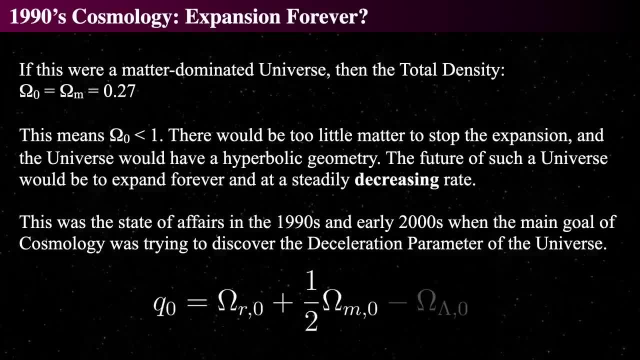 That's. we saw that with that weird saddle shape There's no funny effects like the like, the like the spherical geometry, And it would be. it would be open and it would expand forever And because there's matter in it, that expansion forever would decrease very steadily. 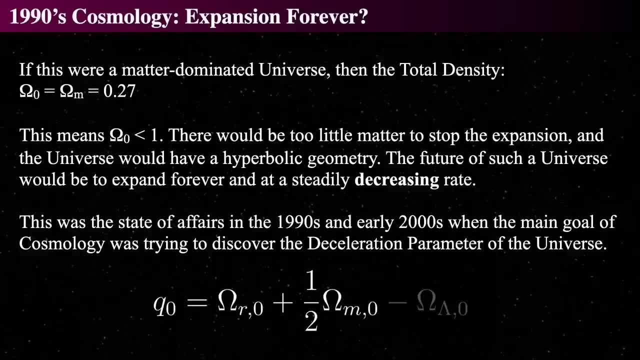 And that's if you only have that in it. And during the 1990s, when I was in grad school, that was exactly the state of affairs And the main goal of cosmology was to actually determine this deceleration parameter and 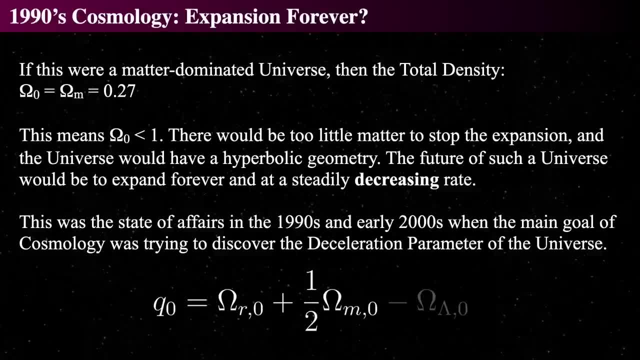 prove whether or not this is true. Okay, So let's start by looking at the global deceleration parameter across the entire universe, whether or not this was going to hold up everywhere, because cluster dynamics for one thing, Milky way rotation is another. but let's look at the entire universe and see if we can figure. 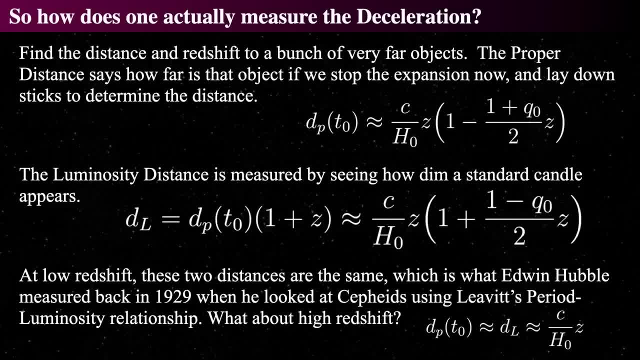 that out All right. So how can we detect the deceleration? Well, first things first. we've got to have a couple of things We're going to now write. we can say the proper distance. So we want to know to get deceleration. 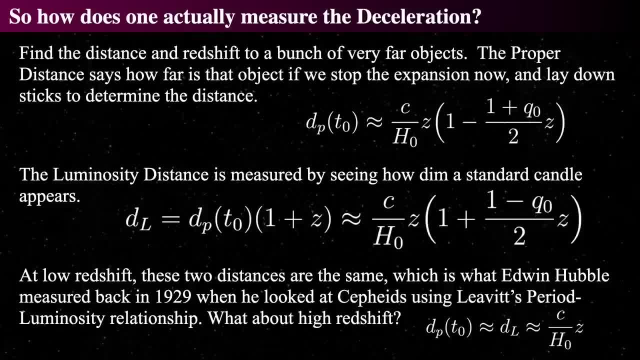 We need to know how fast. two things are right: Are rushing apart or falling together. We want to say: how far are they now, How far were they then? How far are they, How fast are they going apart? And that concept relates to an idea of farness. 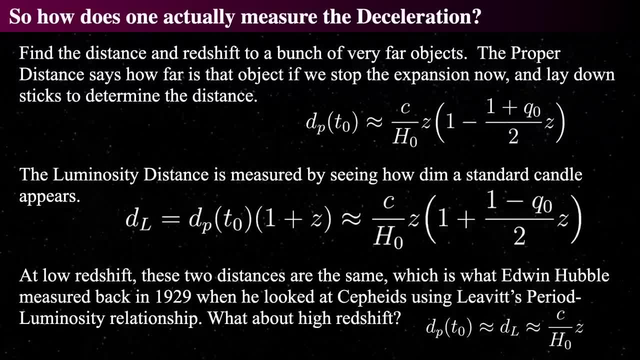 Yes, And the base idea of far is called the proper distance. and the proper distance in cosmology is to say: stop the universe. Imagine you could stop the universe's expansion. Just imagine you could do that. Just put on the brakes for as long as it takes and lay down a whole bunch of sticks to determine. 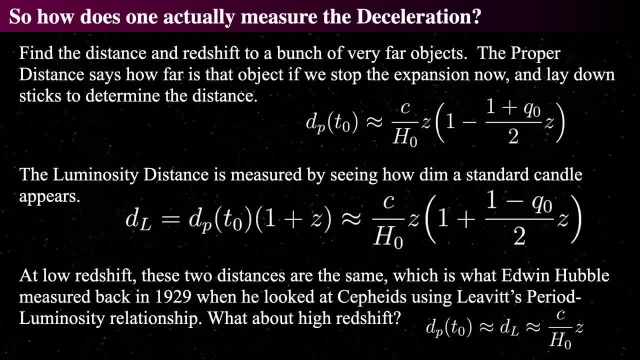 the distance to something, And that's called the proper distance. So you, what you do is you'd stop the universe's expansion for a short period of time And then you'd say: what's the red shift to that object? And that's the Z in this equation. 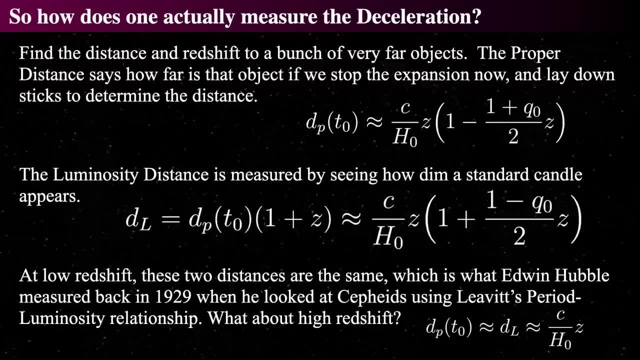 And what is the measurement of a bunch of Zs And you'd have a proper distance to all of those things. Maybe you see, you know how bright something is in there, Like somebody put a hundred, a hundred billion, Yeah, A billion, exactly 10, a hundred billion, uh, uh watt light bulb in each galaxy. 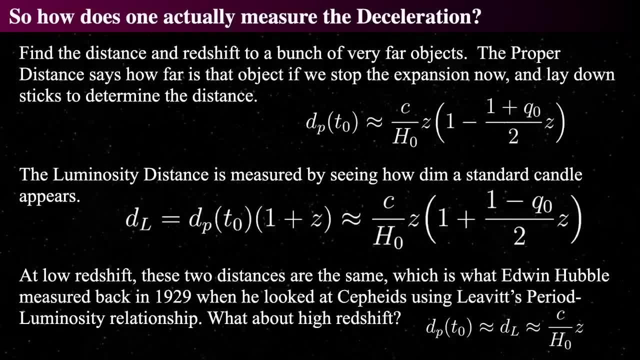 And because each one is exactly 100 billion Watts, you know how bright it should be. So, since you know how bright it should be, you know the distance, the proper distance, because how bright it is, All right. So that would give you this. however, we don't, actually we can't stop this. 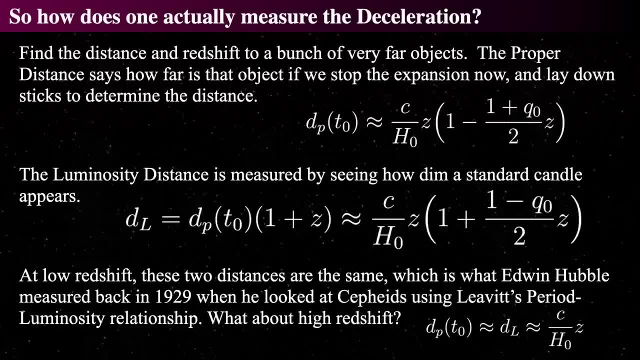 So the proper distance. So the ruler assumes that we can do this. but if you could somehow measure down the ruler sticks, that would be the proper distance And then you'd measure the red shift from that galaxy to that galaxy at that moment that you laid down all the meter sticks. 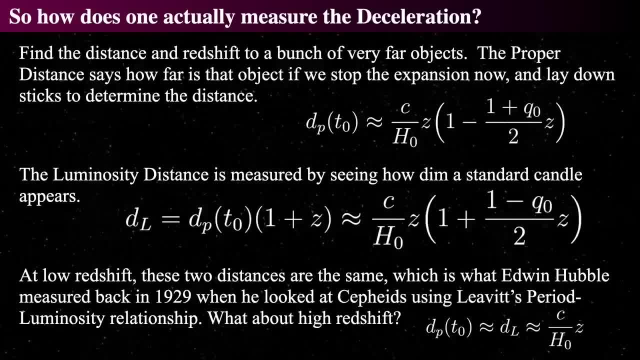 And that would give you, for a large number of objects, a statistical study that would give you H naught and Q naught. However, what we can actually use that's better is called the luminosity distance. The luminosity distance is actually um related to the proper distance. 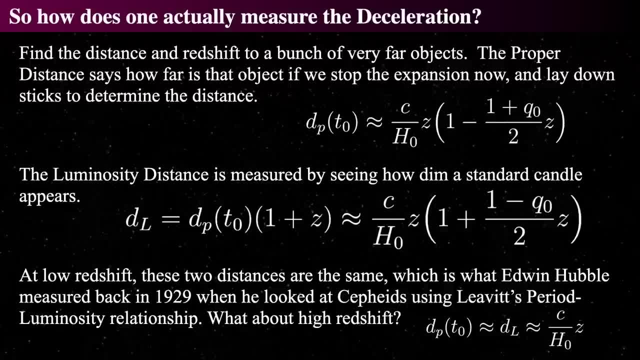 So we can actually use that. So the luminosity distance, the luminosity distance, is actually um related to the proper distance. The luminosity distance is related to the proper distance, which is what you really want to get. You really want to get the proper distance, but the luminosity distance is related to. 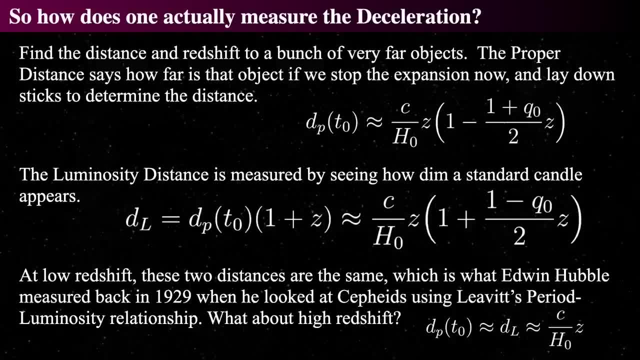 the proper distance. Luminosity distance is what I just said a second ago. Imagine you know how bright something is. how bright does it appear to be Now? that is dependent upon the distance. Remember the distance is changing. Since the distance is changing, then it is affected by the red shift. 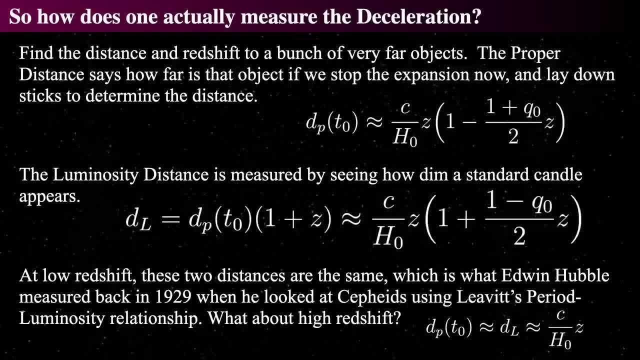 The red shift, the expansion of the universe actually affects that, So you have to take that into account. So the luminosity, the brightness or the distance you would measure by knowing how bright something is and then measuring how bright it appears- is affected by the red shift. 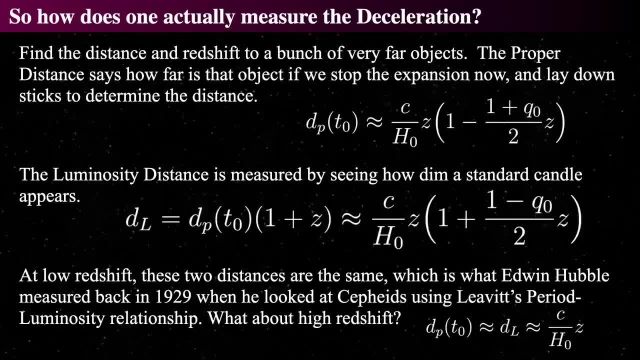 So you have to fold that in. That's where that one plus C comes from, And that's approximately equal to a slightly different equation. They're almost identical. You can see how the minuses and pluses are swapped, So they're almost identical. 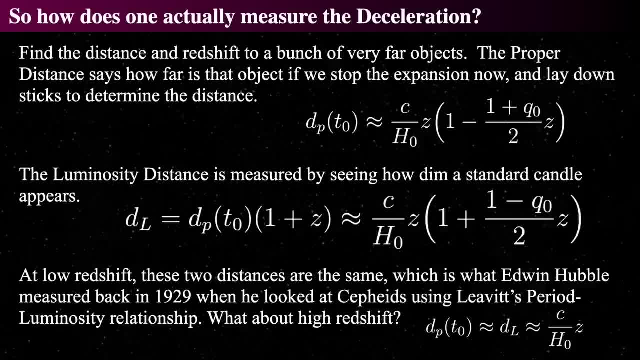 So that's the approximation equation, And so when you measure something, you want to find something. that is where you know how bright it is, And that's what Hubble did. He knew how bright the Cepheids were because Henry Leavitt created the period-luminosity. 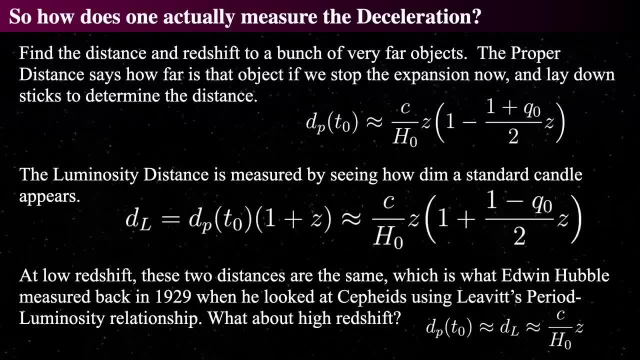 relationship, And so if you have a period-luminosity relationship, you're measuring the luminosity distance. However, at very small red shift, they're the same thing. If you look closely at this thing, you see a z squared in there. 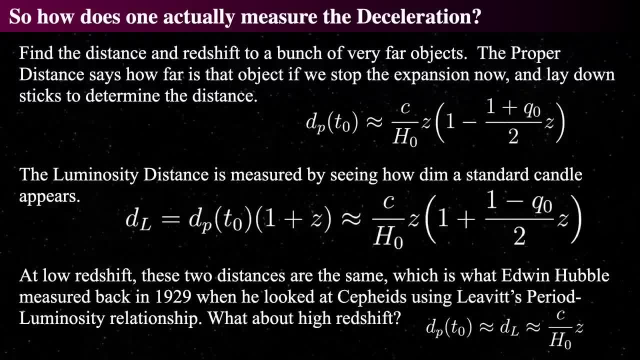 So at small red shift, the z times the z is going to be even smaller. So it's approximately just the thing that Hubble did, And Hubble only looked at it. He only looked at small red shifts. So he could never have perceived the deceleration parameter at all in anything, because he was 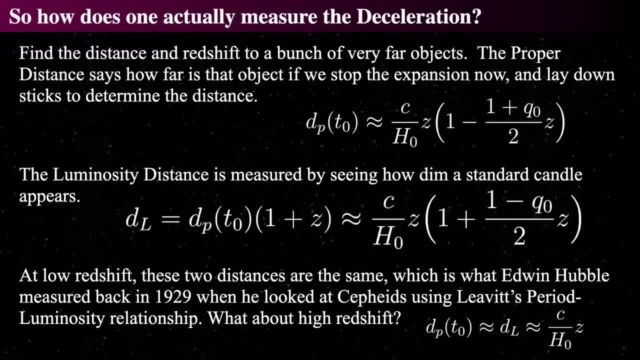 looking at things that were simply too close. Tens or hundreds of megaparsecs is simply too close to measure the deceleration parameter- Isn't that wild? We have to get something larger than 100 megaparsecs to begin to see this. 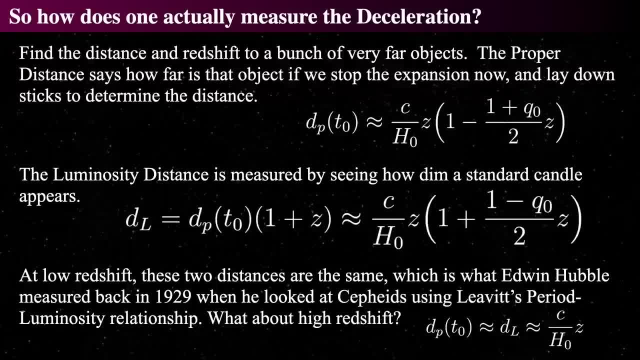 So we need something really, really, really bright. So Hubble measured a very small measure close by And that's why we see the little equation down on the right, Because that's because we take a z, because in the approximation that we have in the middle, 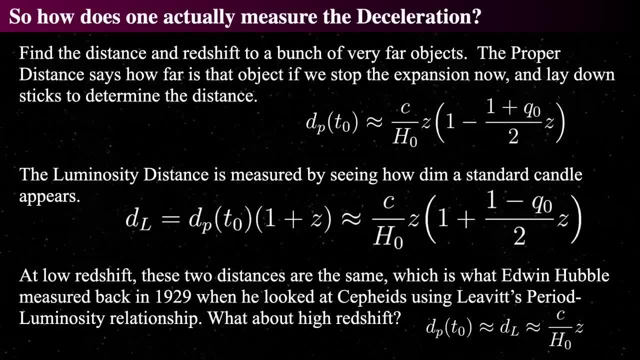 the z times. the z is going to be really small, So the deceleration parameter basically gets hidden by looking nearby. So what do we got to do? We have to look at high, high red shift, very large red shift, so that we can actually perceive. 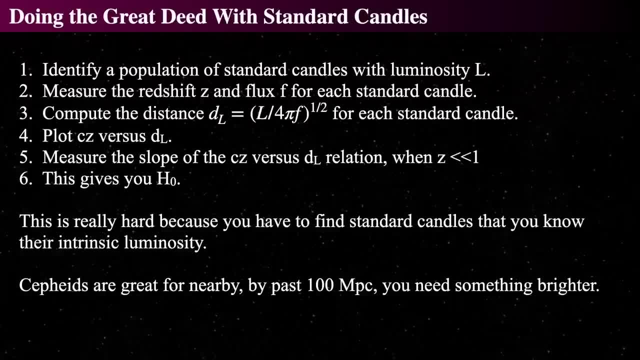 the deceleration parameter. How do we do that? Well, first we're going to find a population of things- It's called standard candles, that we know their luminosities. Hubble used the Cepheid variables. We can use other things. 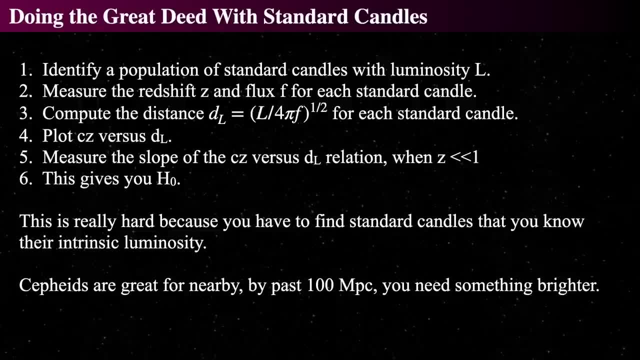 When we talked about the Tully-Fisher relationship in the past, we talked about Type Ia supernovae as well, and supernovae and brightest red stars, surface brightness, relationships, any number of things, the brightness of the core of a galaxy, the rotational, the profile of an. 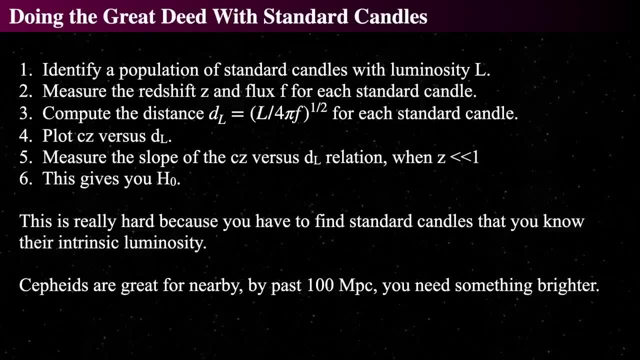 elliptical galaxy. There's many ways to do this. Some are better than others, Some are really good, Some are really bad. But you know, these things are billions or light years away and they're looking at stars in large numbers. 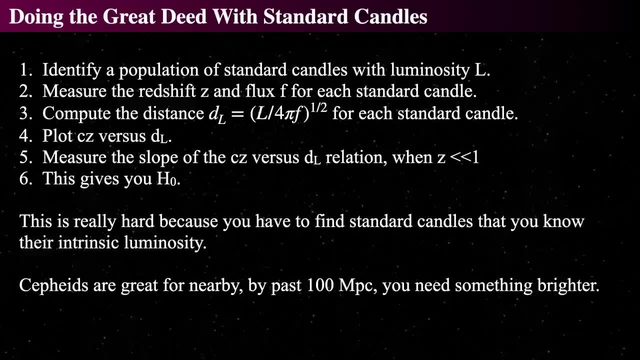 So it's going to be kind of a trick to get anything anyway, but let's pretend we can. So you measure the red shift to that thing and measure the flux, which is the brightness, the brightness that you get for every standard candle, whatever that standard candle is. 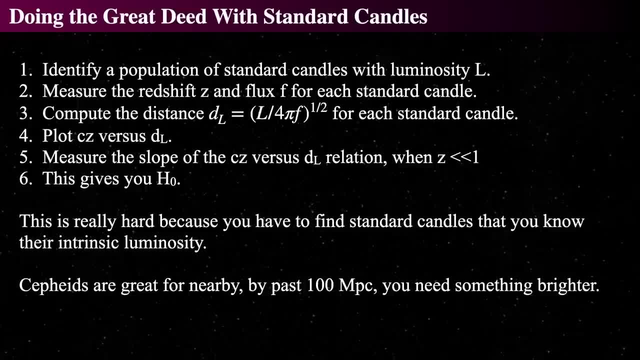 And then you compute the distance, the luminosity distance d sub L, And then you know what the luminosity of the thing is A priori, because you know how bright it is from physics. Physics says this thing must be this bright. 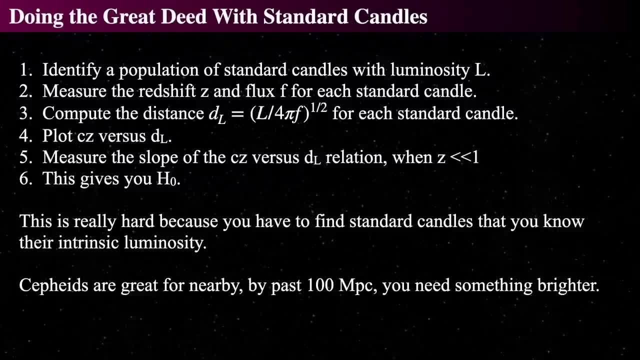 Okay, You compute the distance based on the measurement you take, with the flux and the red shift you take, And that gets you that for every single one of your standard candles You then make a plot of the red shift, C times the red shift versus the luminosity distance. 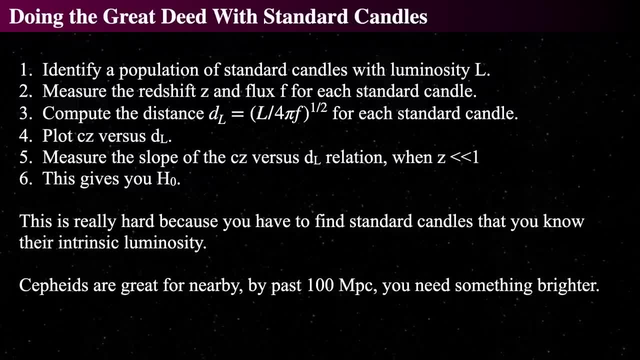 And that gives you the slope of that line, gives you, gives you, when it's very, very, very low, That's going to give you the H sub naught when it's low, low, red shift And this process that we just described, those six steps, that's what Hubble did. 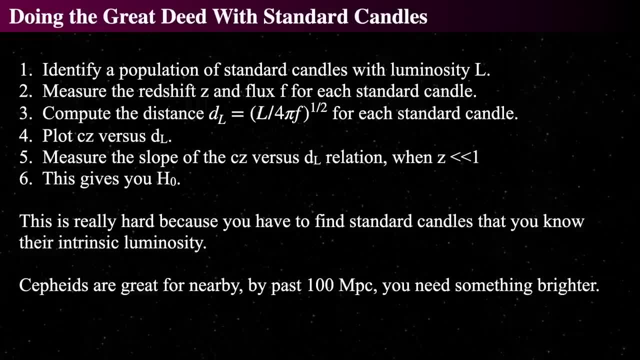 That's how Hubble did this with the Cepheid variables And that gets you out to about a hundred megaparsecs To get farther than that. to see deviations from a straight line, the plot CZ versus DL, it won't be straight, or it's not necessarily straight. 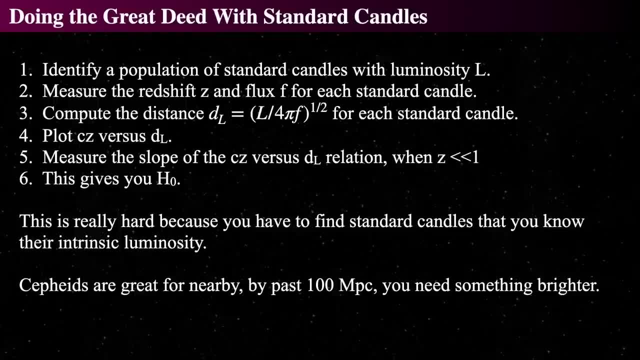 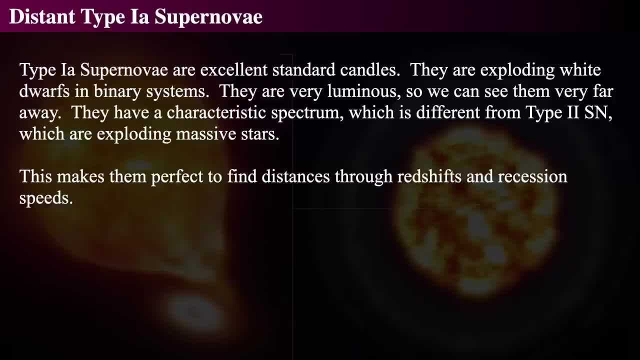 Once you get farther than a hundred megaparsecs. Okay, So let's see if we can find it and let's use a particularly bright object called a type one, a supernovae. And we know that these type one supernovae are good standard candles because they always 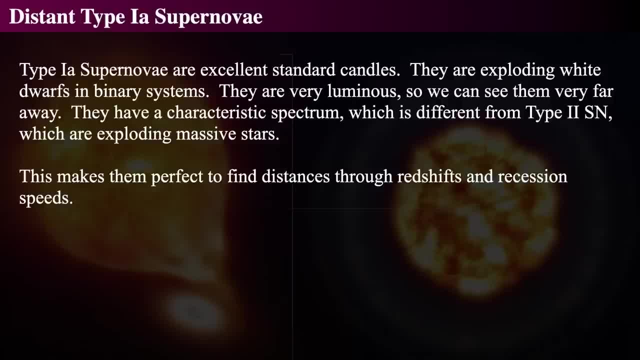 these supernovae, these white dwarfs, explode when they reach their Chandrasekhar limit. They explode when they get 10 molecule, 10 atoms too many. So they're extraordinarily luminous and therefore we can see them from when they're really. 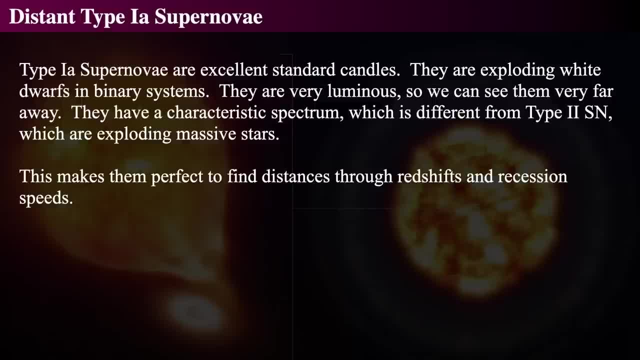 really far away. They have a specific kind of spectrum and they're different from type two supernovae and they also have a different light curve so that we can distinguish them, So you can distinguish a type one from a type two. However, it's also expected that binary stars would actually be more common than supermassive. 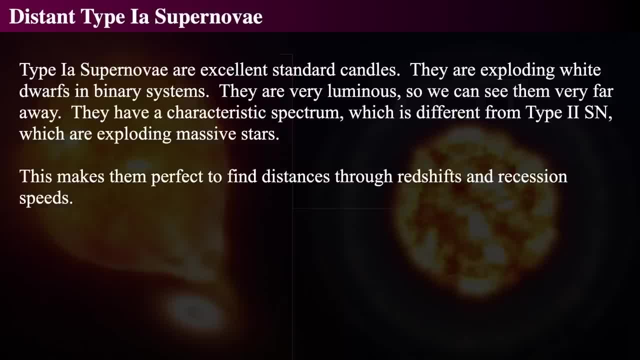 stars. So an extraordinarily bright type two supernova should be less common in general than a type one A. Why? Because, remember, 60% of the stars in the sky are supermassive stars. Why? Because, remember, 60% of the stars in the sky are supermassive stars. 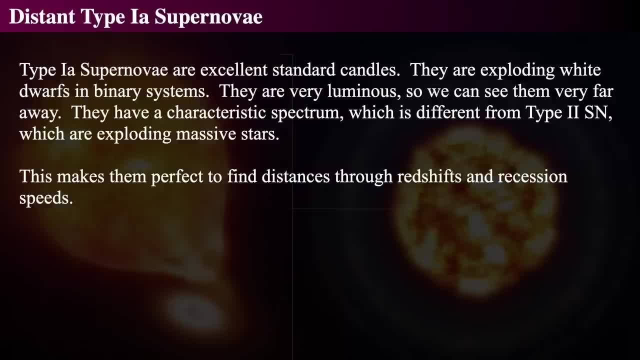 Why? Because they're binaries and a significant fraction of them are spectroscopic binaries And, as we saw way early in the course, is that binaries are really common, but supermassive stars are not. So a star that would become a white dwarf is common. 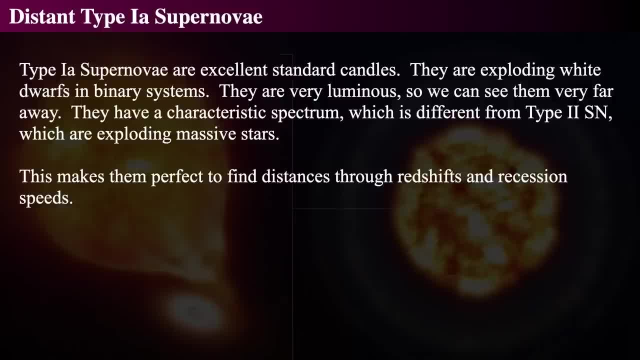 A star that will become a neutron star is not. So you can have a binary star pair: One of them becomes a white dwarf and then the other one dumps stuff onto it, So you should in general, expect to see if it's a supernova. 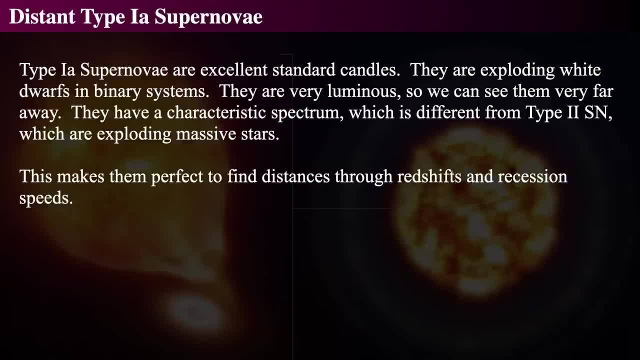 It's more light, It's more likely than not to be a type one, A supernova. So even if you make the mistake, it's still a pretty good mistake to make, All right. So this was a big search. This was an enormous, enormous undertaking. 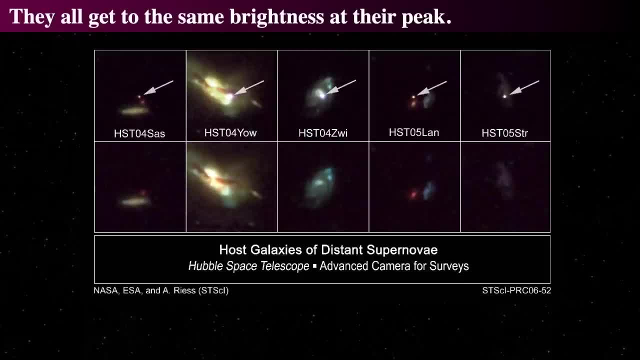 And because here's some images. This was taken by Ries et al with his process using the Hubble Space Telescope, as well as stuff on the ground, But these are Hubble images showing supernovae in distant, distant galaxies and the arrows. 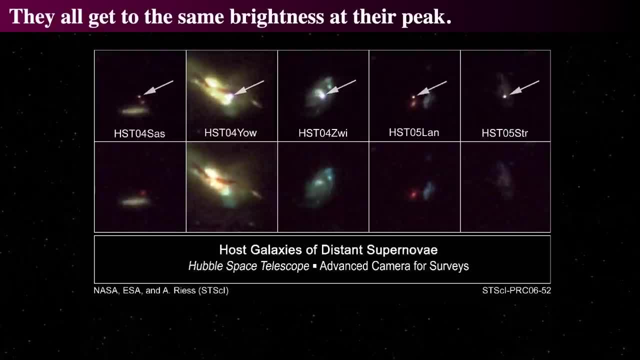 indicate where they are. So there's before and after, So there's befores and afters. where the supernova was discovered? Basically, point a very sensitive telescope at lots of different galaxies in the sky. Make them make a big search, Then go back to see if anything has appeared there that's different, and go back repeatedly. 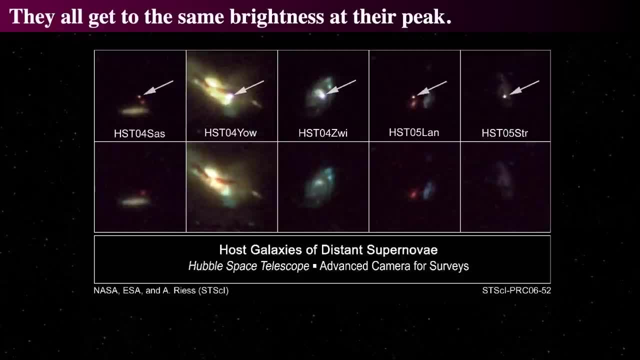 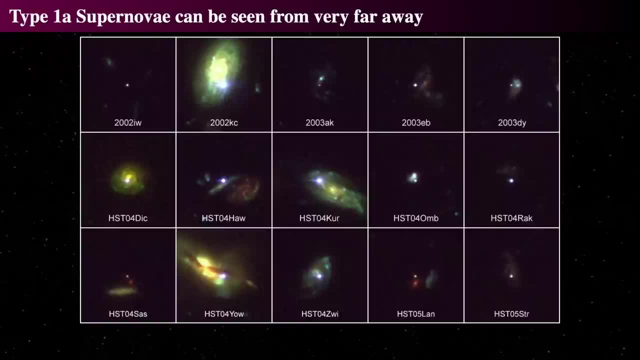 So you're going to go back and forth and back and forth amongst many, many, many galaxies and try to get as many as you can and see if you can find any. Well, the answer is: they did. And here's some more. 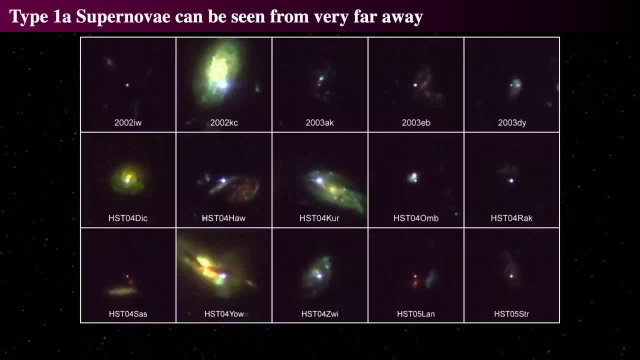 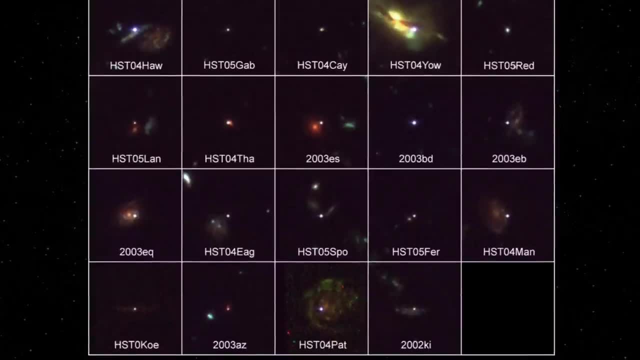 Here's some more ones, Those little dots in the center of each one. Those are some, And then there's more, And there's a bunch of them floating around and there's even more. So there's a lot of these things that we're seeing. 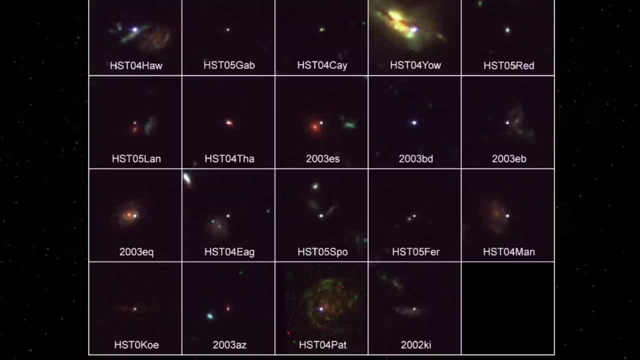 And so the Type Ia supernovae. there's roughly one every you know, thousand years or so in a given galaxy. So all you have to do is go: hunt for enough galaxies. If you look at a thousand galaxies, you should see one. 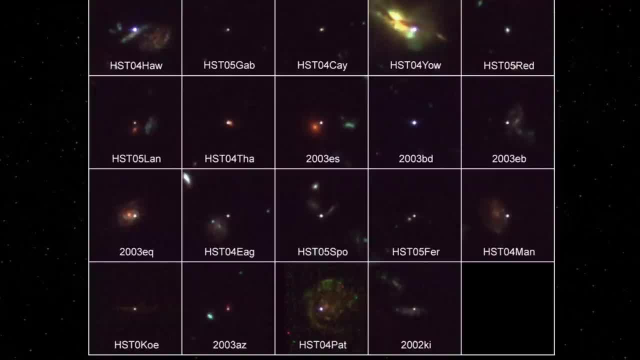 So if you look at 10,000 galaxies, you should see 10.. That's kind of the idea. So now we actually ask the question: Are they really the same? Are all these exactly the same thing? Because if they're not the same thing, then they're not a standard candle and we can't. 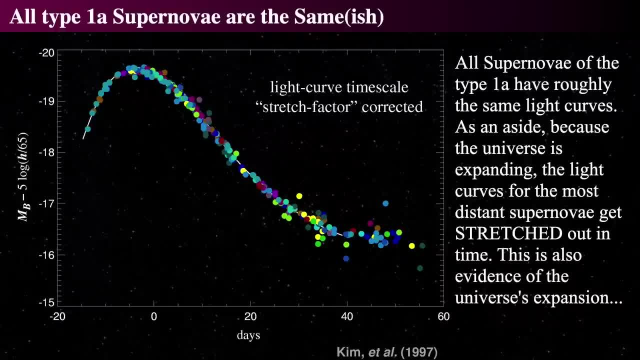 do that. So what we do is we say: let's look at the light curves for all of these standard candles, And each of the colored dots indicates a time that they were looked at and when they were caught at their brightness. So brightness is up and down and time is left and right, with time progressing from left. 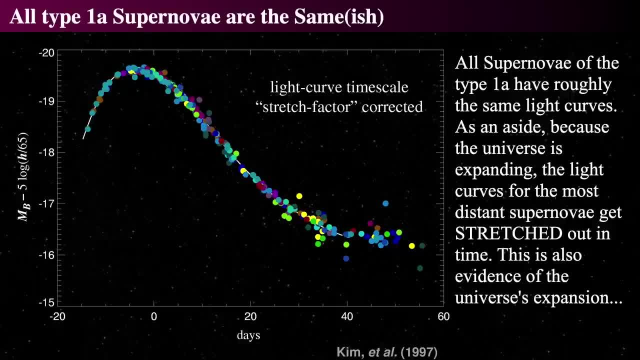 to right and brightness going up and down. Right, it's the same color, it's the same supernova. so you can see that there's many different colors. they all follow the same curve. since they all follow the same curve, they must be the same kind. 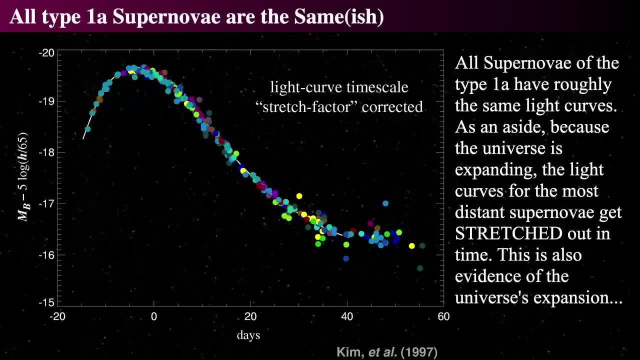 of object. now i do mention something about a stress stretch factor here, and that's because the time gets stretched too. remember there's the that redshift stretches times too, because it's stretching the frequency as well as the wavelength of the light, so it'll stretch the length of the 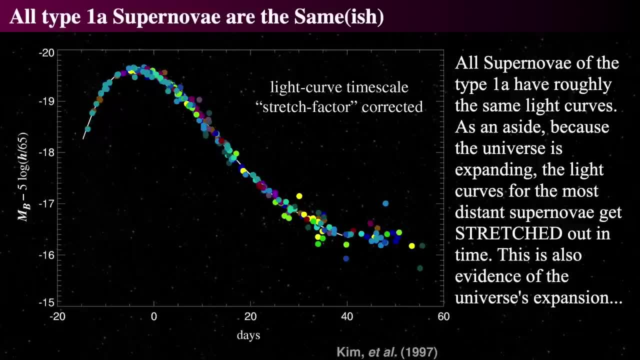 curve, but once you take that into account, they're all the same. so type 1a supernovae- this is. this curve showing a plot of the type 1a supernovae over a large group definitely tells us that, yes, we're actually on to something by saying these actually are standard candles, so let's keep going. 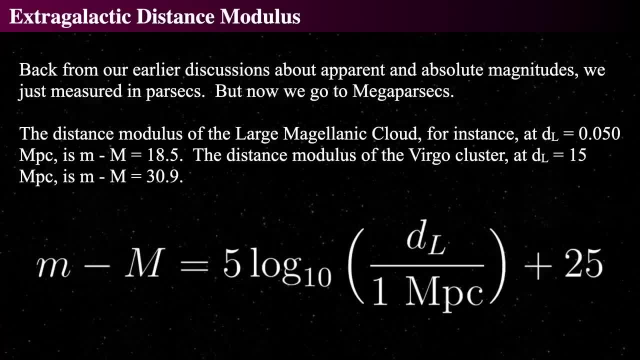 so here's what you can do. let's go all the way back to our first first first thing. we talked about brightnesses and distances and things. remember these? this is called the distance modulus equation. so we're digging this way up from way back. in the first section, we talked about distances and and magnitudes. 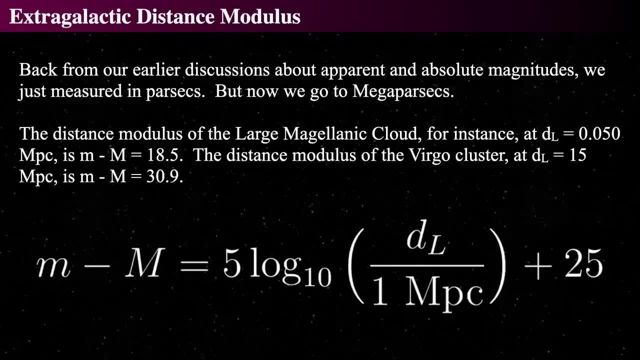 so the first things on the left hand side are the apparent magnitude and the absolute magnitude, and then there's the logarithm base 10, and there's the distance, the luminosity distance to the object in megaparsecs. now we're not just doing parsecs, we're doing in megaparsecs, because we're doing in. 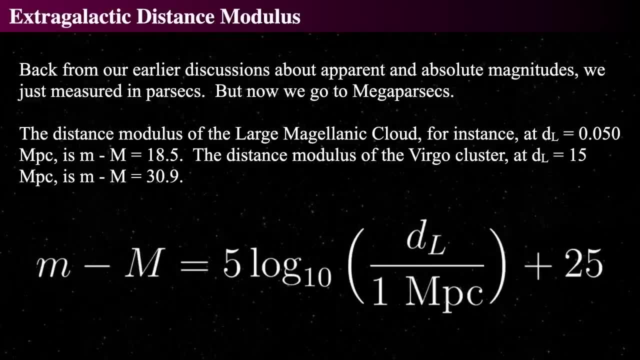 megaparsecs, we instead of adding 5, we add 25.. so we then get a distance modulus which is m minus m, and then we can say that distance modulus is the thing that we care about, and because the capital m is the absolute luminosity or absolute magnitude, that's going to be our thing, that we say: oh, this. 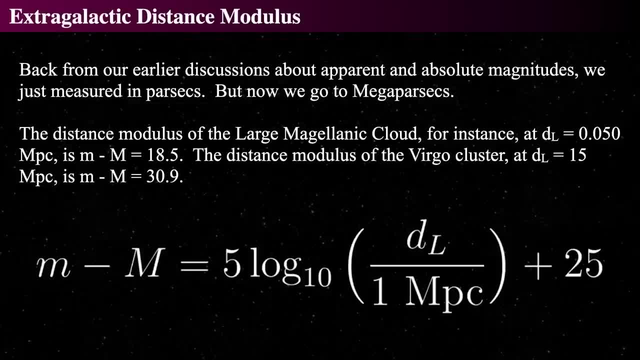 is what the absolute magnitude is, and we can say what's the apparent magnitude. so m minus m gives us the and, knowing the luminosity distance based on the redshift, we can get a lot of information. for example, though, we can say what's the distance modulus to the large magellanic cloud is about 18. 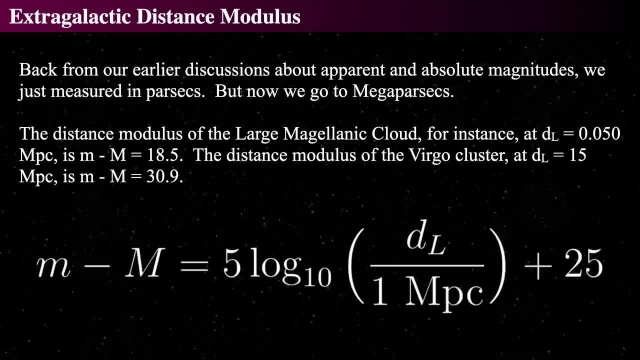 and a half modulus to the virgo cluster, since it's 15 megaparsecs, that's distance modulus is 30.9. so clearly, the farther things are, the larger the distance modulus number is. so we can get a whole bunch of distance moduli for things at different distances. so the distance modulus is then only. 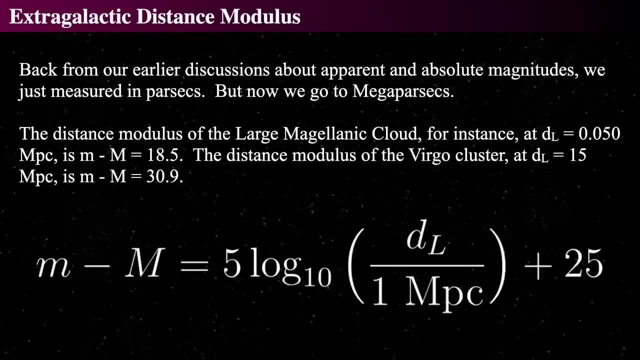 dependent on the absolute, on the apparent magnitude, right? so if you measure the apparent magnitude and you know what the distance is based on, the by that we can get the absolute. we know. we know that we can. we can curl everything around to make sure we got the right thing. but that's not a hundred percent because we're not measuring distances. 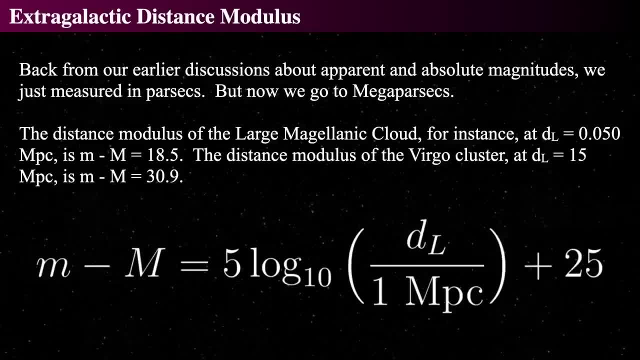 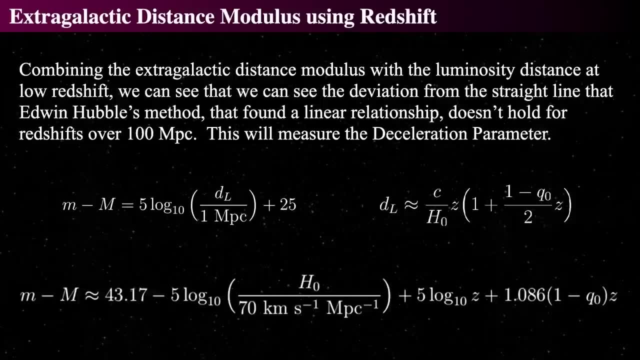 we're measuring redshifts, right, we're associating redshift with distance. we're trying to at least. so let's see how we can do that. so we measure brightness and we measure redshift and we posit the idea of absolute luminosity. so we're going to combine this extra galactic. 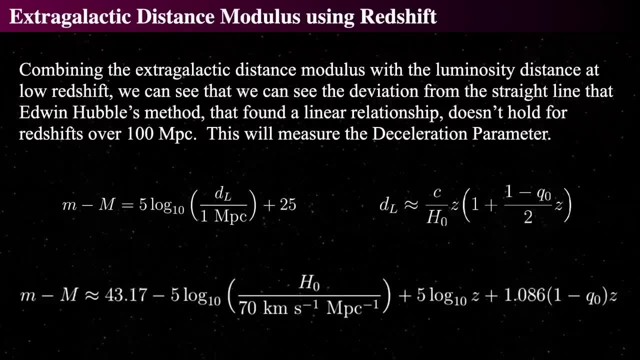 distance modulus equation, not just the normal distance one, but for extra galactic distances on megaparsecs or more, and then we can plug that distance modulus equation, or the specifically the d sub l, which is the luminosity distance, into this pro equation. just combine these two things. 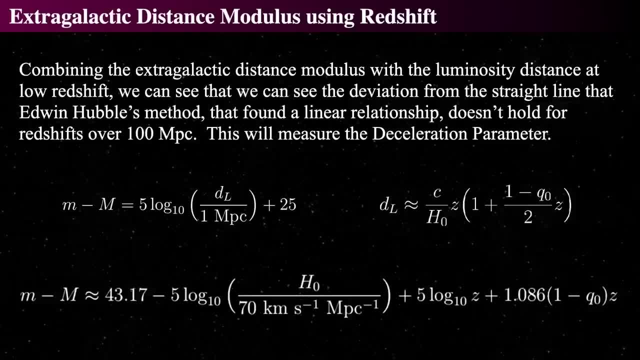 plug the dl into the equation above and make some approximations and yadda, yadda, yadda, and then what we get is that we find that the distance modulus equation with respect to the distance modulus equation with respect to redshift as opposed to d sub l, is rather simple. we have for that. well it. 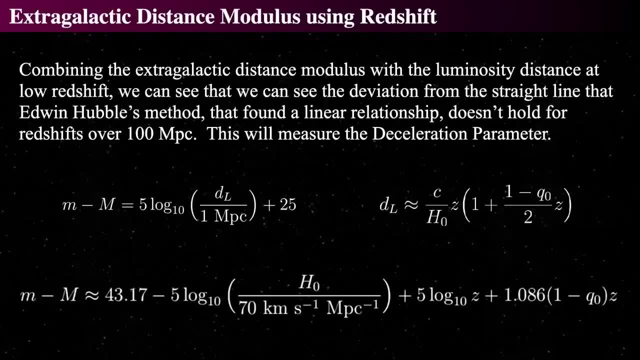 looks kind of complicated but it's a sum of terms and we have the hubble parameter in there, we have the deceleration parameter in there, there's our q naught and our h naught. we try to get a handle on the m, the capital m, which is the absolute luminosity, and we measure the apparent magnitude. 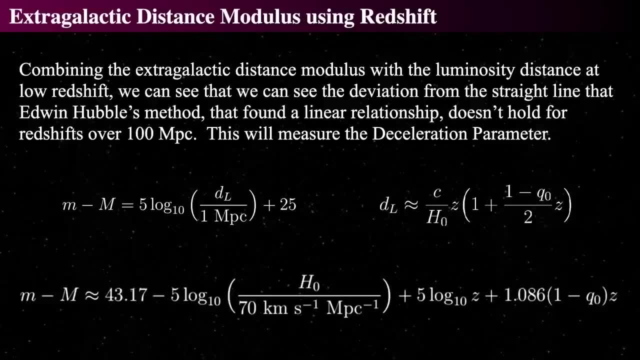 which is little m. so if we know the absolute luminosity capital, m, and we can measure the redshift, we can measure little m and measure z and do this a whole for a huge number of things. it's basically a linear plot. notice this looks linear in, or logarithmically linear in, the in the redshift. 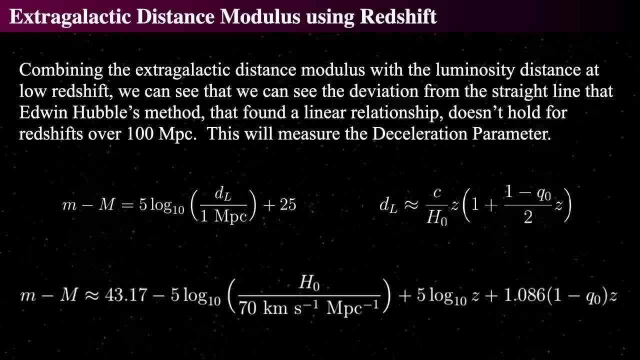 notice. there's a log base 10 of the z, and then there's a, there is also a, there's also a. just a linear relationship with respect to z as well. that's dependent on the deceleration parameter. so if you have enough stuff, you can. 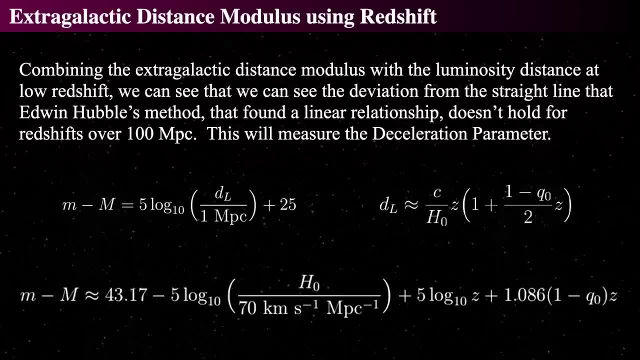 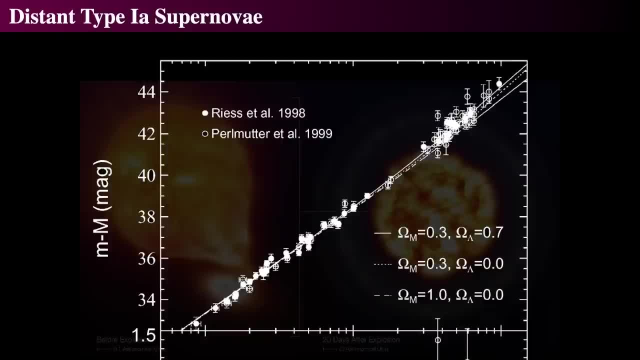 make a line and see what numbers for h naught and q naught fit. that's all you do and that's what was done. so here is the plot from reese et al and uh, adam reese and his team with the high, super high z supernova search team in 1998, as well as saul perlmutter and his team. 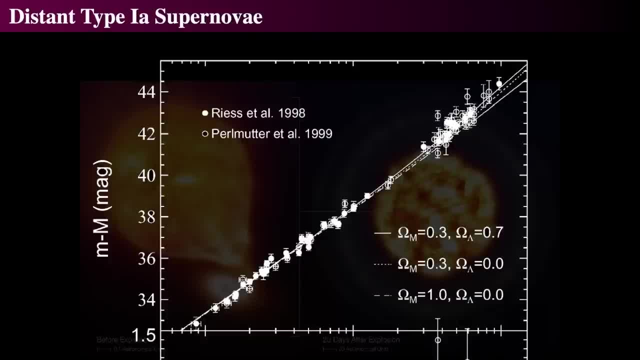 with the supernova cosmology project. in 1999 these two things were were published together and this distance modulus of redshift for these objects for extraordinarily high redshift out to about one on the right hand side is almost a redshift of one, and what we're looking at here is that there's three lines going. 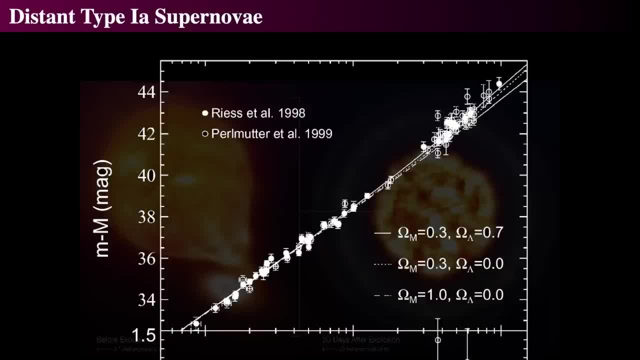 through the graph, and one of them is the critical mass density. remember we related the deceleration parameter to the content of the universe. we could have put that in there too. so we just went to deceleration parameter, just did that. but if we then say, what's the best fit, deceleration parameter. 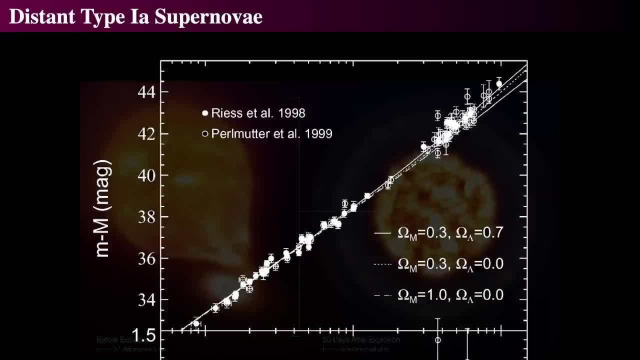 to this stuff. it's kind of hard to tell from this graph, but let's say we remove or normalize it to what we thought we knew because, remember, the expected amount was about 30. so the middle thing, with the triple dots, 0.3 and no dark, no cosmological constant, which is lambda, omega, sub lambda, there's. 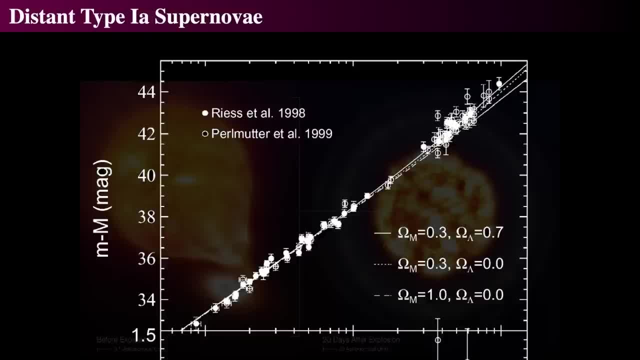 no energy constant contribution from that and the matter contribution omega sub m is about 30 percent of the critical density. that's the thing that everybody thought from the 1950s through the 1990s. so getting the exact value of the deceleration parameter is tricky and, as you can see, it's very tricky from. 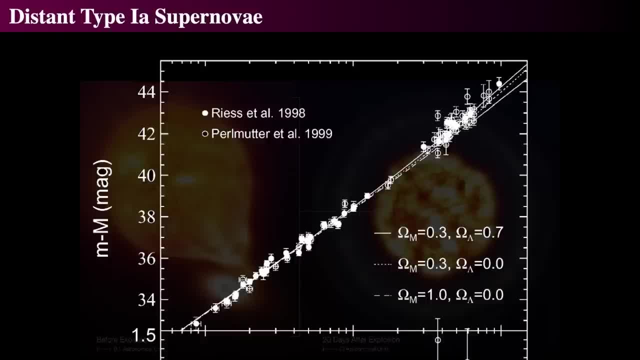 this because each of these dots is a data point and the and the little bars up and down from it, those are the error bars associated with it. but let's normalize this to the look when we just say: let's see, let's just go around the 0.3, so let's actually 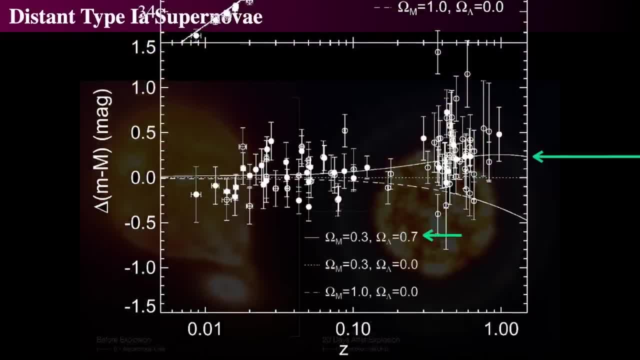 take a slightly different view of it. and the dotted line again is the mat, is the critical dent, is the total matter density compared to the critical density which is 0.3. and that's the dotted line going across the middle, the, the flat universe, with critic, with mass. what made a flat universe is the. 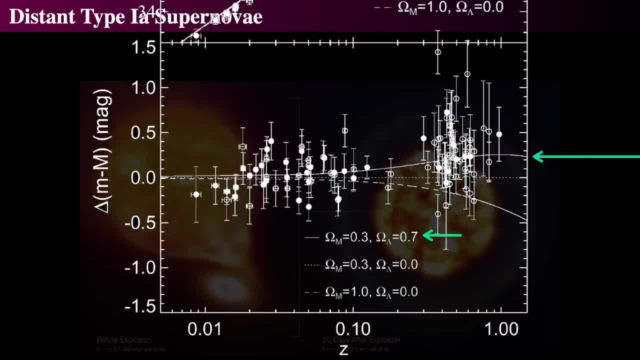 sol is the is the deep dash line going that arcs to the bottom. notice it kind of goes across and across and arcs down at the bottom. So it's the one that meets the right-hand side really low, the one I have not indicated with a green arrow. The best fit for the data that they have is one where we have a flat universe. 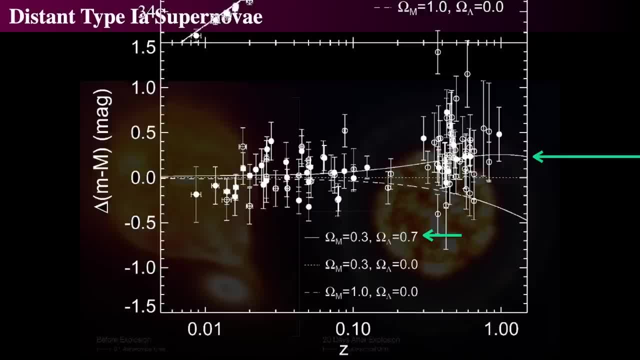 and that the omega sub lambda is 0.7.. So the best possible fit to all that data. you know it kind of looks scraggly but it certainly isn't. There has to be something there that's different than matter. That's kind of scary. So their best fit to the data. and this is the data. 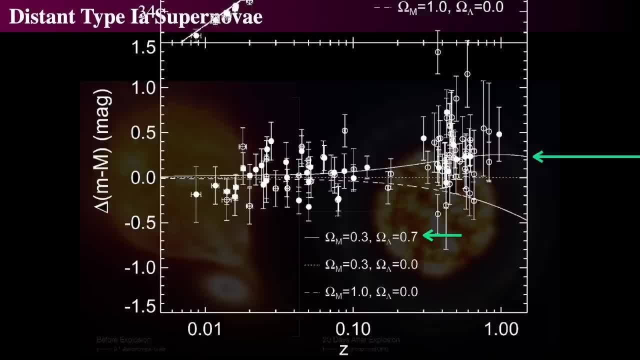 from the 1999 and 2000 papers and so forth in 98, this is the discovery papers- where they said the best fit includes an energy density of 70% of the critical density for the cosmological constant. And this is the data that they showed. So what about a cosmological constant? Let's go. 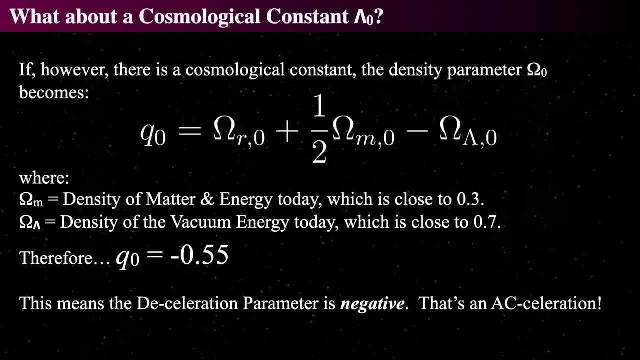 back to that equation that we have. where we demonstrate it, We find: oh okay, what do we get? Well, what does that mean? It says that if the matter and energy density is close to 0.3 and the density of the 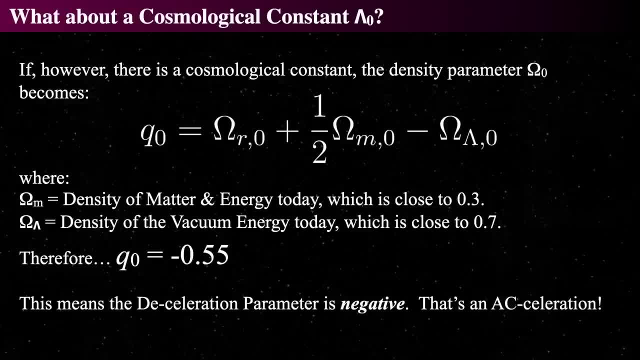 vacuum energy or the cosmological constant is 0.7, then the deceleration parameter is negative, 0.55.. A negative deceleration parameter is an acceleration. That's an acceleration because it was defined in terms of deceleration. So a positive Q naught is a deceleration and a 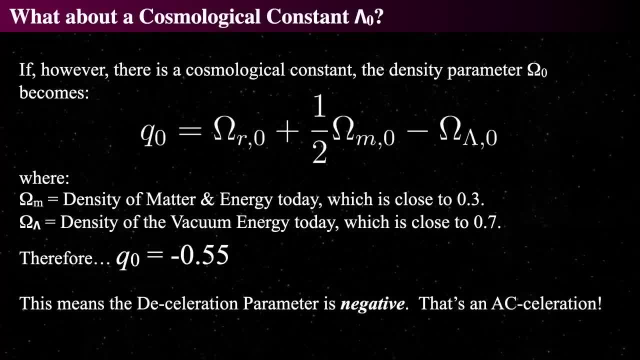 negative Q naught is an acceleration. So the best fit to the data was one where there was where there deceleration is an acceleration. Now, this is important because there are a lot of different ways that the deceleration parameter could have been measured. There's lots of different. 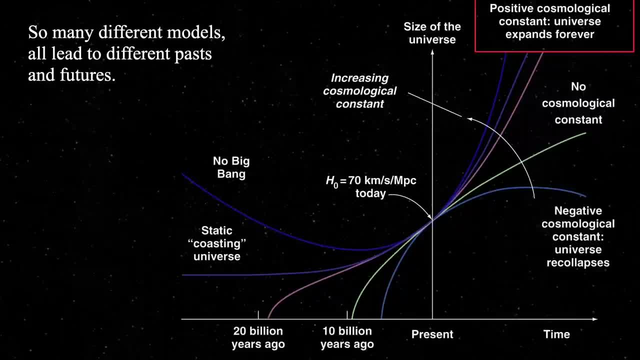 possibilities for the, for how the universe can go in the future and how it can go in the past. but only measuring it can get you there. There are some toy universes- and we call them toys because they don't really happen. where we have a negative cosmological constant, it re-collapses. 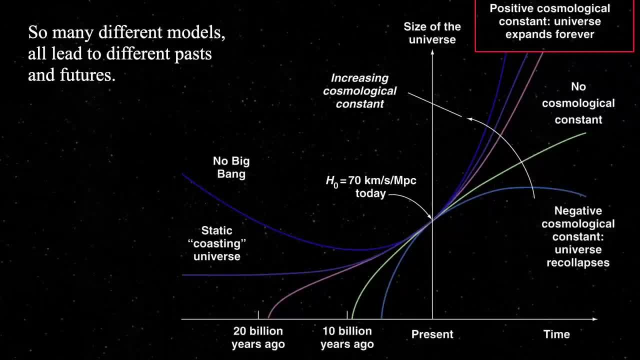 or maybe there was no big bang and it just went down to a minimum size and came. well, like it started, big, collapsed down to a minimum size and re-expanded, so there just didn't get to zero size. Or maybe it was: it had a big bang really long ago and it didn't do anything for a 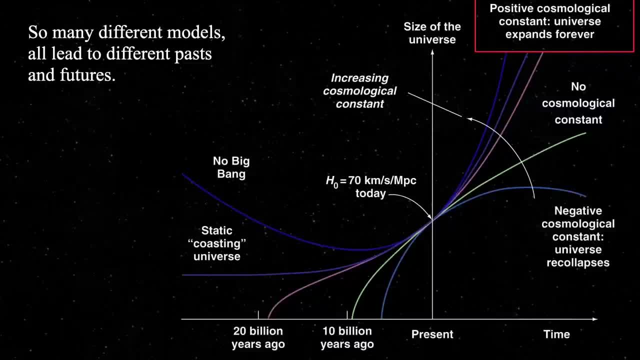 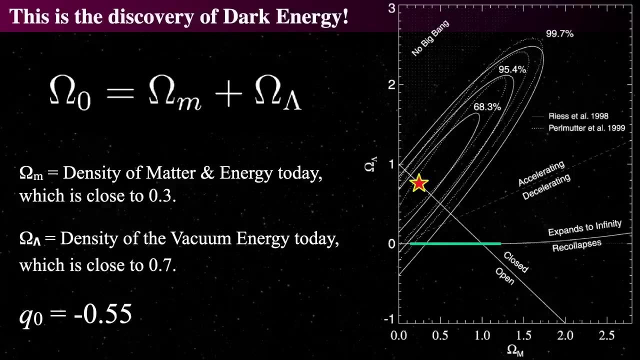 very, very, very long time and it coasted, then expanded. and maybe there's no cosmological constant and so forth. But what the measurements are showing is that there is a positive cosmological constant which makes the universe expand forever and accelerate. So that is the discovery of dark. 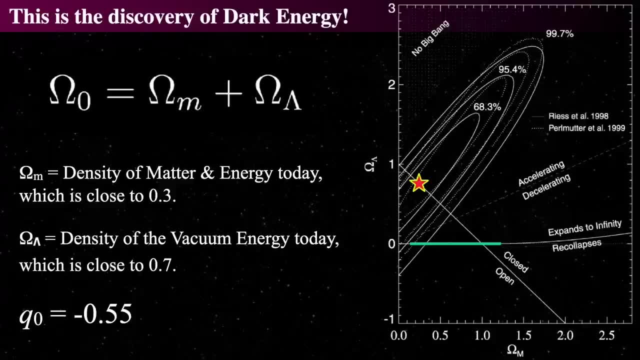 energy, And so they're best fit to the data. and that's what those arcing curves are all about. Remember how the data points were there. They tried to do their best statistical study to say what is the highest likelihood, And the and Rees and Perlmutter were competing teams. 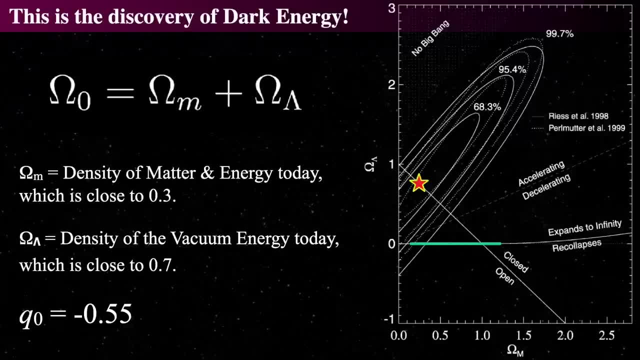 Perlmutter's team was called the Supernova Cosmology Project and Rees's team was called is called the Hi-Z Supernova Project And their values are overlap quite well And the whole idea that I dealt with when I was in college is on the green line, where there is no 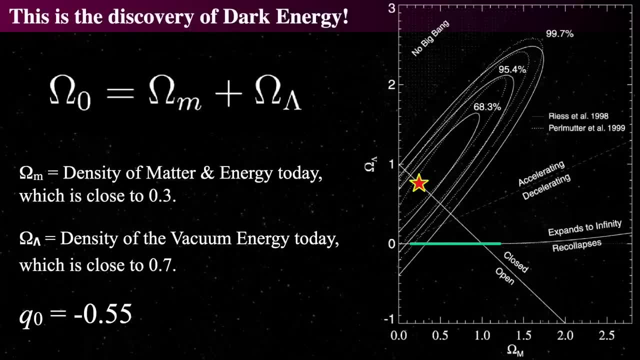 cosmological constant, And so we would all it would be in the decelerating universe parameter space. See how that decelerating is below the dot dot dot and the accelerating is above the dot dot dot. So if there is a positive cosmological constant and it is larger than zero, then the 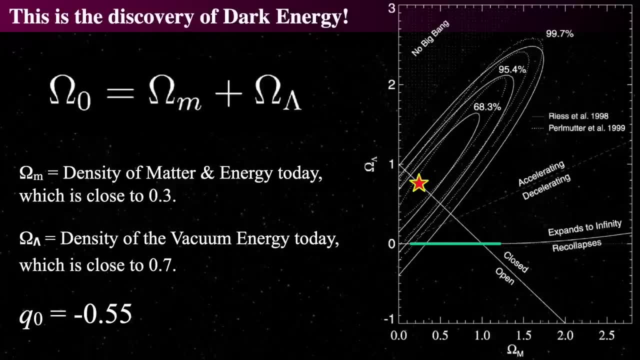 universe will likely accelerate. I mean, if it's not too big and there's a lot more matter than it could still have, could decelerate eventually. But the funny thing is is it lies right on that. their measurement lies right on the flat universe line which is between closed and open. but it 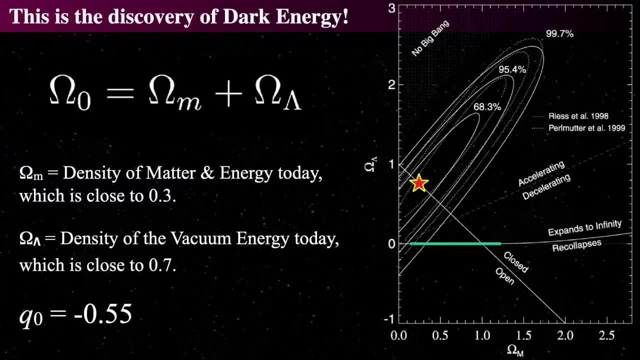 definitely lies above the accelerating thing. So we find that it's definitely not a no big bang like a bounce universe. It's definitely because that's way up high So you have to have a huge cosmological constant which is not seen in the measurements. So that's not. that did not happen. 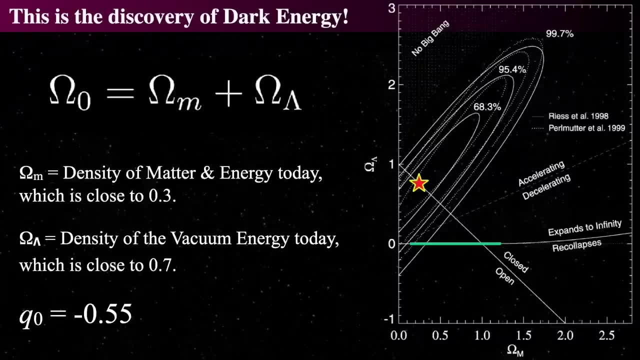 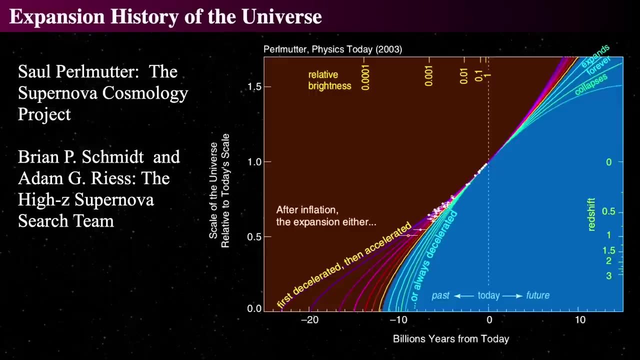 There was some big bang. however, the universe is now has some component that is causing it to expand and expand and expand. The ovals show there's best statistical fit to the data, and that's what that means. So here's something that they wrote up that came out in physics today. 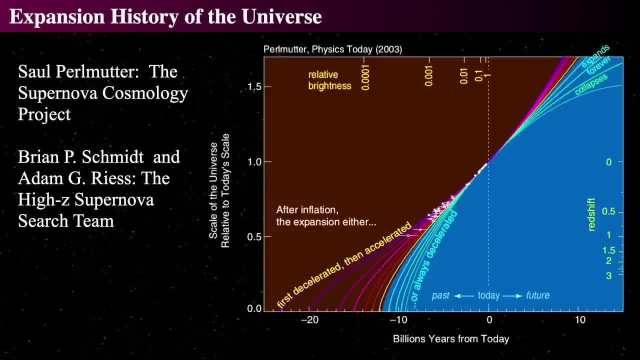 and this is: this shows more about the nature of when the redshifts were dot and where their dots are, And you can see that the higher the redshift, the farther back it goes And looking at that, we can see that. 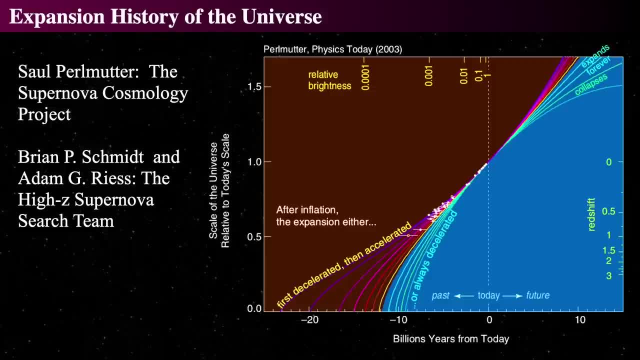 the universe had first decelerated, then accelerated, or basically has been accelerating since about 5 billion years ago. It's definitely in the expanding forever category as we look in the farther and farther past, and it also is definitely in the farther ago. So, really, when 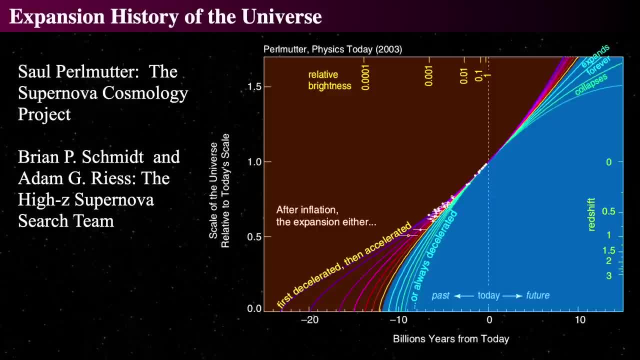 you look at the distance modules, all it said was that the things were dimmer than they should have been. The supernovae were dimmer than they should have been, so that meant they're farther away now than expected, so the universe must be accelerating. That's basically what was found with the distance. 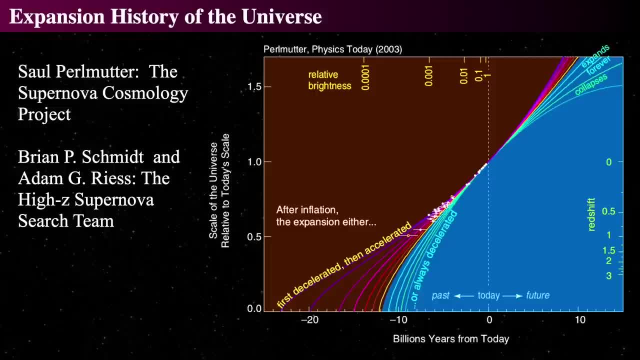 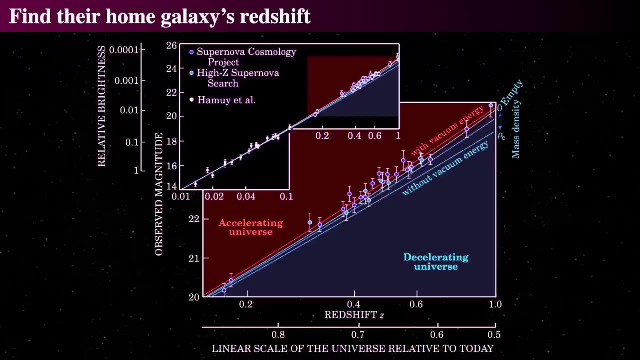 modules. They were fainter. At a given redshift they were fainter and the farther the bigger the redshift the fainter they were than is expected. That's what that means. So if we found their galaxy's redshift in there, we could discover that, basically that the universe has some sort of vacuum. 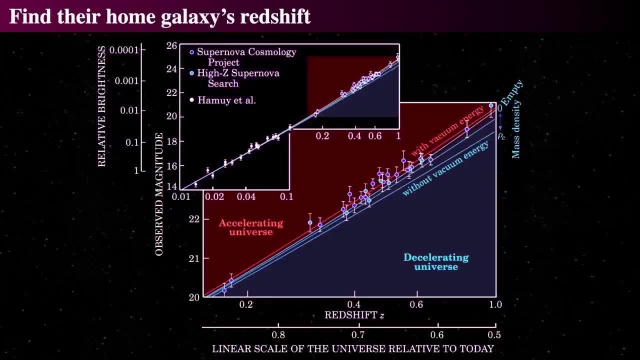 energy in its life and that's what we're looking for. So if we found their galaxy's redshift in there, we could know that that's what they're likely accelerating and that's what was found by Perlmutter and Schmidt and Reese. So Brian Schmidt and Adam Reese were the supernovae. I'm 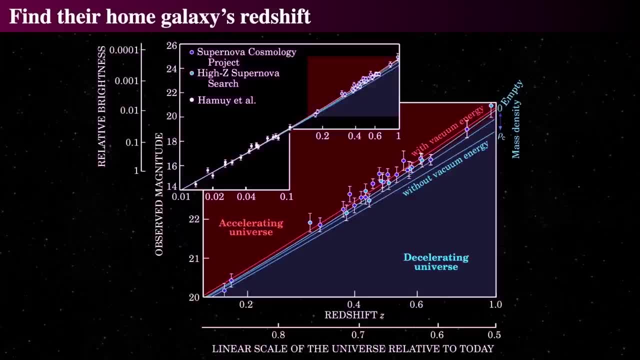 sorry I kept omitting Brian Schmidt from it, but Schmidt and Reese were the supernovae team Heise Supernova Research Team and Saul Perlmutter led the Supernova Cosmology Project. All right, so the next thing we see is: here's from the Supernova Cosmology Project's data. 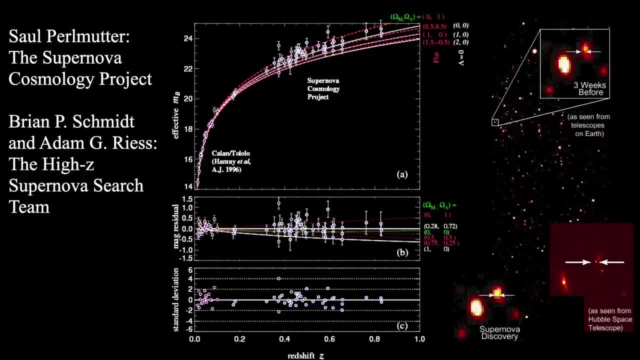 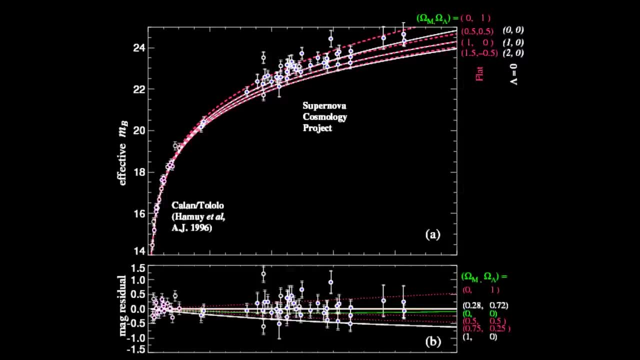 themselves and, zooming in a bit, I have a slightly different view of that, and we see supernova cosmology product only from their material. they say that it's about 0.28 and 0.72. no matter what, both teams agree that there must be something like 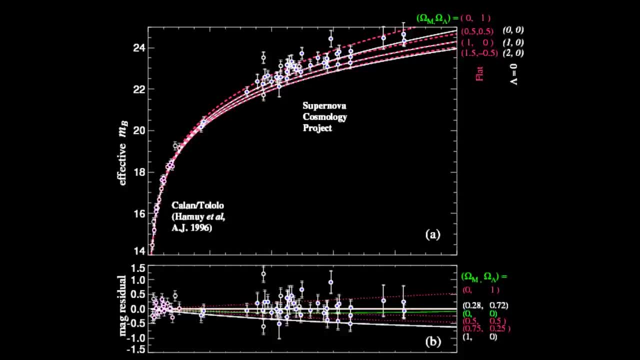 that, and there's a very interesting story that you can find if you go hunting around about the nature of how this was discovered. basically, there was an illicit email that caused quite a kerfuffle between team members who communicated to each other without going through the highest-end people, so 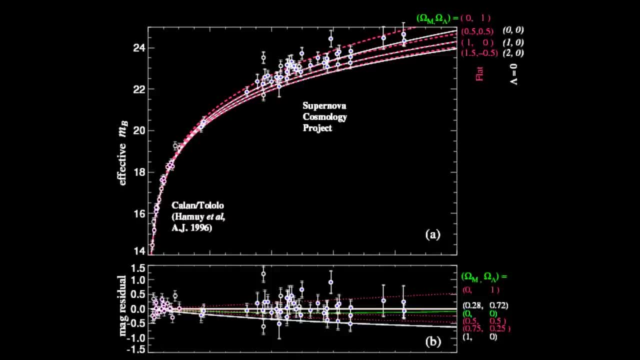 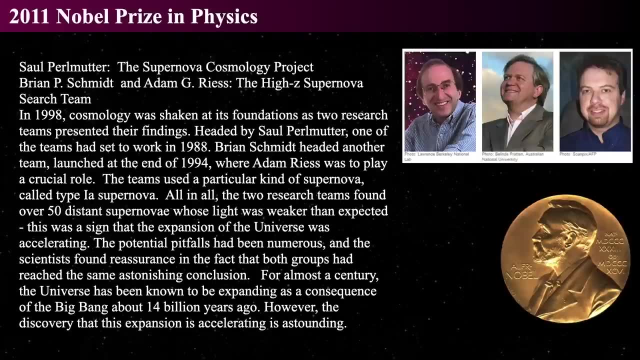 basically they- one person tipped the other's hand, they were competing to get this information- and they basically tipped each other's hand and, as a result of it, both teams got the Nobel Prize as opposed to only one. so if one guy, or a few guys, had kept their mouth shut, then likely only one of these teams would. 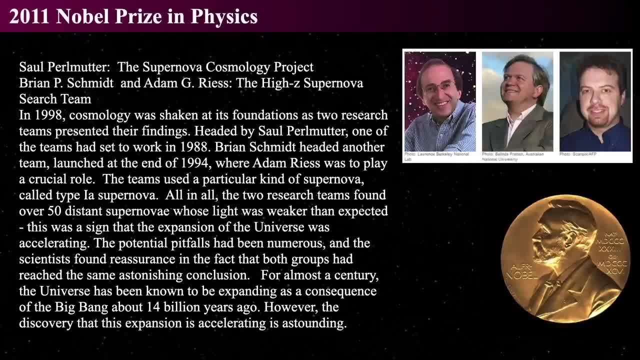 have gotten it, because they would have announced it first. in any event, because they essentially jointly announced it, they jointly won the Nobel Prize in 2011 for decision-making. so, now that you know, you can get a lot more information and you're just discovering a lot more information and you're just exploring the acceleration of. 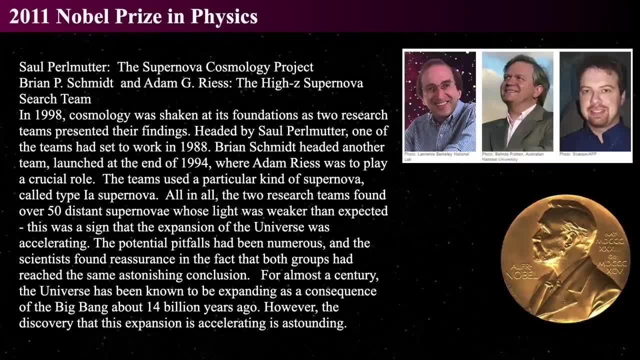 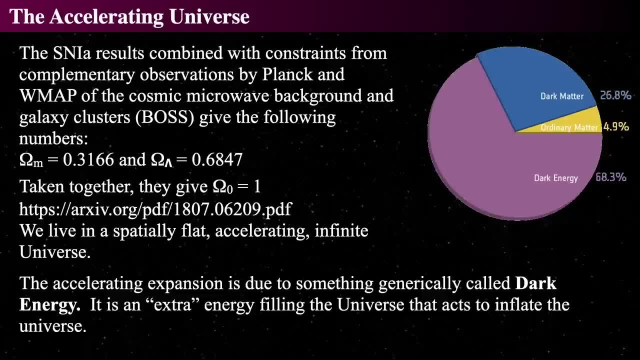 the expansion of the universe and opening the window into the new physics of understanding what the heck this dark energy stuff was. so that's not just from supernovae. in fact, the supernovae results combined with other things: constraints by the cosmic microwave, background emissions such as Planck. 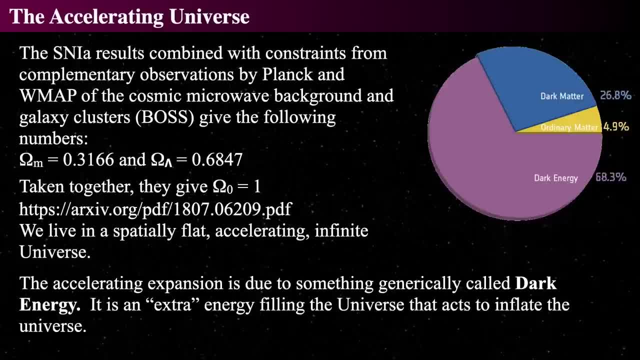 and wmap that look at the cosmic microwave background clusters like BOSS give and specifically later and much more accurate, much more, much more precise results of being about point zero, thirty two percent or a point three, one, six, six of the critical density for matter. and this has come. 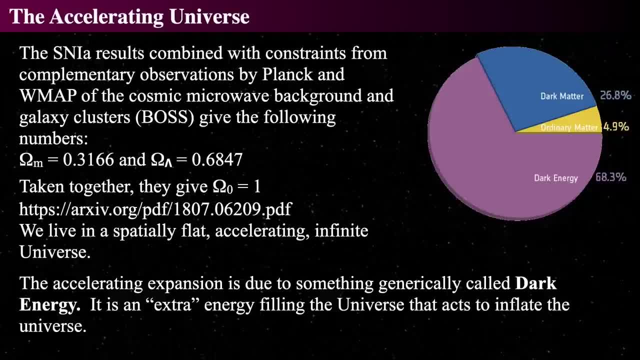 specifically from. this comes specifically from the Cosmolux from from June of 2018, from the Planck team. that's what that archive link is for. is point six, eight, four, seven. so if you add those two up, it's almost exactly one. they give a almost exactly one, which is really nuts. it's almost. it's one plus, or. 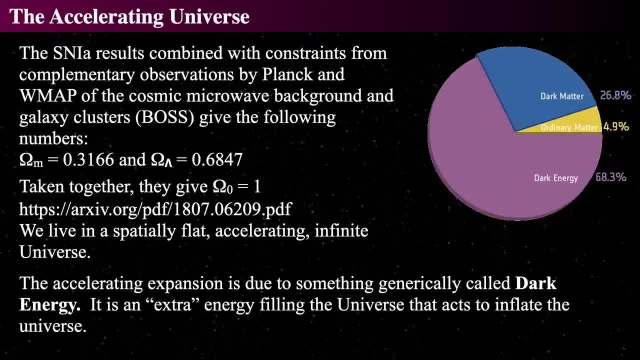 minus. I didn't get the error bars in there, but we add the error bars in there. it's pretty much one. so the cosmological cosmic microwave background studies, as well as galaxy cluster studies, support the idea that was found in this, which is a completely independent concept. looking at the, the background light of the 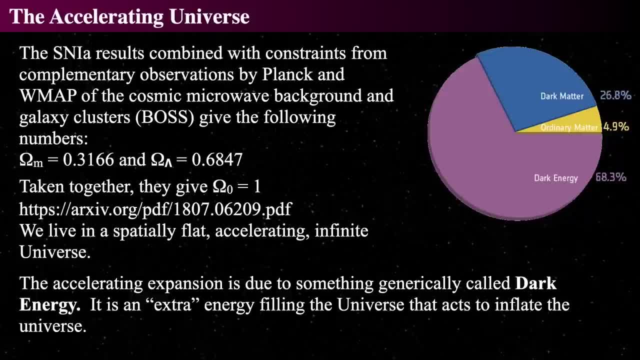 Cosmos. it's very different than studying the other, the cosmic microwave backgrounds does that by looking at the distribution of lumps and bumps inside the cop in there and galaxy clusters. look at how fast galaxy clusters appear to be, how the size and scale of galaxy clusters across the cosmos. so all of these things. 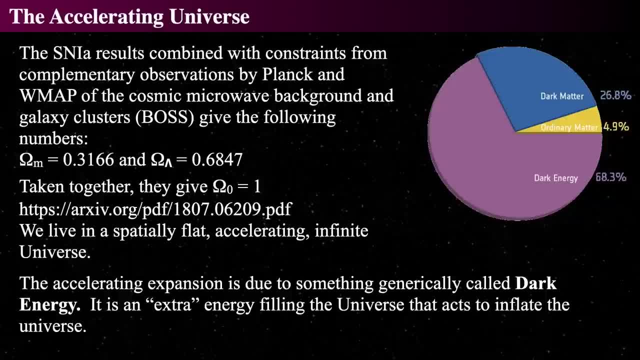 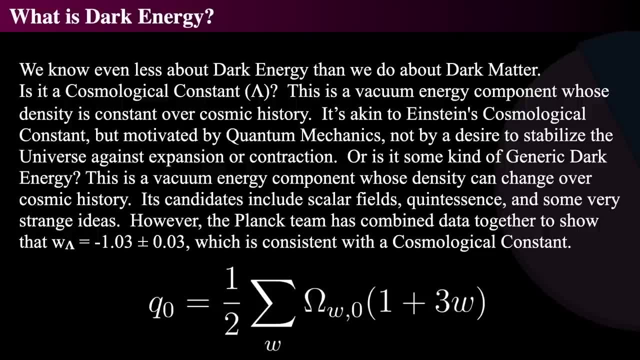 taken together say the same thing: that there is something called dark energy, which nobody knows what the heck it is. nobody knows what dark energy is. nobody knows, nobody who it is. nobody, no one has any freaking clue what it is. no one knows. the simplest concept is: it's probably a cosmological constant, and 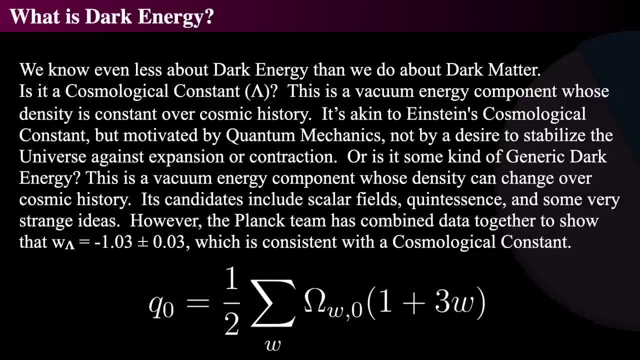 that means it's a w of minus 1, and that cosmological constant would simply mean that there's a vacuum energy component. it means the the very, that the thing that we call space, the thing that we call space-time, has energy associated with just being space-time. that is a constant composed of energy of some kind. but this, once we have such energy, then we swim over thisوي. will it dissapear from our universe by the G 되는? 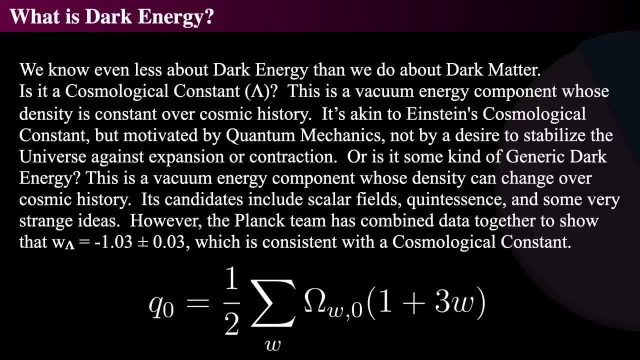 and so there's just so much stuff of energy that is part of it, And that's what a cosmological constant is. So as the universe expands, there's more space. So therefore, since it's constant, it doesn't dilute. 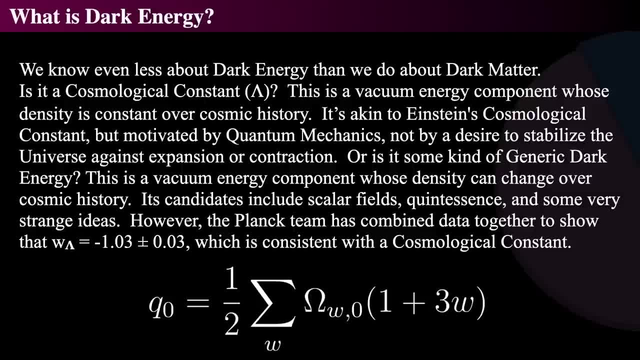 So every box of space has the same amount of cosmological constant. So once you get diluted, once the matter gets diluted, you're only left with cosmological constant. So that's what's happening in the future. It's a very strange thing. 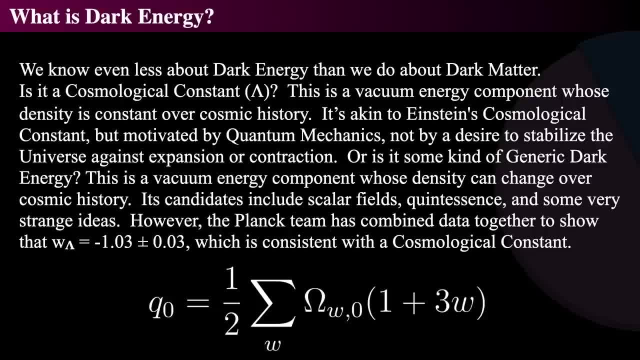 Nobody knows what it is. It could be some other kind of dark energy, though, and people have tried to figure out exactly what the W is for dark energy. What is it exactly, Minus one? Is it a little less than that? Is it a little more than that? 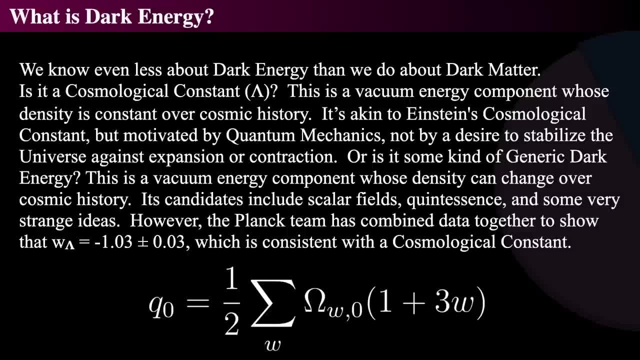 Remember W is not doesn't have to be minus one, It can be something else. So that's another thing that's been checked. There's all sorts of weird things that it can be called that it can maybe the nature of the cosmological constant changes with time. 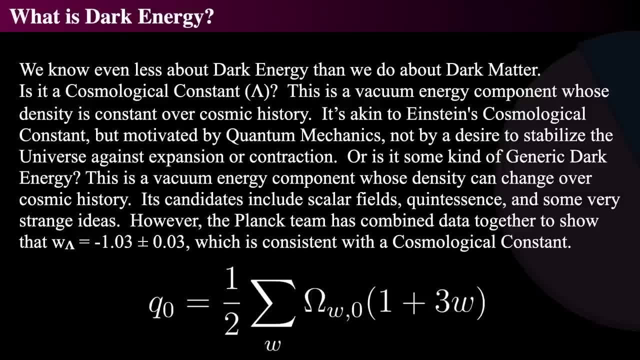 Maybe it's only minus one over here, Maybe it's minus 0.5 over there And maybe it's a whole bunch of things. So you can go out scalar fields or quintessence or lots of different things. A lot of them have to do with it changing with time or being different at different locations in the cosmos. 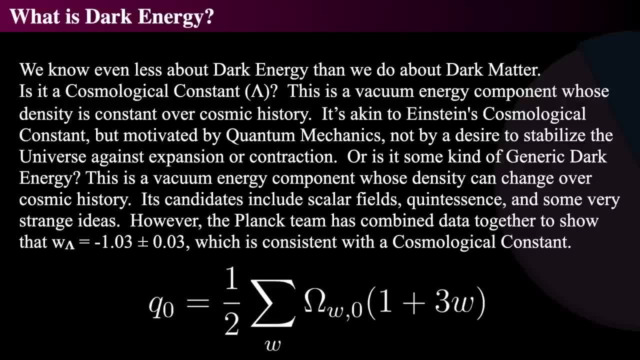 But the Planck team, looking at their data- this comes from the July 2018 paper I referenced- says that they measure that the W or the or what the- basically the equation of state. what the equation of state is for the- for it- is that it's pretty close to minus one over there. 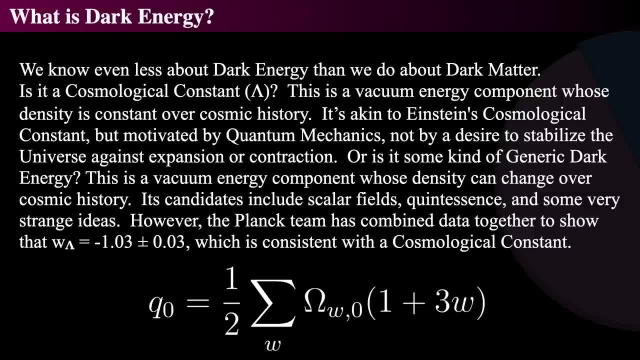 So it's pretty close to minus one And they're hoping. and the other thing is it could be that if it's not minus one, if it's less than minus one, say that's like minus two or something- then we would call it a phantom energy. 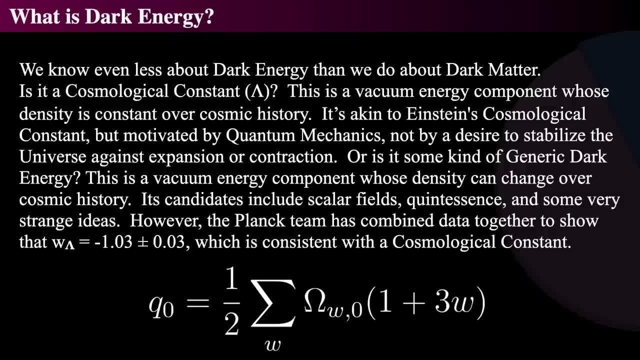 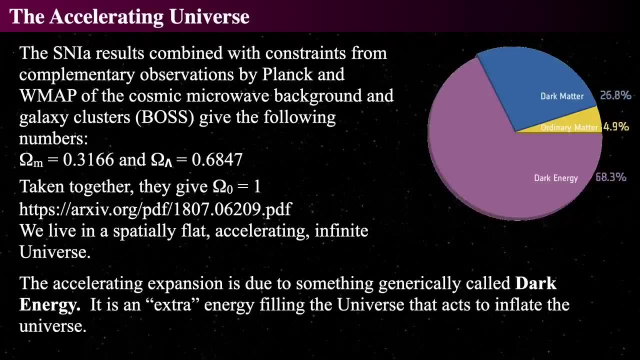 And that's a really weird thing, But right now, the current consensus is that the universe is composed of a minus, a cosmological constant which takes up 70% of the universe's material- 68%- and matter and dark matter composed- 32%. 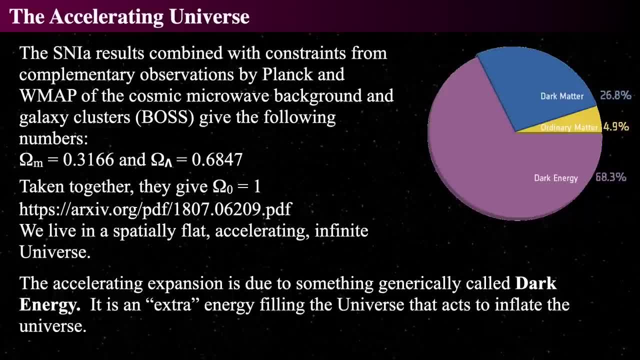 And that the universe is flat. So our universe is geometrically flat. It's not hyperbolic shaped, It's not spherical shaped, It's neither open nor closed. It is flat And it is accelerating. It is a flat, accelerating and infinite universe. 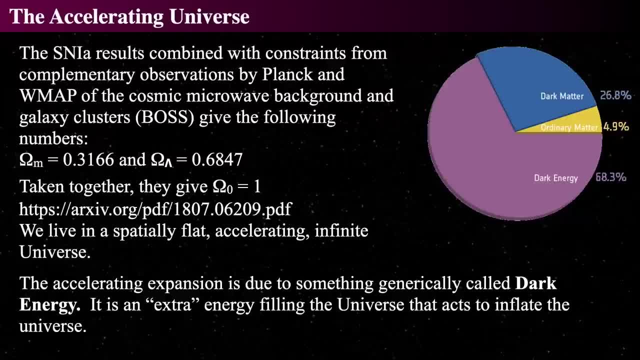 And that's what we live in. And so dark matter composes 26.8, at the current date, 26.8%- of the energy density of the cosmos. Normal Normal matter is about 4.9%, but dark energy composes about 68% of the cosmos's, of the entire universe's energy density. 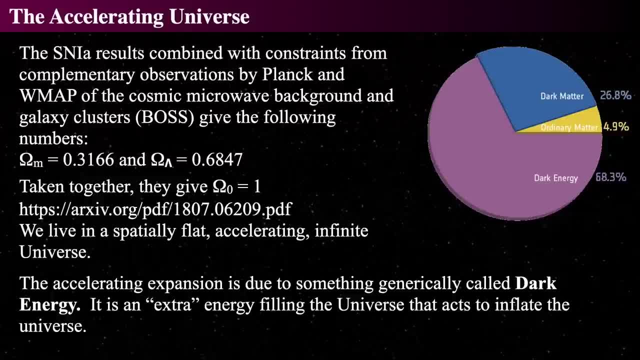 And as the universe expands, dark matter and ordinary matter will be diluted, And so those numbers will drop until dark energy becomes. everything becomes everything. So that's our current energy budget. Only 5% of the universe is ordinary matter, And of that ordinary matter, only 10%. 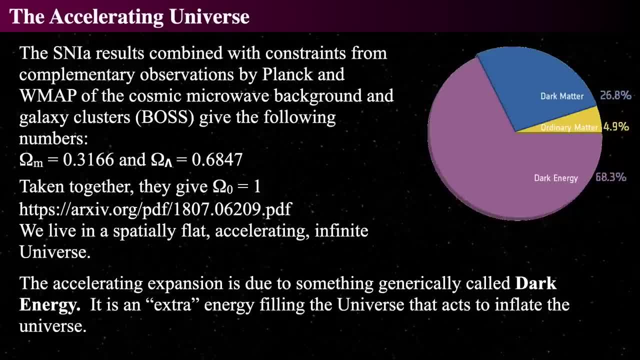 Or 0.4%. Half a percent is stars. So the rest of the ordinary matter is just intergalactic gas, hydrogen gas or basically hydrogen at extreme heat. So ordinary matter is not even planets. Ordinary matter is mostly intergalactic gas. 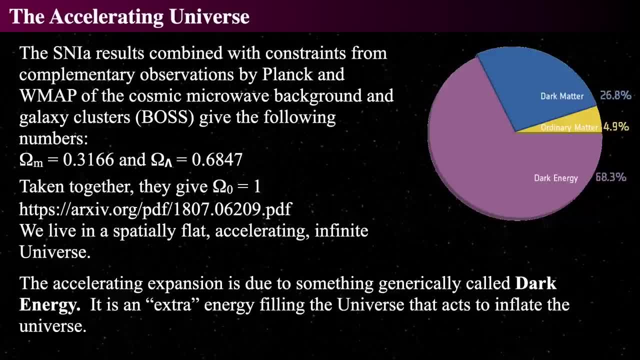 The rest of it is the rest of normal matter, is dark matter that doesn't interact with light in any way, And dark energy. we have no idea what it is. All we know is that it's forcing the universe apart. All we know is that it's forcing the universe apart. 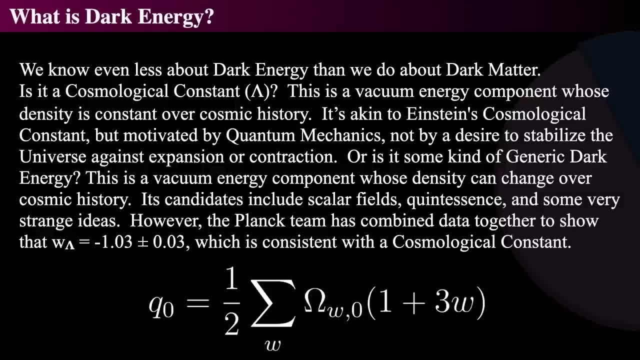 And then forcing it to accelerate in its expansion. All right, So that's where we get the, and so there is what we get from from all these strange things, And really no one knows what dark energy is. It's presumed that you can't actually make a box out of dark energy and you can't box it into anything. 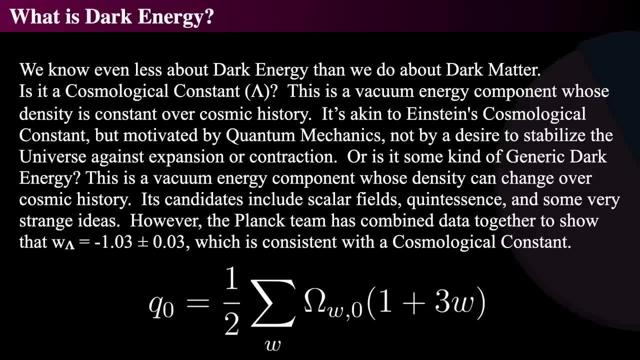 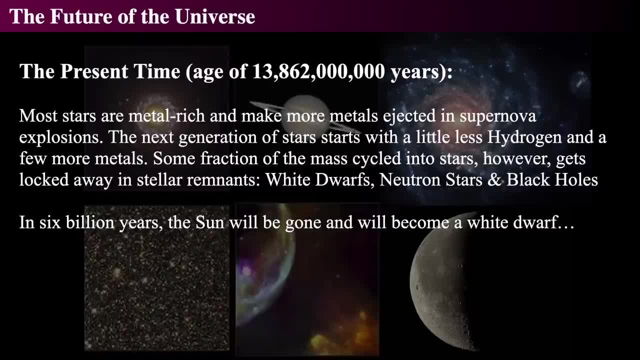 But even though it's everywhere and it's inherent to space-time itself. That leads us to what to say. what's going to happen in the future of the universe? So what will happen So today, in the future of the universe? Because if the universe is going to do that, it's expanding, accelerating. 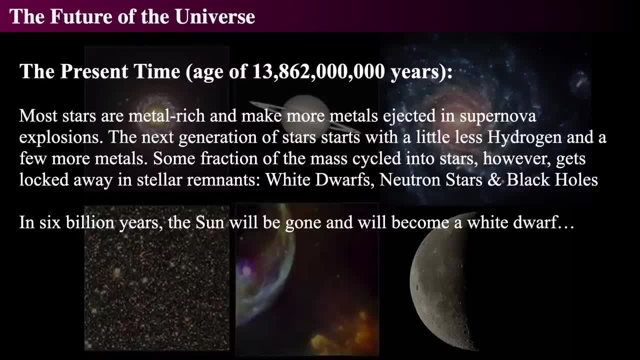 What's going to happen? Well, today there's stars, Stars that are metal rich. More stars explode. If they explode, they make stuff And then that makes there's a little less hydrogen as time goes on. But there's pretty stars and planets and things like that. 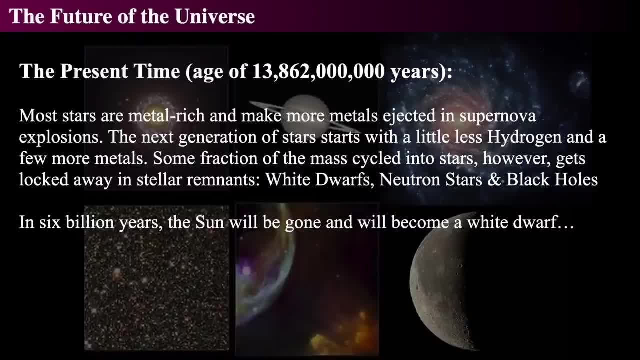 And white dwarfs are made and neutron stars and black holes, But things get locked up in those things. So in about six billion years or so the sun is going to be gone, It'll become a white dwarf And you know that's going to be sad. 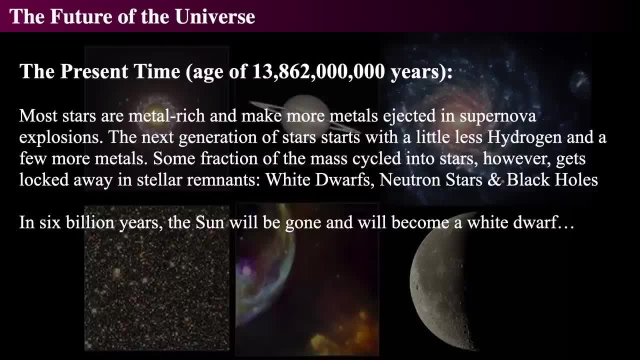 But right now we're calling this the stellariferous era. Stars can be made and born in galaxies, And they can be. multiple generations of stars can be made, And that's the current day, 13.8 billion years after the start of the Big Bang. 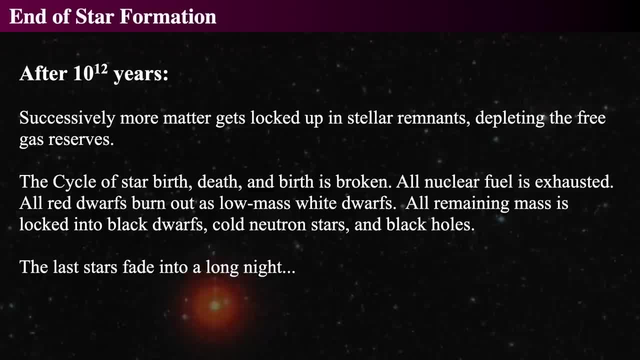 However, in about a trillion years, which is a long time from now, About a thousand times the current age of the universe, Current, a thousand current universe ages from now, The matter will be locked up in white dwarfs and neutron stars and black holes. 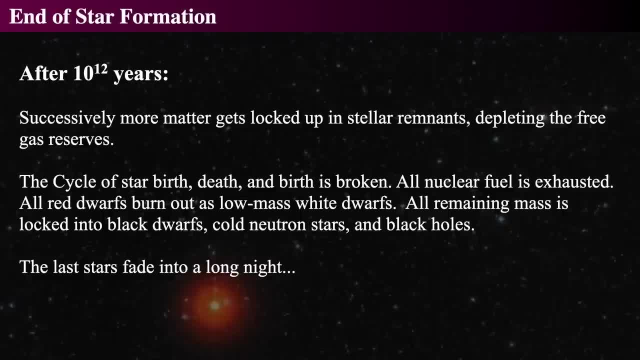 And that will be all done. All star birth will come to an end. There will be no free hydrogen gas anywhere And the last of the red dwarfs, those little tiny M-type dwarf stars, will burn out And become really, really, really low mass white dwarfs. 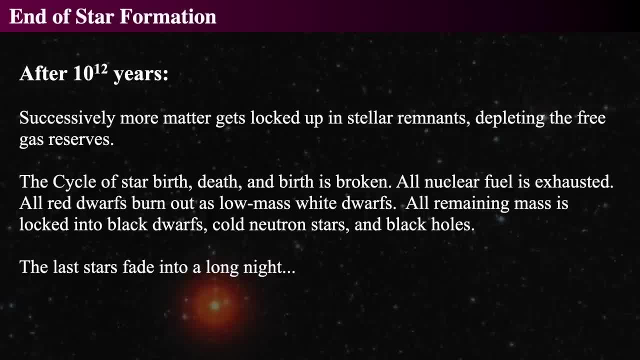 They will become the tiniest, coldest objects And all the rest of things will be in black dwarfs or cold neutron stars and black holes And all the stars will fade into a deep, deep night And that will be the end of the era of starlight. 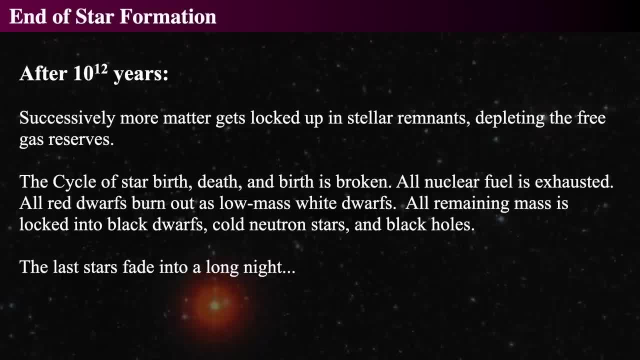 All stars will go out. There will be no light from galaxies that come from starlight, So star formation will be done in a trillion years. Needless to say, that pretty much puts the kibosh on pretty much everything. In fact, we can go about a hundred times farther. 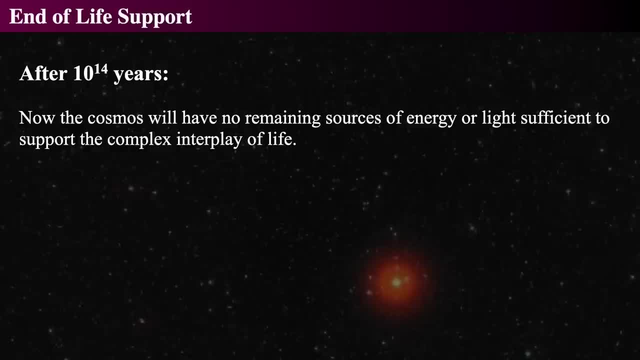 If you wish to kind of think about it, The cosmos won't have any sources of energy in about a hundred trillion years, In ten to the fourteenth years, To support any kind of complex interplay of life. So, no matter what, after the universe has become ten to the fourteenth years old, 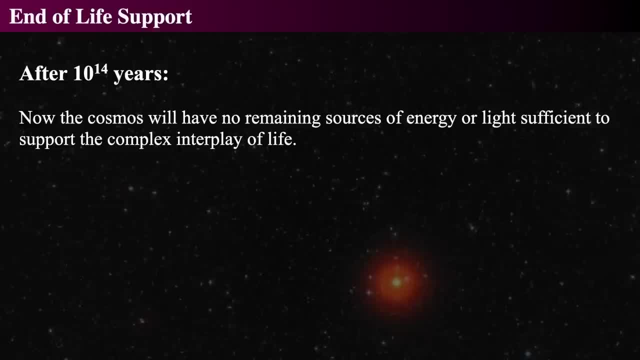 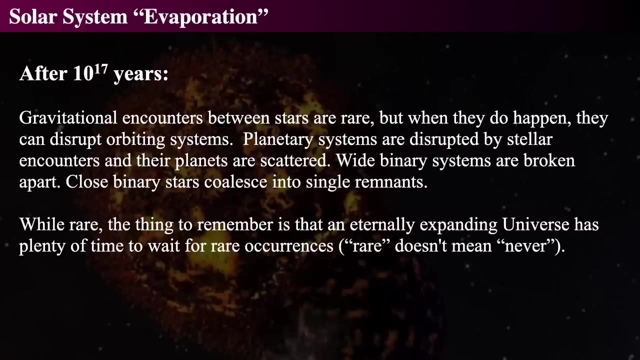 Currently it's ten to the tenth, So ten thousand times the age of the universe. today, There will be no capacity for life to exist anywhere in the universe Because of the loss of energy. After a thousand times more of those times, The solar system would evaporate due to interactions. 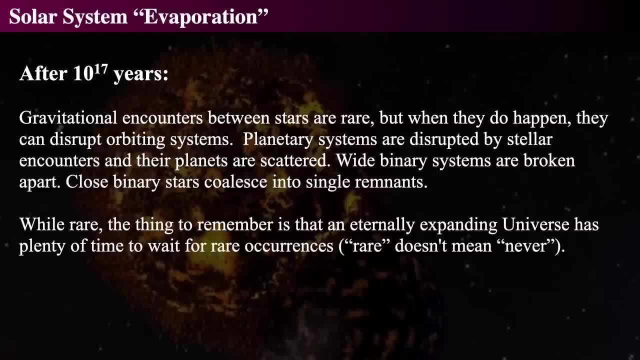 Not evaporate like stars, like the planets themselves would come apart, But simply random interactions between the moon and dust and asteroids, and Jupiter and Saturn and Mercury, Or whatever is left in the solar system And every solar system in the universe, Of which we know there are many through the Kepler Space Telescope. 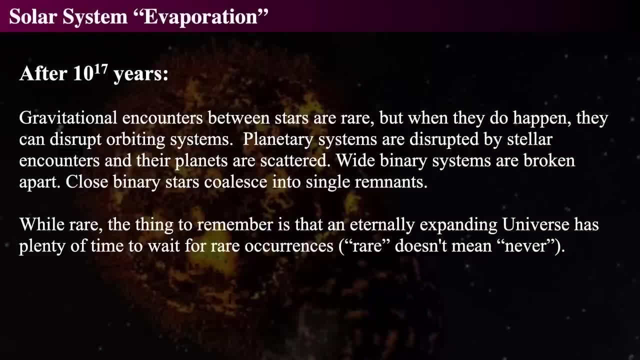 They eventually would be scattered. So planets would be scattered out into the interstellar, into the galactic medium That is now very dark, Or, if they didn't get scattered, They get swallowed up by the white dwarf or neutron star That makes up their whatever they're at. 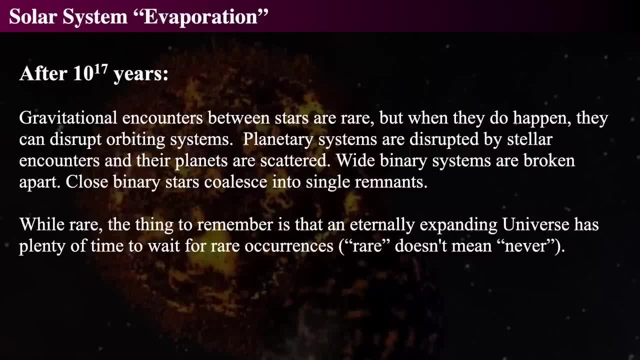 So wide binary systems are broken apart, So everything is now evenly distributed And they're all, or anything that's close gets pulled together, Anything that's far gets flung apart, And so the expanding universe just means that these rare, rare, rare, rare, rare things 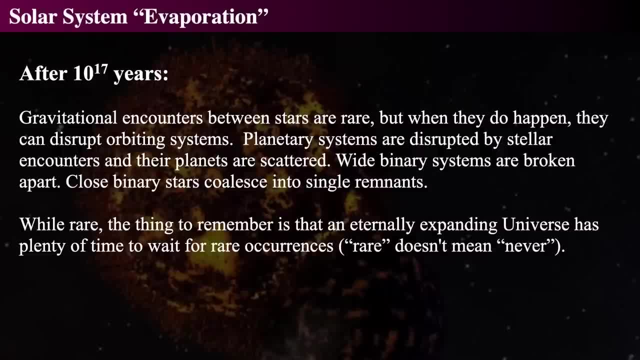 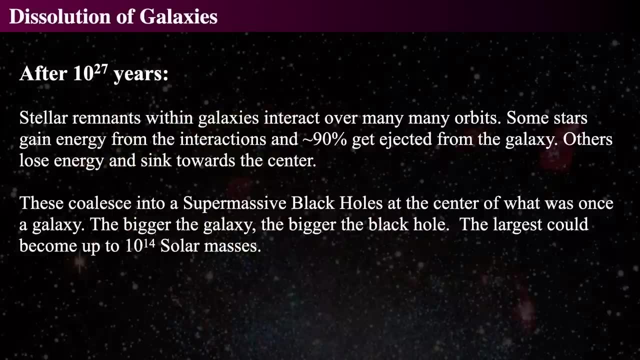 Where a planet might go by another planet, Another planet get flung out. It takes a long time for something like that to happen, But ten to the seventeenth years is a catastrophically long time, Because that's a hundred thousand times more time than the current length of the universe now. 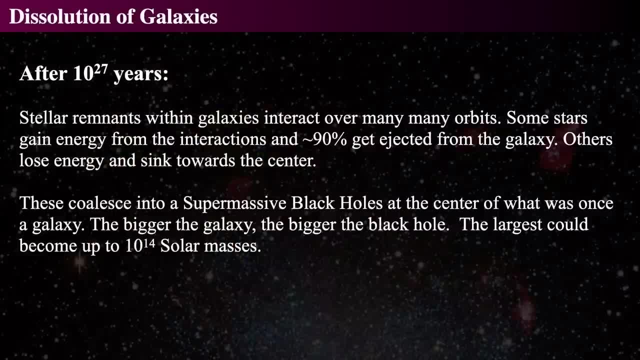 After ten to the twenty-seventh years, Which is a hundred billion times longer than that. So we have to go a hundred billion times more of those In order to get to the point where galaxies themselves- Not just, not just, they get spread apart. 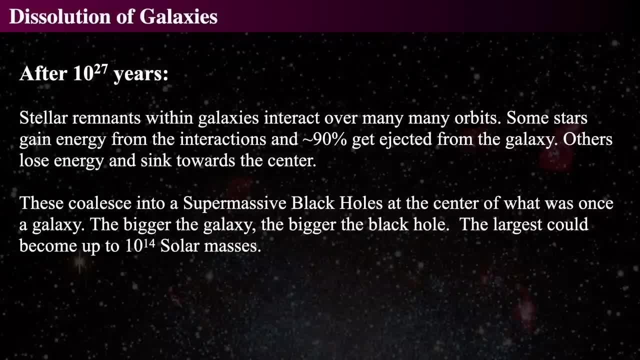 Because of interactions between stellar remnants Such as black holes and dead neutron stars, And almost everything gets ejected And out from them And they just go out And so now there's no such thing as a galaxy anymore And the rest is falling into the supermassive black holes at the center. 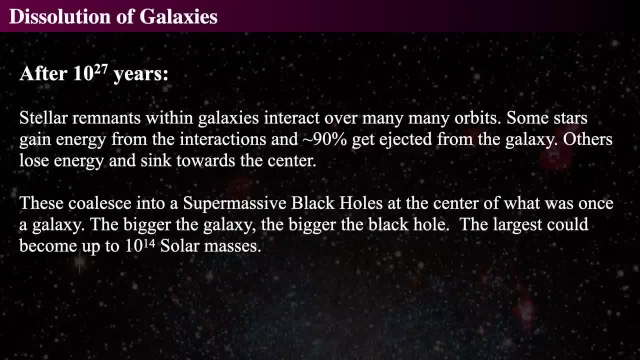 Some of those things. if they coalesce into that supermassive black hole, The largest would become up to a hundred, a hundred trillion solar masses, Which is much larger by a factor of a thousand Than any of the other any current supermassive black hole known. 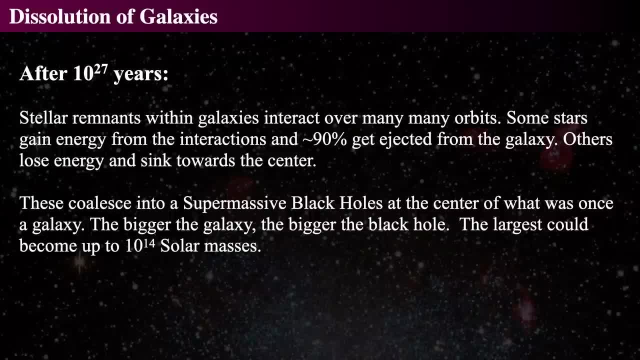 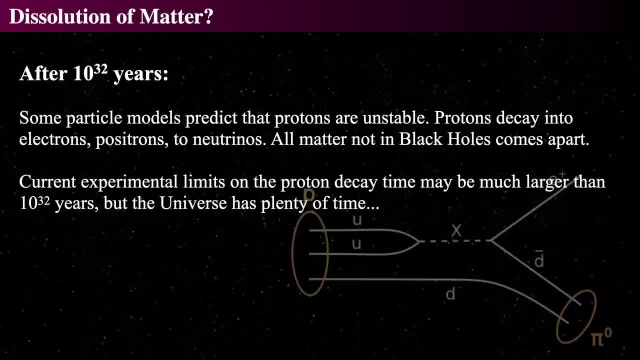 So galaxies would eventually spread out And not be recognizable in ten to the twenty-seventh years, Even farther in the future than that, After ten to the thirty-second years, Which is now, wow, really far: Ten to the twenty, ten to the twenty-second times, the current age of the cosmos. 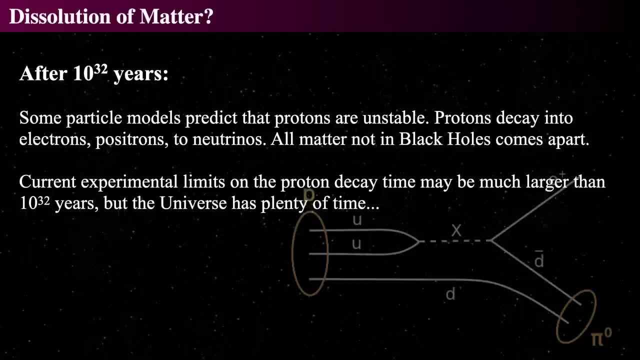 It is thought that protons Themselves would be unstable, And if they are unstable, They would decay into electrons and positrons and neutrinos And maybe even pions or something like that, Which means that protons would disappear And matter would simply fall apart. 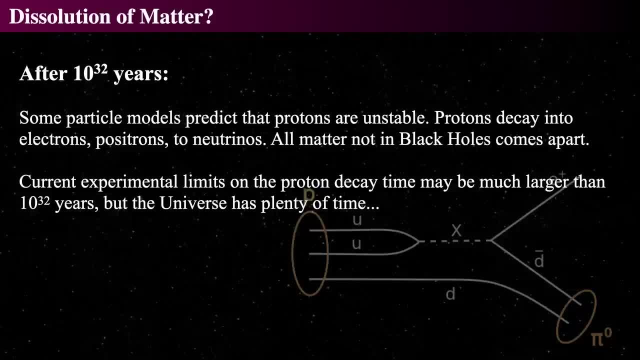 And if matter falls apart, If it's not in a black hole, Anything that's matter stops being what we call matter And basically becomes positrons, electrons and neutrinos, And that's all we're left with. So that's going to be long. 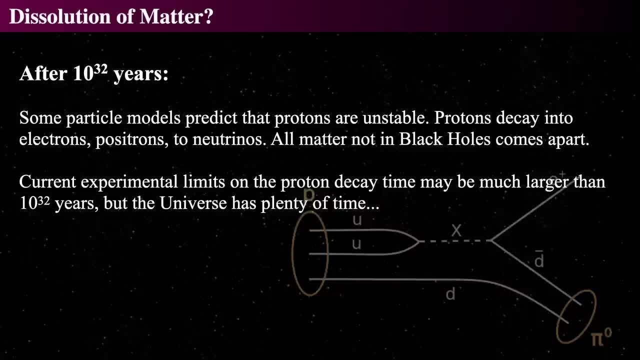 Nobody really has ever seen this decay, But it's possible that it's going to happen Because you know the strong nuclear force allows for things to happen, But the probability is extraordinarily rare After an extraordinarily long period of time- Ten to the sixty-seventh years. 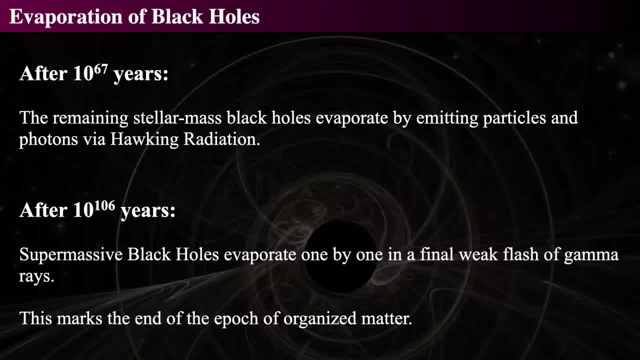 Stellar mass black holes evaporate by emitting Hawking radiation And after ten to the hundred and sixth years, Supermassive black holes evaporate by Hawking radiation. This is enormous, enormous, enormous. ending, And that is the end of all organized matter in any way. 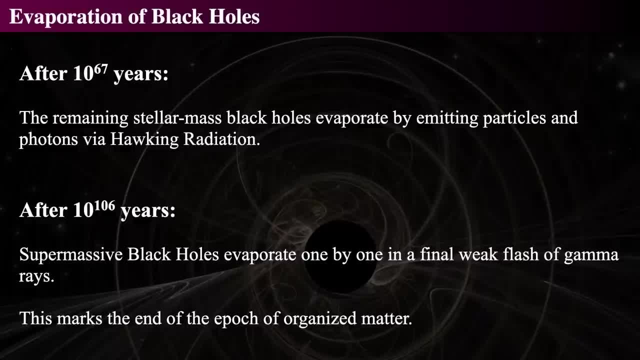 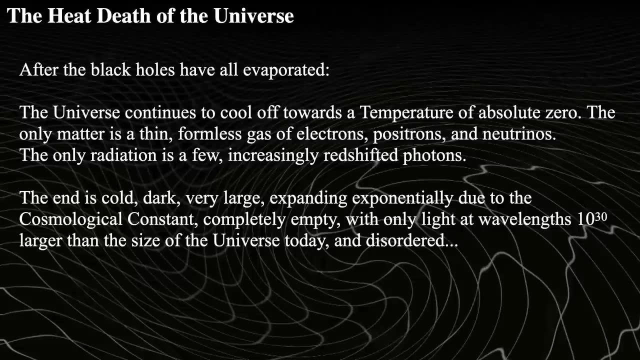 All that's left in the cosmos now is an accelerating, rapidly accelerating cosmos Filled, or only gently filled, with extremely long wavelengths of light And neutrinos, and electrons and positrons. So after they're all evaporated, The universe is basically cooled off to a temperature of absolute zero. 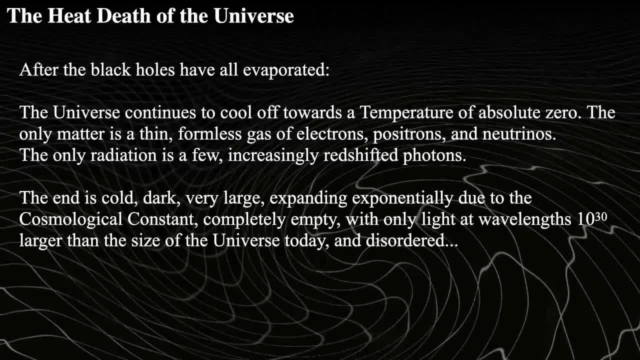 The only thing that's left is a formless thin gas Of electrons, positrons and neutrinos, And they're spaced apart by hundreds of megaparsecs, So they're not really touching the radiation. The light is incredibly redshifted photons. 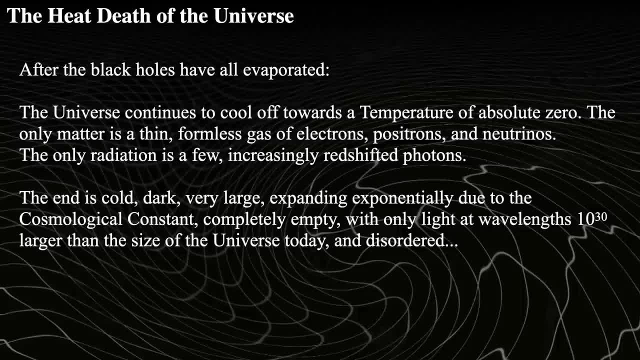 And in fact probably the photons themselves would be much larger than the size scale of the universe today, So they would basically not even feel like photons to us. They would be very, very old And the exponential expansion would make it very, very, very cold. 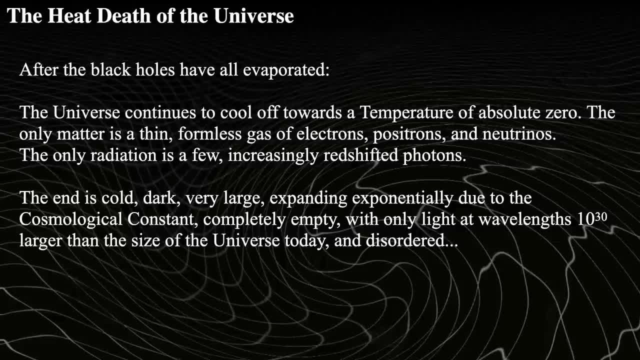 Very, very empty, With nothing in it. So a size scale universe, So a size scale of something like our current universe, might contain one electron And might contain one neutrino And one photon. That's what's to happen in about 10 to the 160 years. 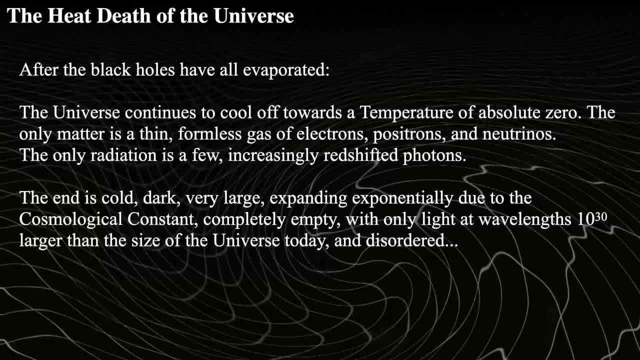 And probably that's a very large number of one of each at that time. Probably none, Probably nothing. It will all expand away. So that's kind of the heat death of the universe. There won't be nothing left. There won't be anything left. 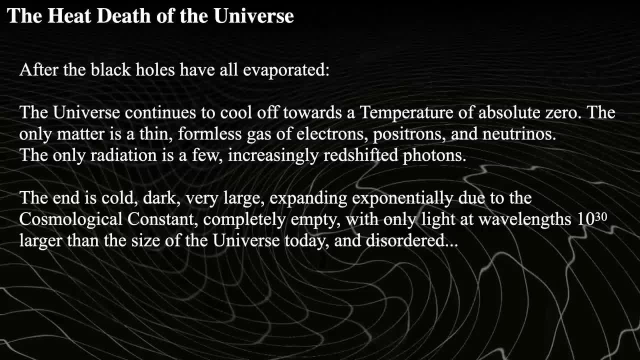 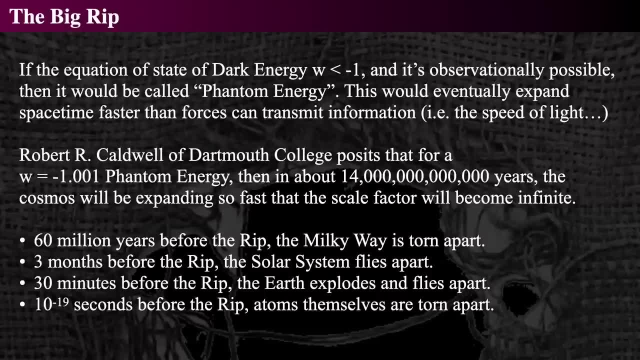 It will just be cool, cold and empty And continuing to expand, And space will be bigger and bigger and bigger. However, if the equation of state of dark energy is less than minus one, Then it's still observationally possible, But it's not quite probable because of the most recent stuff that's come out by the Planck team. 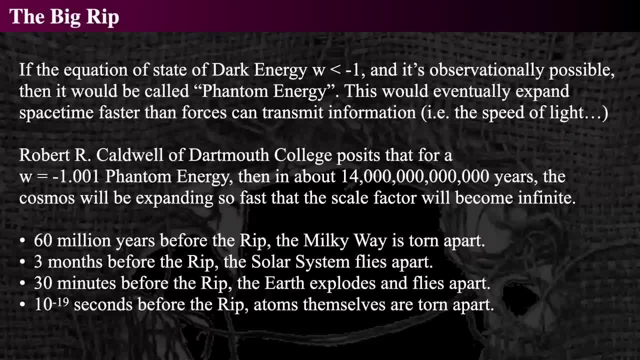 Then they would have a phantom energy And it would eventually rip the universe apart in about 14 trillion years, Where the expansion of the universe would be so fast that it would overcome the ability of the electrostatic force, The weak nuclear force And the strong nuclear force. 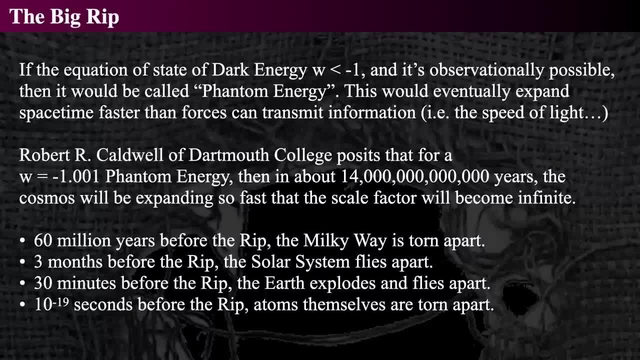 To respond to the expansion of space time And right before this, if the phantom energy was just minus .001.. If W was just a little bit less than one, The universe is done in 14 trillion years, Like really done, Or more like 20 or so trillion years. So it's going to take a while, But it will happen. It will rip itself apart 60 million years before that. The Milky Way is torn apart by the expansion of the universe Three months. The solar system flies apart 30 minutes before it. 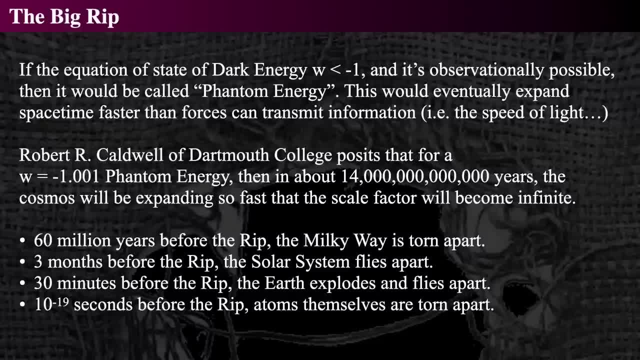 The earth explodes because of the expansion of the universe And 10 to the minus 19 seconds before the rip, Atoms themselves are torn apart And it becomes kind of an inverse singularity, Like we have with the Big Bang, But it's just the universe expanding. 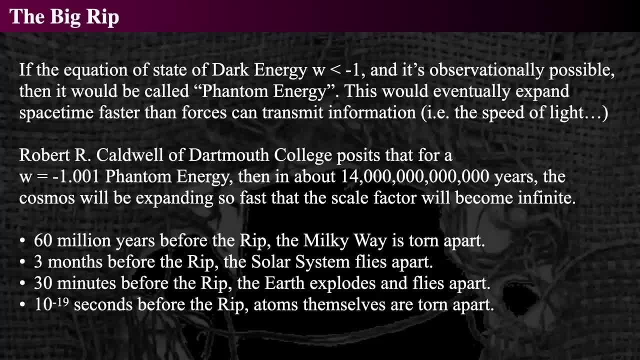 Expanding. with nothing in it. That's a big rip. However, the Planck probe shows that we're in a flat, accelerating cosmos And not one with phantom energy, So this is very interesting to talk about, But it's probably not what it is. 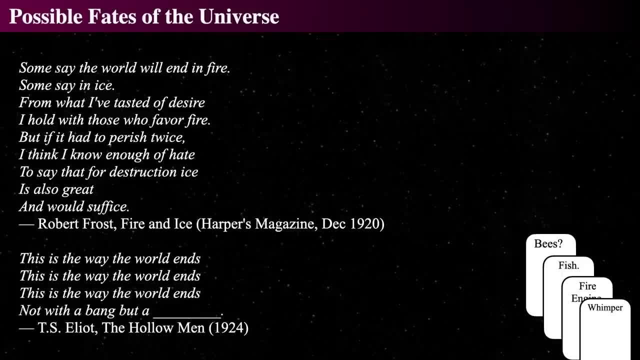 So the possible fates of the universe. Some say the world will end in fire, Some will say in ice. But from what I've tasted of desire, I hold with those who favor fire. But if I had to perish twice and think I know enough of hate to say that destruction ice is also great and would suffice. 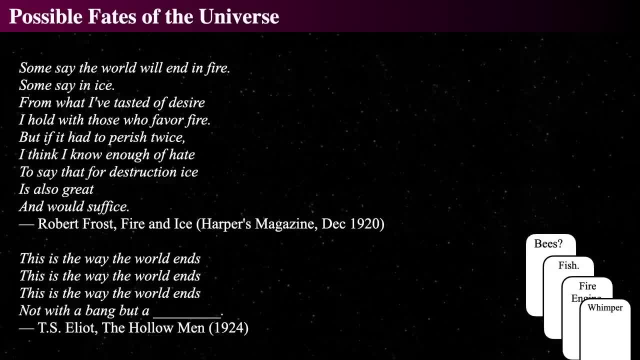 And will the world end with a bang Or a whimper is the real question. We don't know, But it seems like the world will end in ice, essentially Not even in ice. Ice won't even be there. It'll be emptiness and cold. 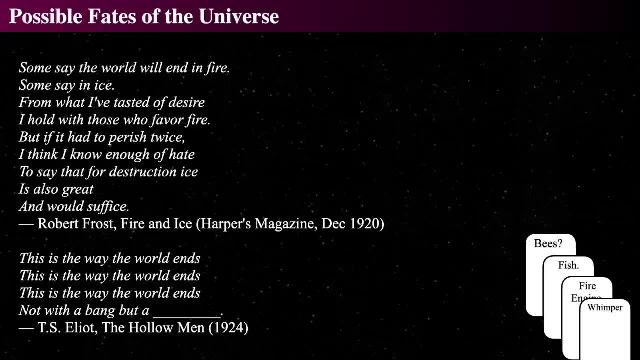 And so the end is a whimper, A tiny, tiny nothingness. How's that for you for an afternoon? Now, if we look then to the largest size scales and say outside of our cosmos, it's called beyond the particle horizon, Meaning beyond everything in the universe, what we can possibly know. 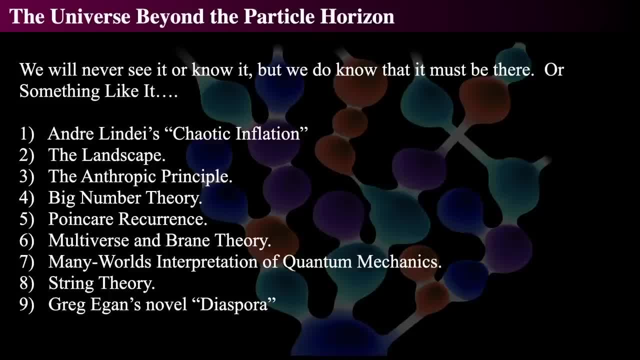 What we can possibly measure. Not know, but measure. There are lots of different things that we can talk about, that we could go over in extended things, So I leave this as a list. I leave this as a list to you to go over and go hunt down. 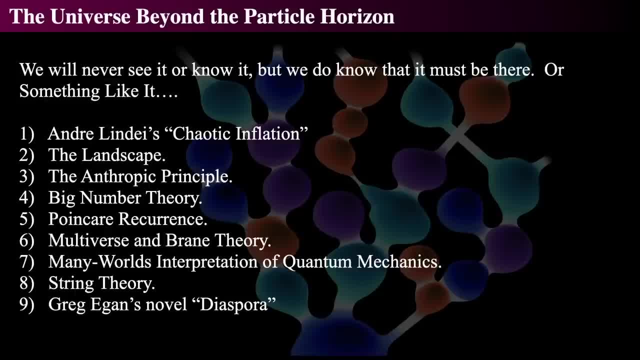 Because this is really some interesting stuff for you to go investigate and learn about, Because to me, this has always been some of the most interesting things, Like the chaotic inflation, Meaning maybe the inflation happened here, Or maybe it happened there And it'll happen here. 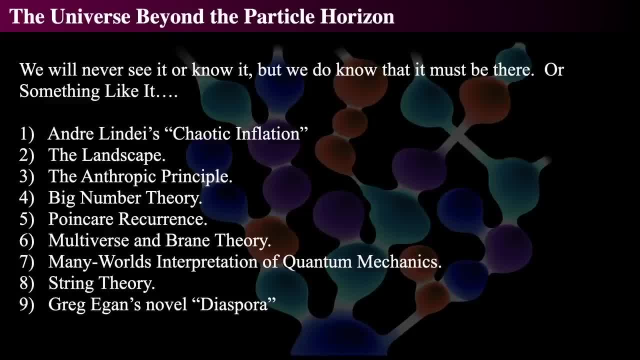 And maybe it'll happen again. So chaotic inflation has a very interesting concept, The concept of the land escape, Meaning that there are many, many, many, many universes, And the universe is much, much larger than our observable horizon, And there's a vast area where universes pinch off and expand from each other. 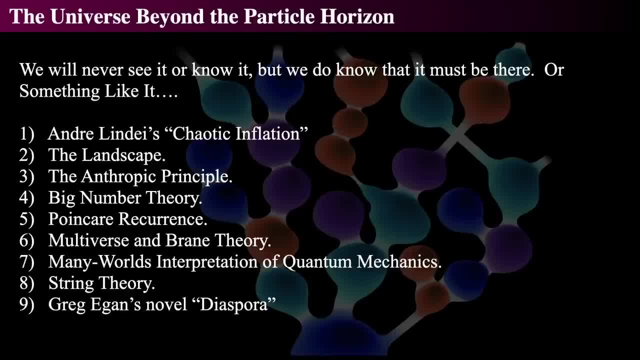 But maybe they have different physical constants, Maybe the constant of the speed of light is different, Or the charge of an electron is different, But then that leads to the concept of the anthropic principle, Which is: hmm, our universe is funny. 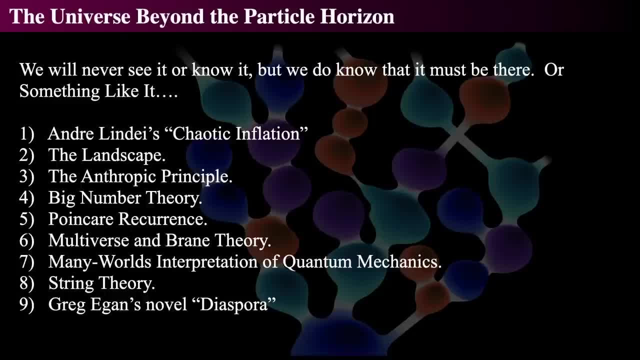 It has life in it And all. if you change any one of those constants by a little bit, we ain't got nothing. Big number theory has some very strange things that say there must be some relationship between the big, big, big numbers. 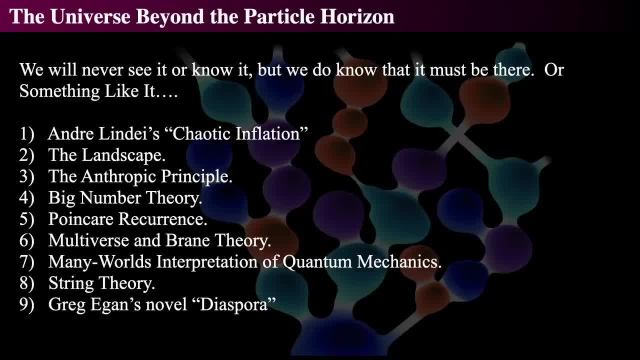 Because they all tend to be big and all the same rough value. The Poincaré recurrence says: well, if you let the universe age long enough, you eventually get the same stuff again. But that seems to be eliminated by the fact that dark energy is going to push everything apart. 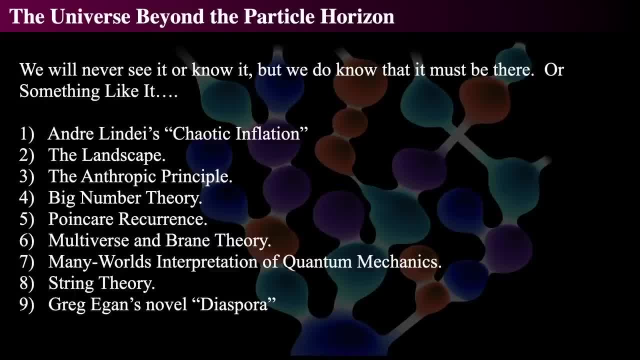 Multiverse concepts and brain theories posit that there are additional spatial dimensions that we do not perceive. That, then, are literally right next to us, But since we don't perceive them, the only thing that leaks across is maybe gravity, And that would be what we call a brain. 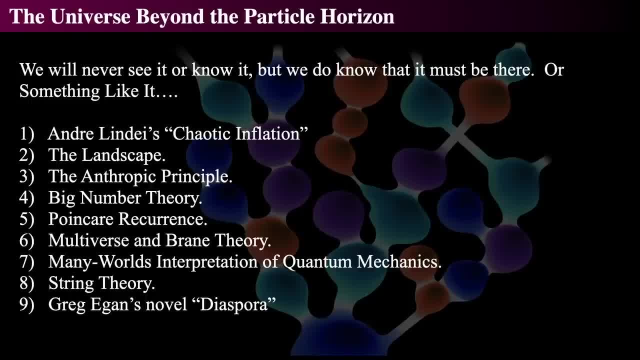 So as in membranes, So there'd be multiverses with the distance between them is millimeters, But in every direction. But we can't get there. But maybe gravity reaches through And that leads us to the concepts of string theory And also the concept of many worlds. interpretation of quantum mechanics. 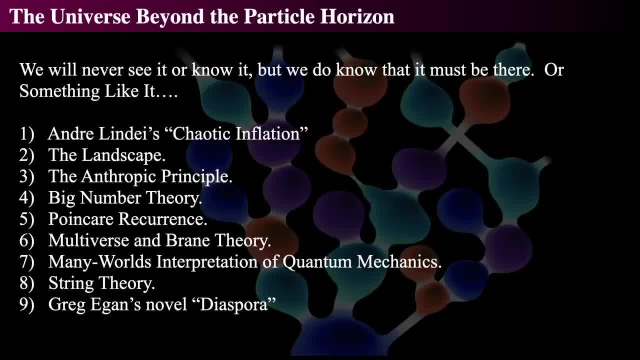 which says that every action you do creates a new universe, And that's an actual interpretation of quantum mechanics because of the nature of choice. String theory supports the concept of brain theory, which says that the fundamental things aren't atoms, but these tiny things that are strings, that are 11 dimensional objects. 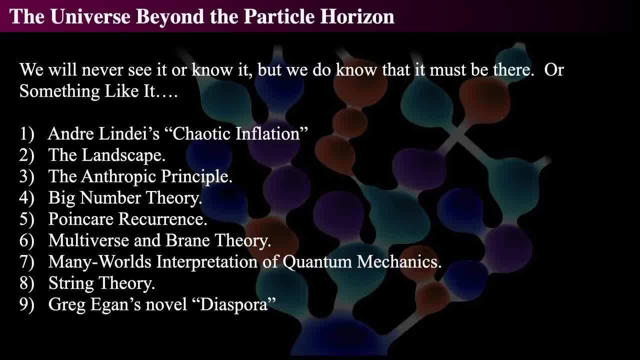 that you can only perceive their 11th dimensions if you're down on the size scale of 10 to the minus 43rd meters or so. For fun and enjoyment, I invite you to go look at author Greg Egan's science fiction novel Diaspora. 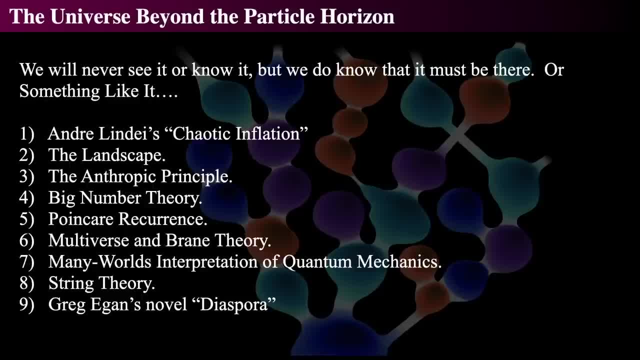 which looks at all of this, Looks at all of these things that we just talked about in a very, really, really heady way. It's one of the most hard sci-fi novels, But I encourage you to go take a look at it.